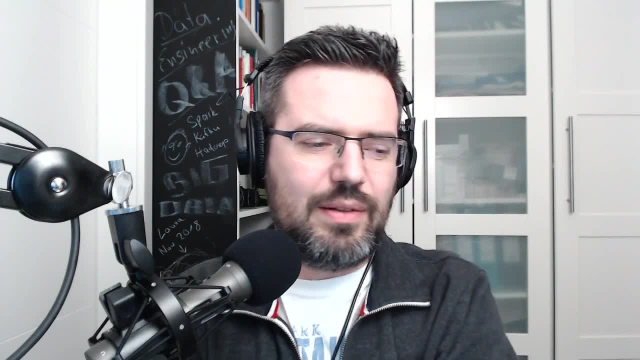 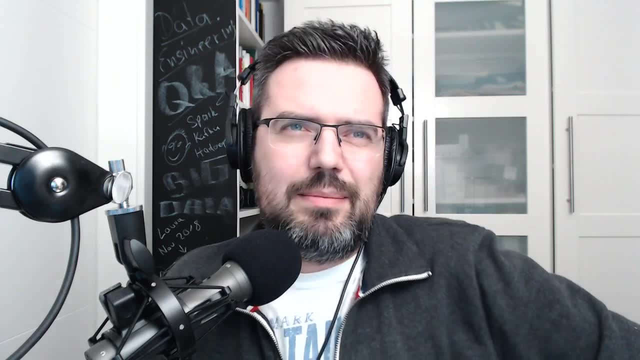 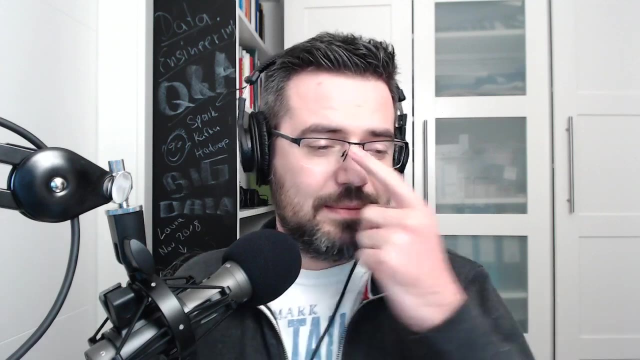 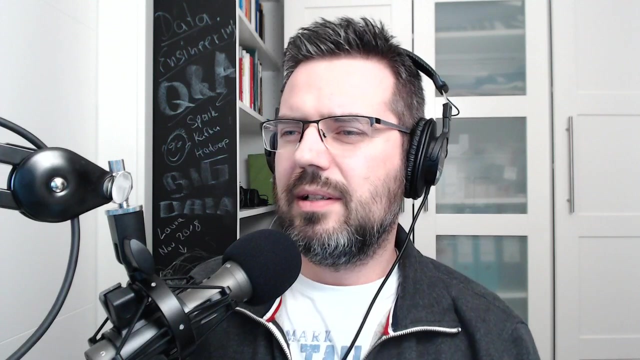 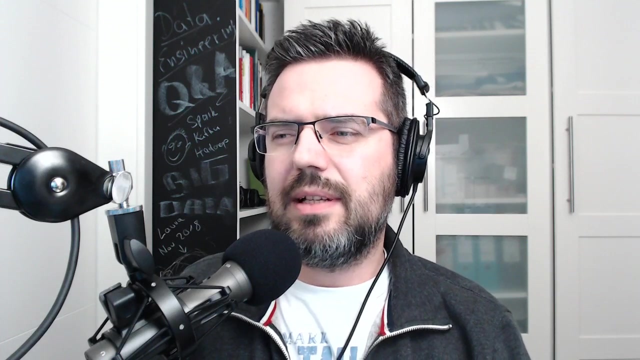 a lot of confusion about when to use NoSQL databases, and people are many times using them although they should not use them. And so, yeah, NoSQL databases. I would say let's start first looking into SQL. make a quick SQL excursion on how stuff. 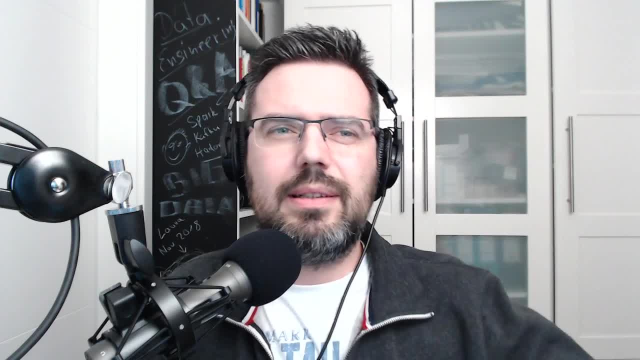 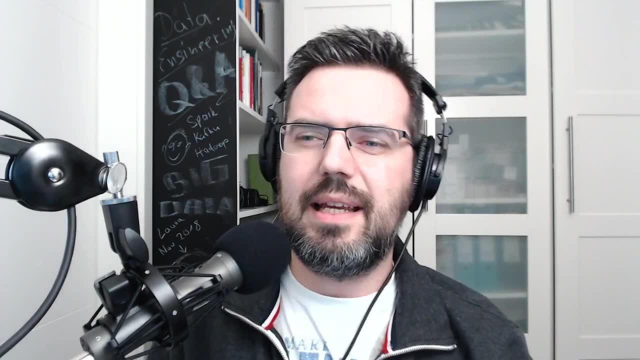 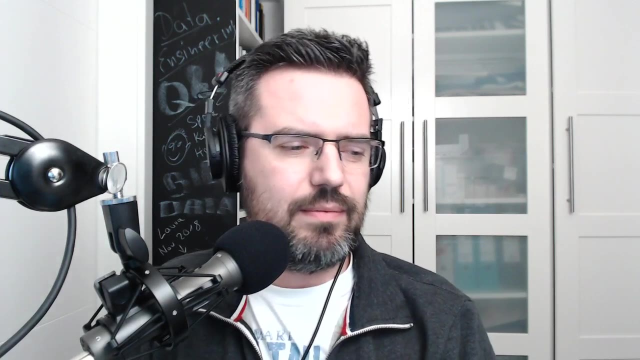 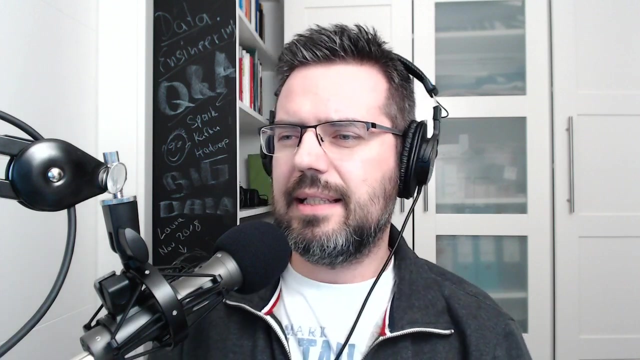 looks in a SQL database and then we are going into a NoSQL database that I'm very familiar with and that is called HBase. HBase is a NoSQL database based on Hadoop or based on the Hadoop ecosystem. It's delivered basically with Hadoop and it's super interesting and it's a column store. 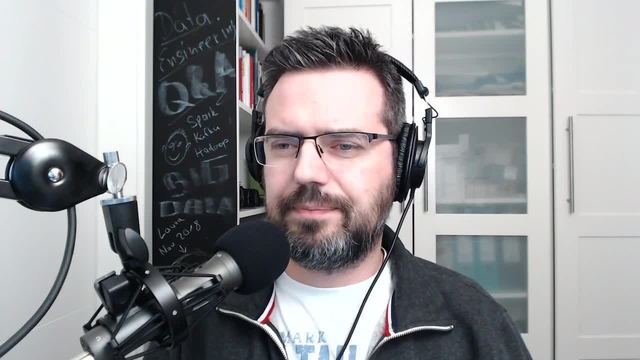 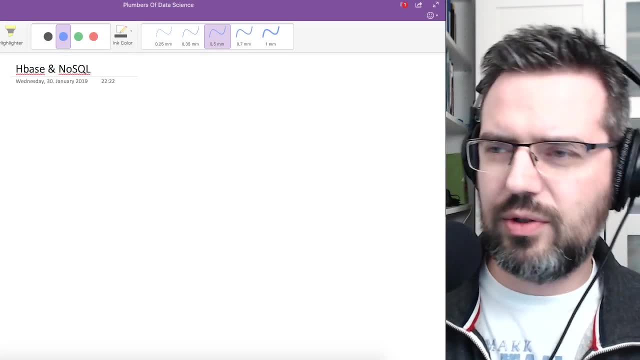 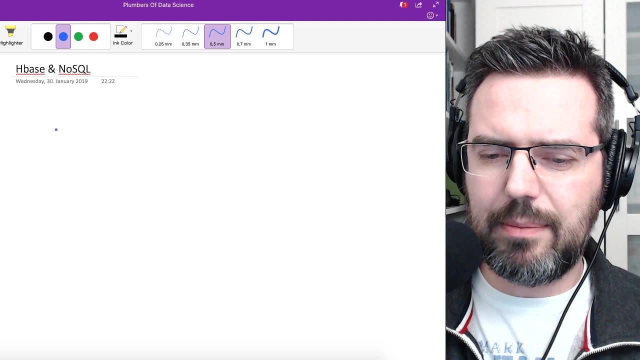 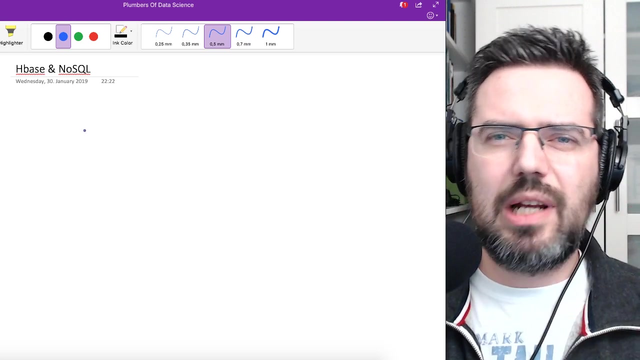 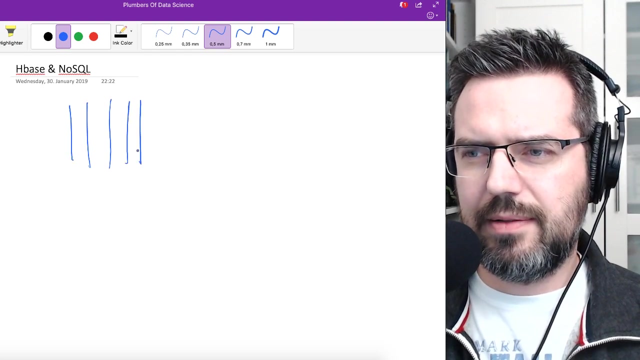 So, okay, let's first look at how a SQL database actually looks. If you have a SQL database, the thing is with SQL databases: You have a row and a column store. It's much like an Excel sheet. You have your columns. 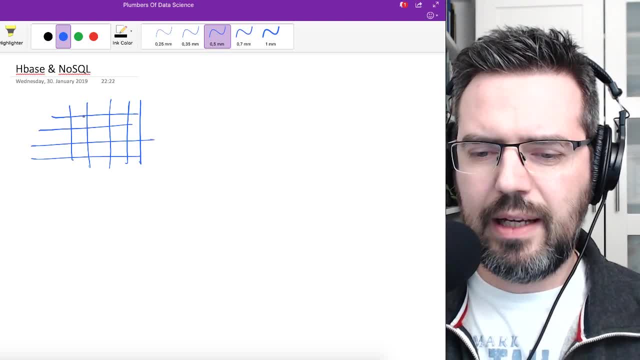 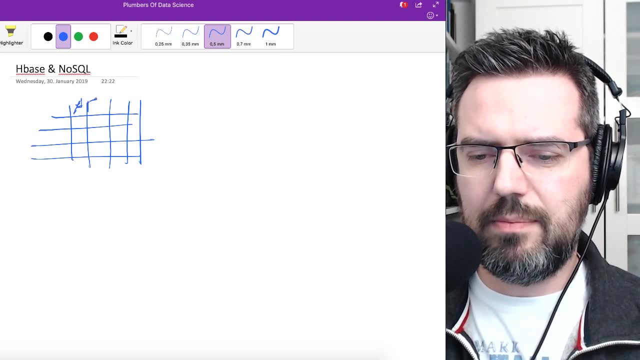 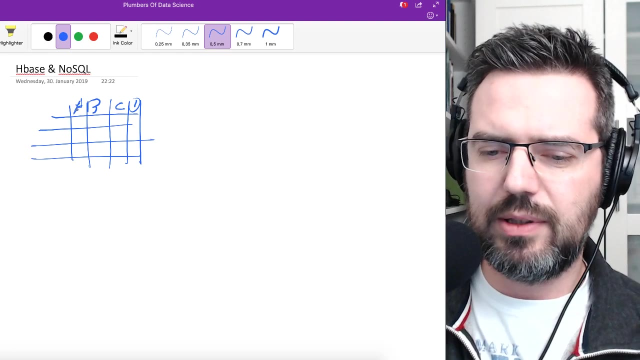 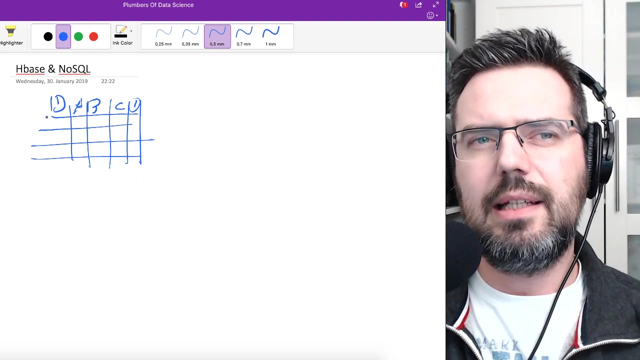 and then you have your rows and each column. you're giving them a name. Let's say, this is A, this is B, C and D. What you're also giving them is an ID. This is usually done. ID is automatically incrementing. 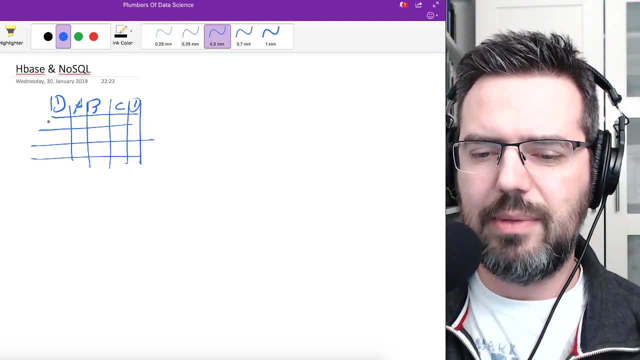 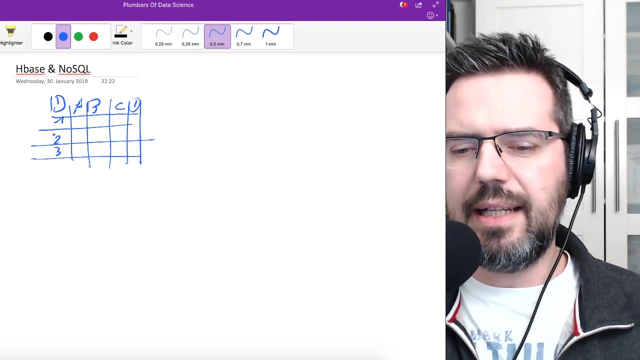 so with every step, with every row you're setting in, you're incrementing the ID. So it's basically one, two, three, So every row gets an ID, And the idea behind a SQL database and behind a SQL database is that you have multiple of. 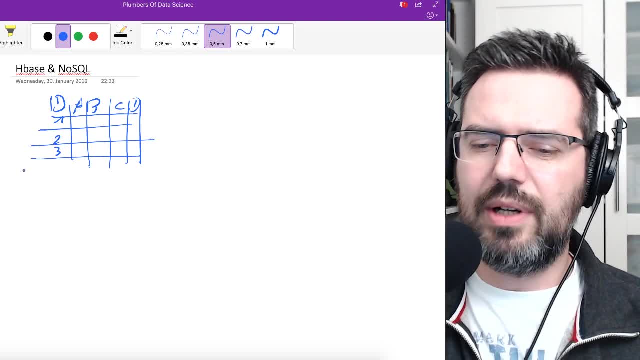 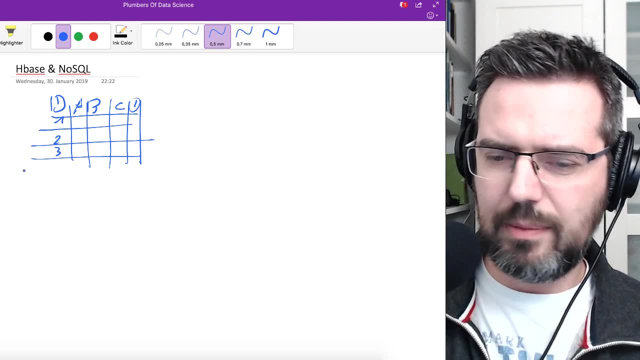 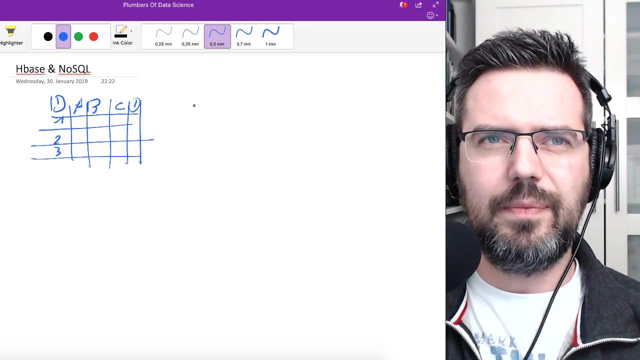 those tables And you define them beforehand, before you're setting or before you're uploading the data, putting in the data, and then, basically, you have multiple of those. So what you could have, you could, for instance, yeah, what you can have then is, for instance, 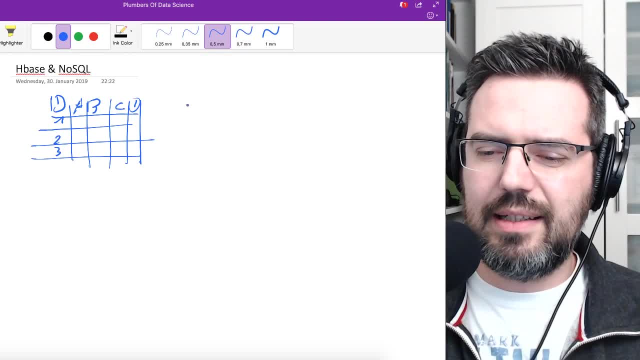 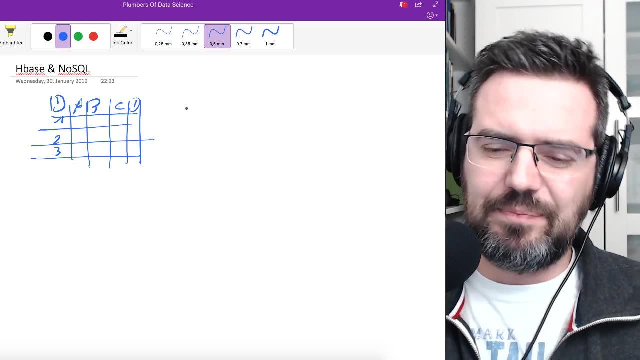 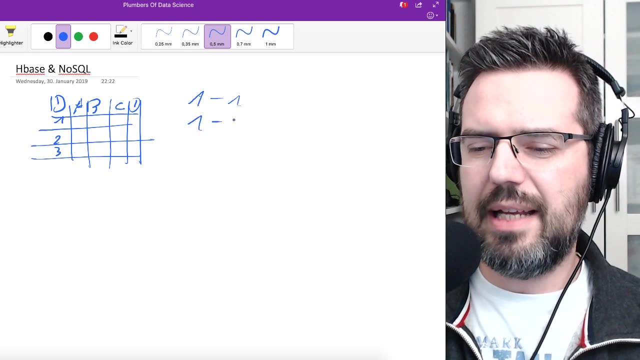 you have multiple relations between the tables And it's basically a SQL database, is super easy to set up And to architect. Yeah, it's not really hard You can have. for instance, you can have a one-to-one relationships or one-to-n relationships. 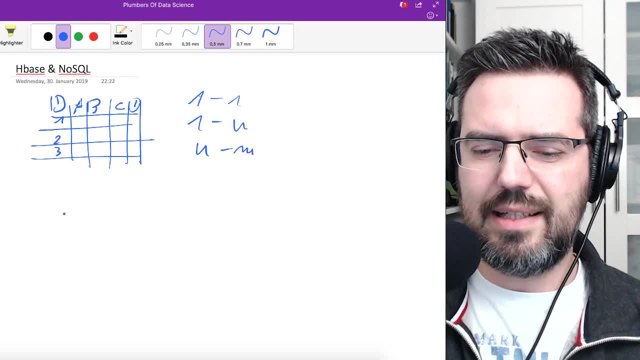 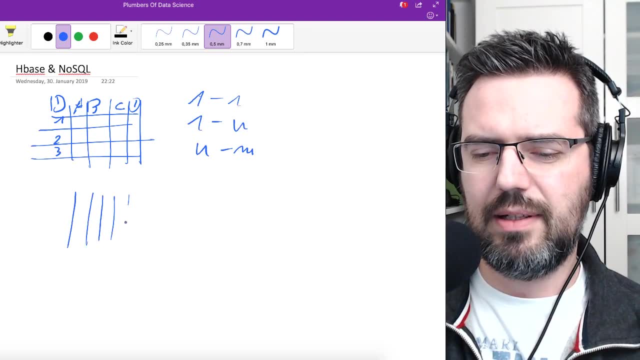 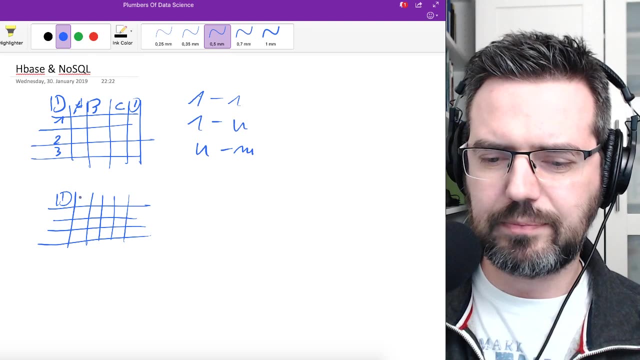 or n-to-m relationships And for a, let's say you have a one-to-n, then you have another. let's say you have another table, And how this works is this table also has an ID And some names of these tables. 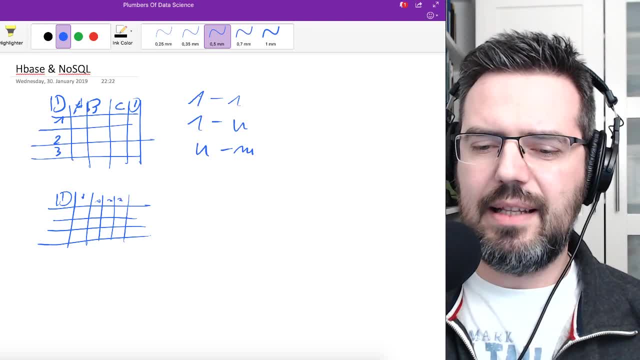 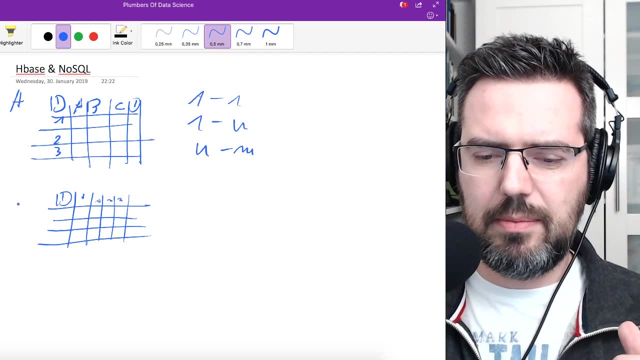 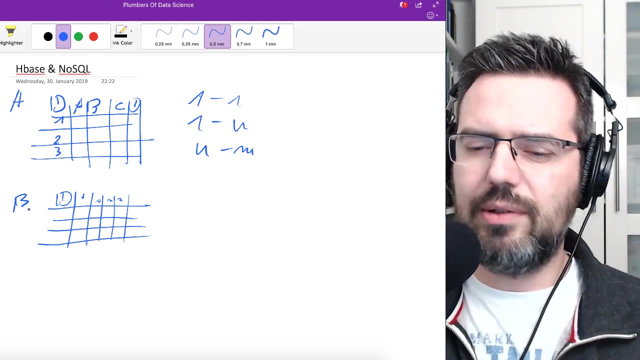 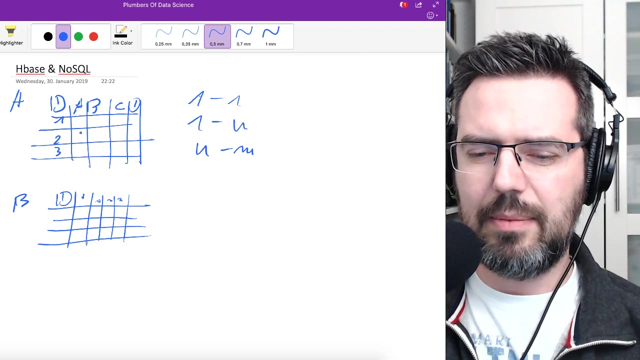 Of the columns And this is. then you have a, what is called a. let's call this table A And let's call this table B. What you have is a primary key and foreign key relationship. So you can have, for instance, this ID from row A, from table A. you can have this as: 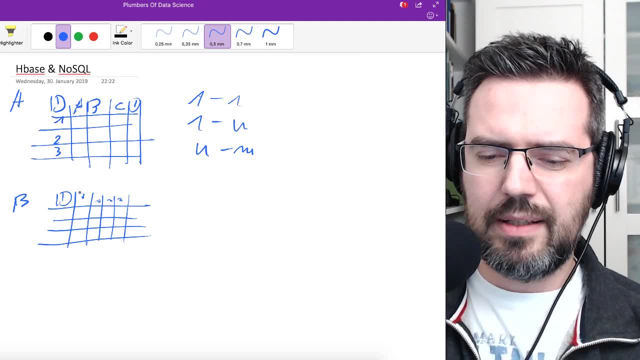 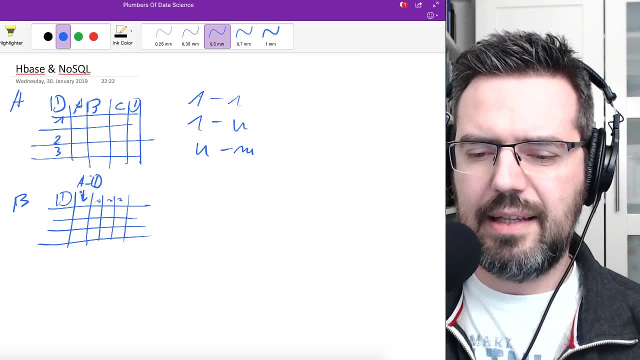 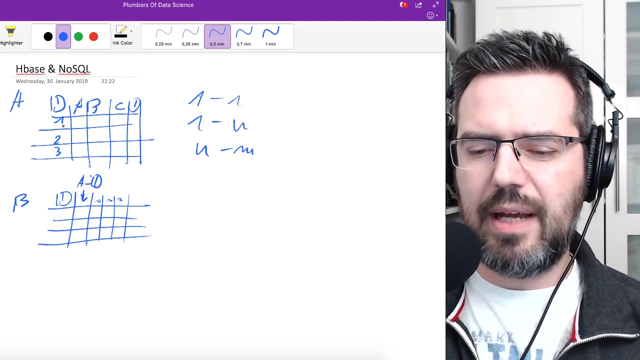 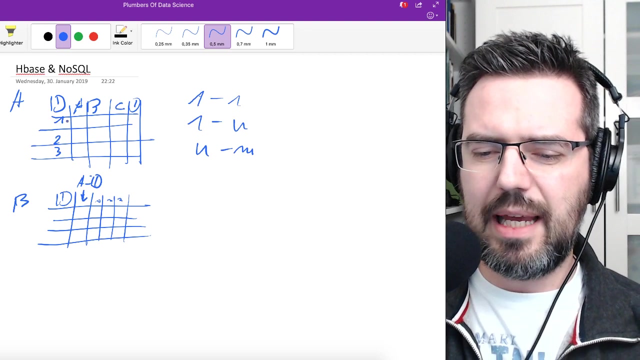 a column in table B. So then you would have here a ID, Um ID, in one of those columns And this is then a foreign key of the table A, And this way you could have a one one-to-n relationship. So one row of those, one row with one ID of table A can be then here multiple times in. 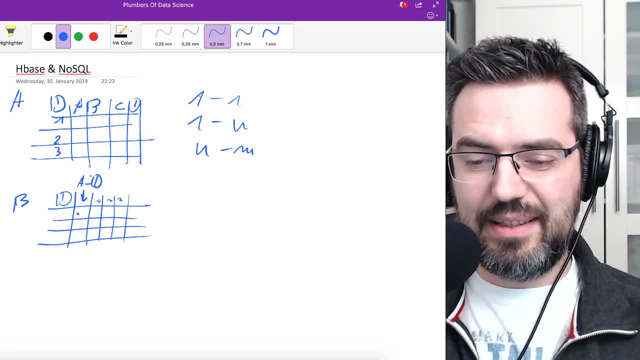 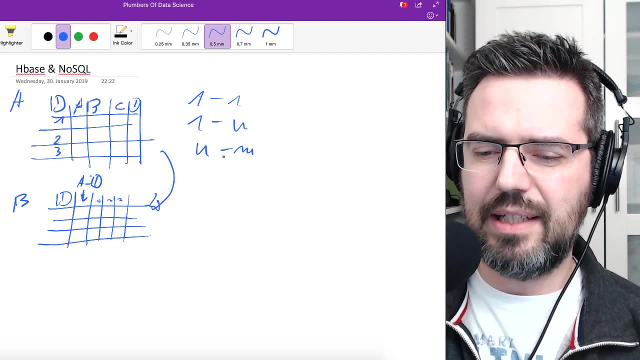 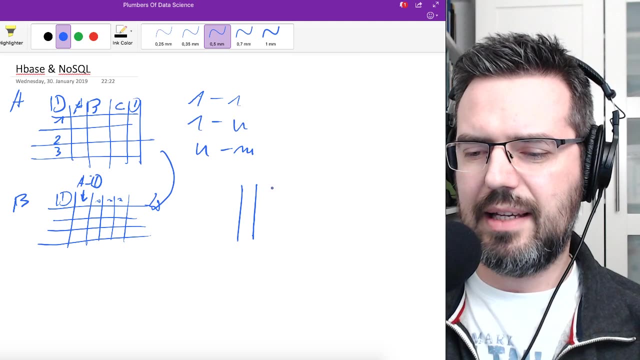 row A in table B And in one of those rows, then you have basically linked those together here. But you could also have N to M relationships. then you have both IDs, IDA and IDB, and you have another, let's say, a helper table. 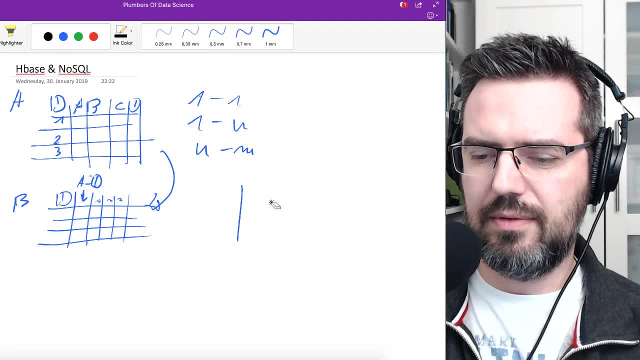 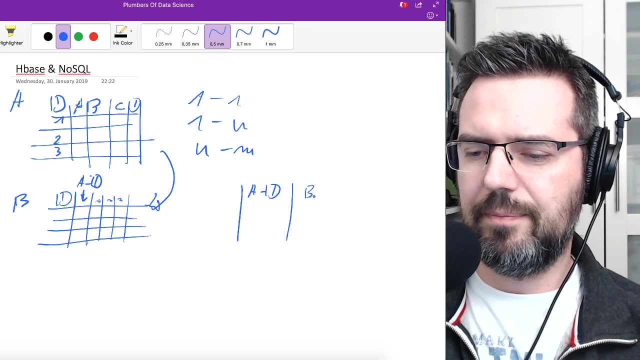 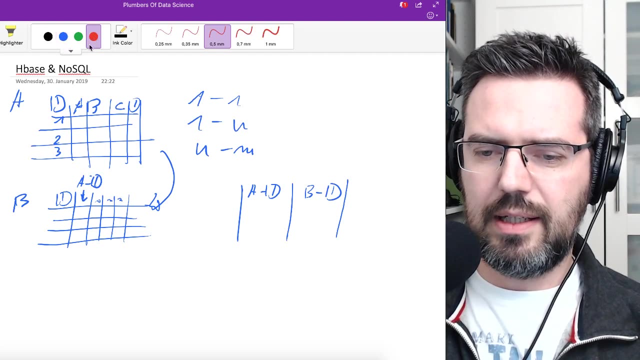 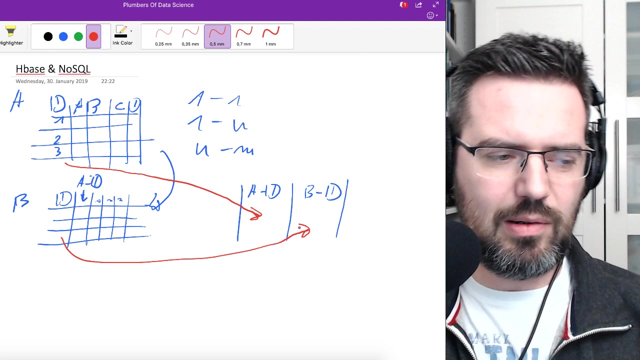 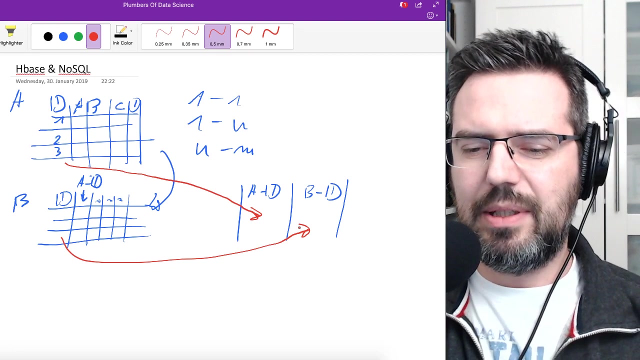 and this table has in the columns. let me do this differently here. you have in the columns, you have A ID and you have another column, B ID, and then those IDs are getting then filled into this helper column and so you can basically have a link between these. 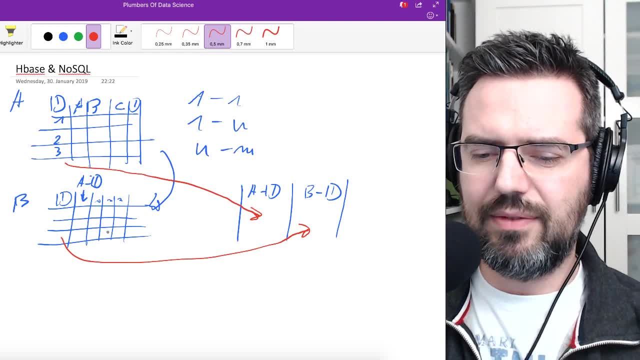 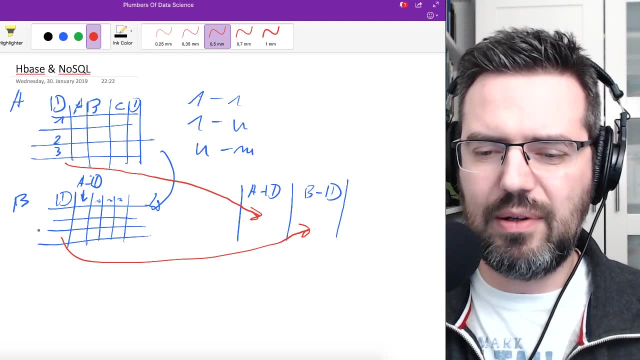 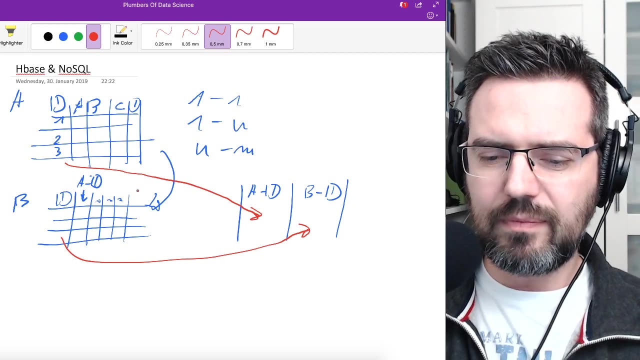 and with select statements you can then select the different. you can then select the rows that you are you want to query from the database. So it's a very, very simple thing and you can have the relations here this way. 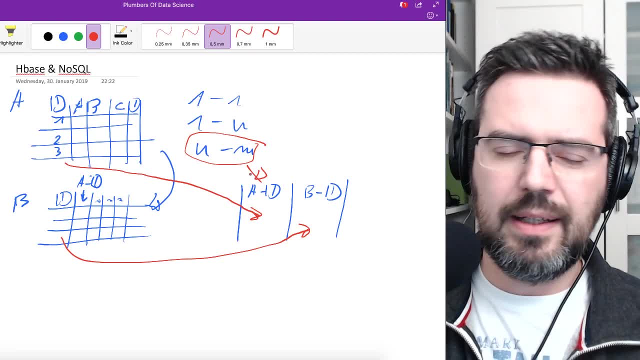 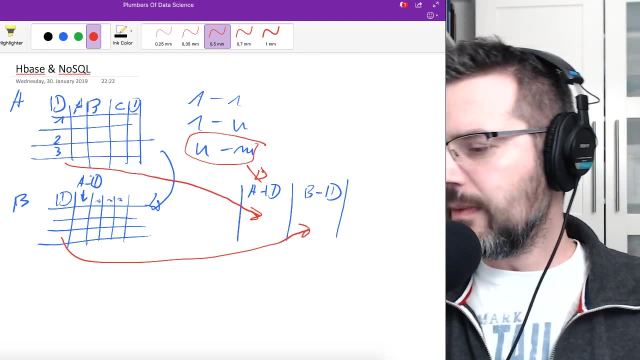 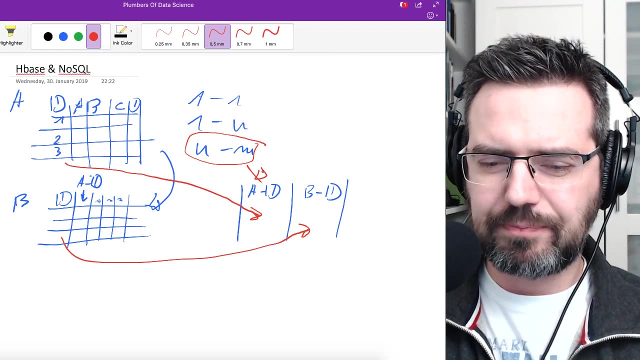 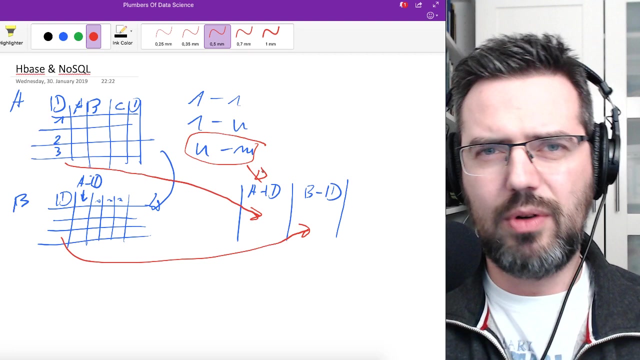 So this would be here. this is here N to M. So the thing here with this is: how does that? how does that work? How does basically the SQL database find the table or the rows within the tables, if you are searching for them? 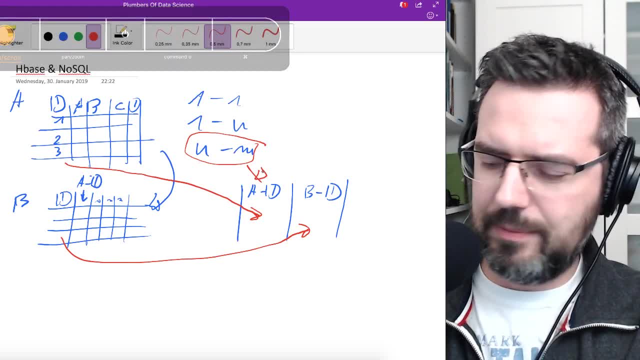 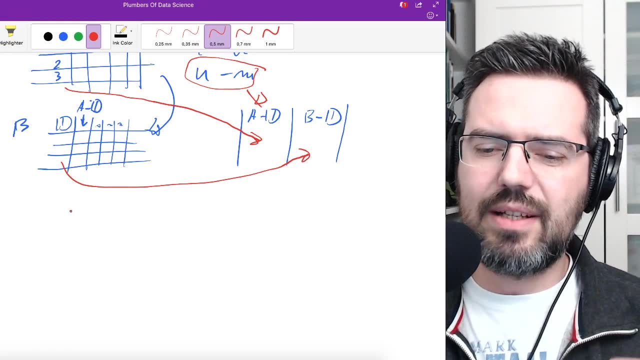 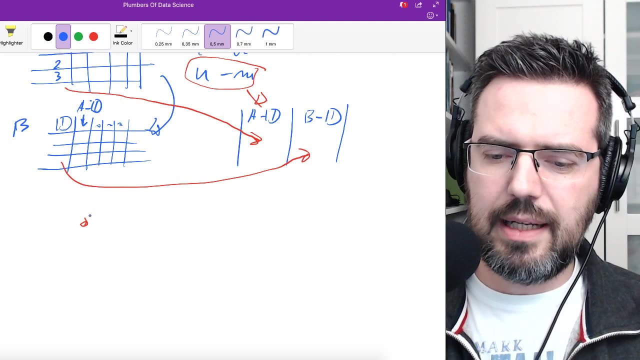 And the idea here with this, how this works, is usually it creates an index of each table and this index is working basically like a. let me do it okay. blue is working basically like a binary tree. So you have a tree. 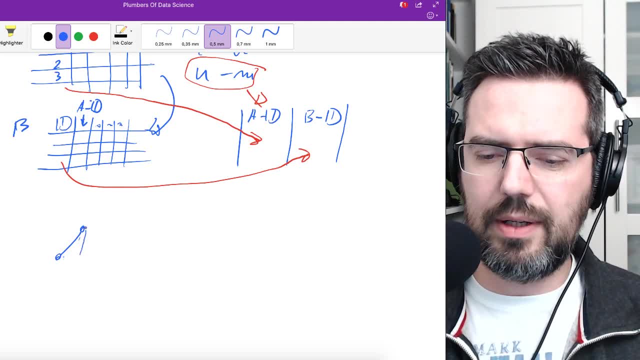 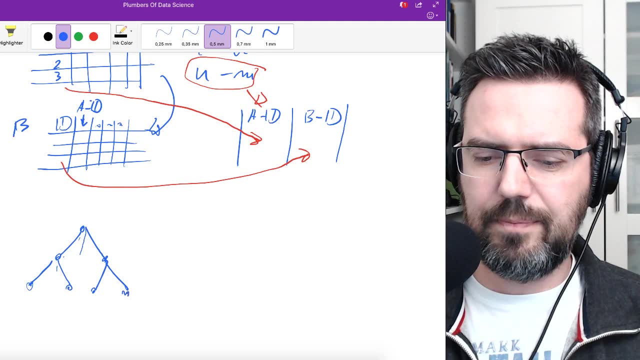 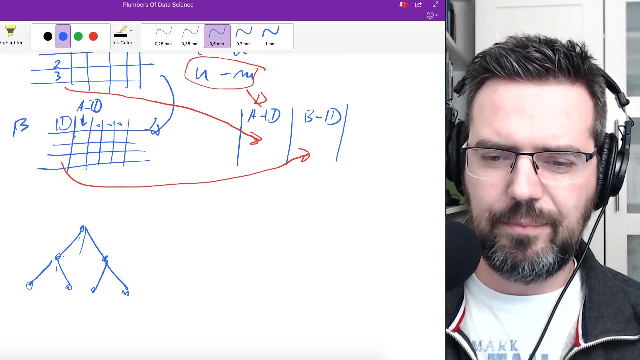 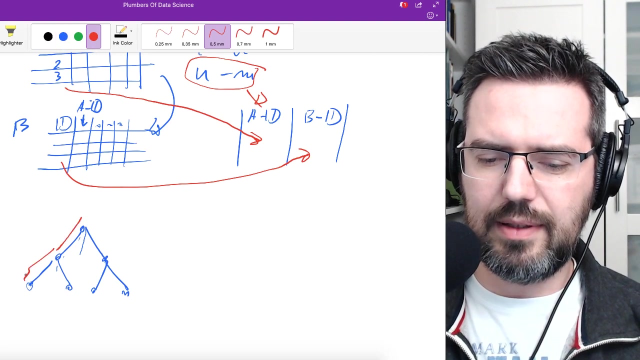 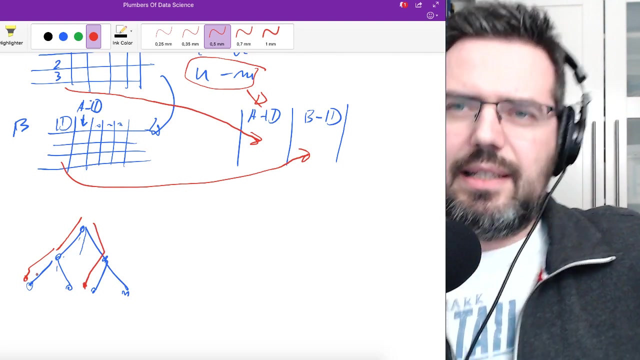 and then it's going. it's going always down here and always the binary decision. So when you're doing a select, the whole thing basically walks down and finds the, the columns that you want to query. And now here's where the problem is coming in. 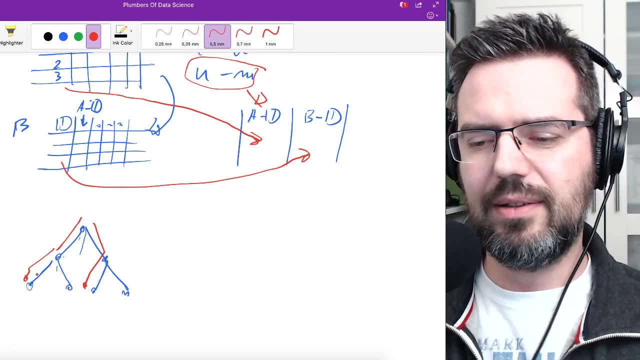 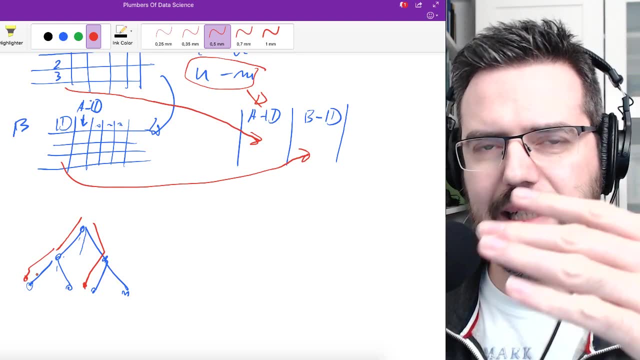 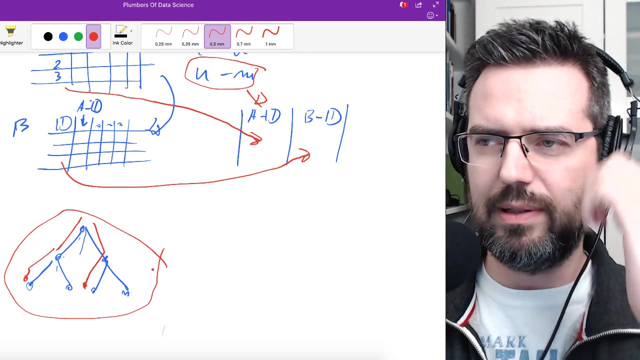 If you have a SQL database and you have defined all this and now you're going to fill it with a lot of data, What is happening when you're filling it with a lot of data? Well, this tree here, this thing, is getting super huge. 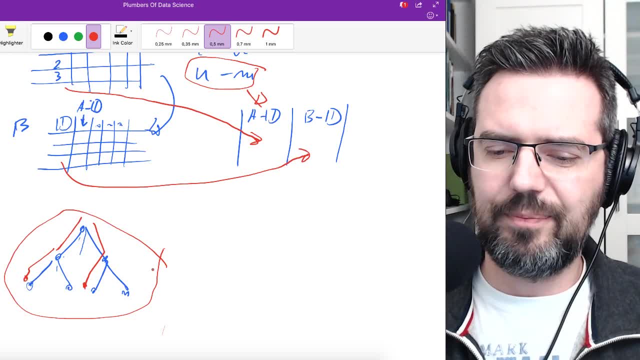 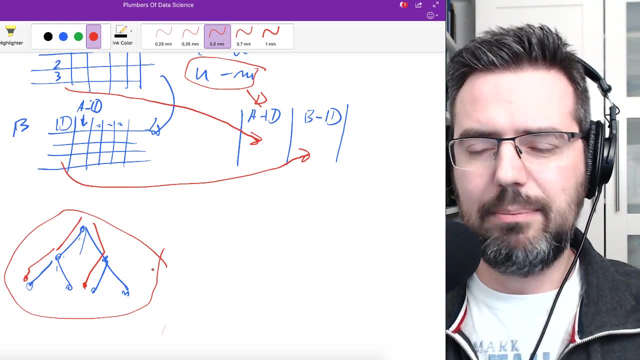 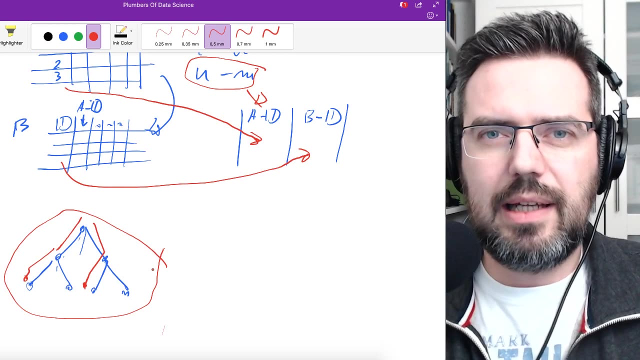 So you have billions of rows in that table And it's taking a long time. First, the index is getting very, very big And it's taking a long time to query a lot of rows. So if you're doing- let's say you're doing- a bulk. 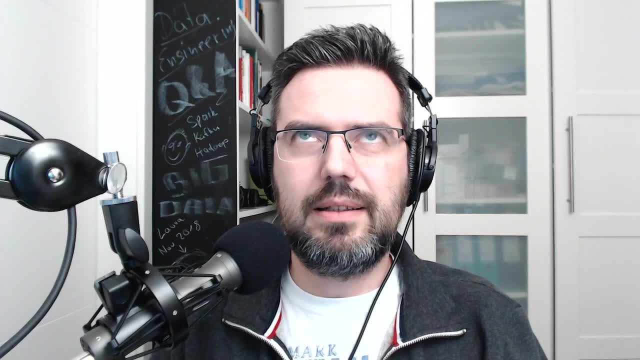 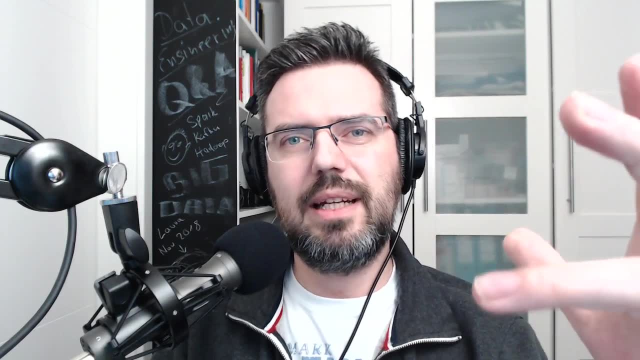 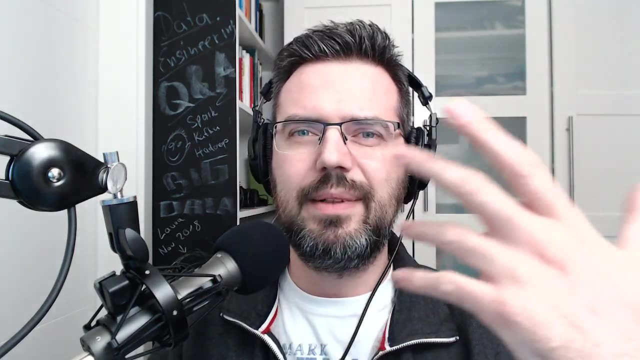 let's say you're doing a bulk- no, not a bulk- a batch process. So you're querying a lot of data and you're getting a lot of data into the analytics and you're processing it. Then you potentially, are going to extract billions of rows from this table. 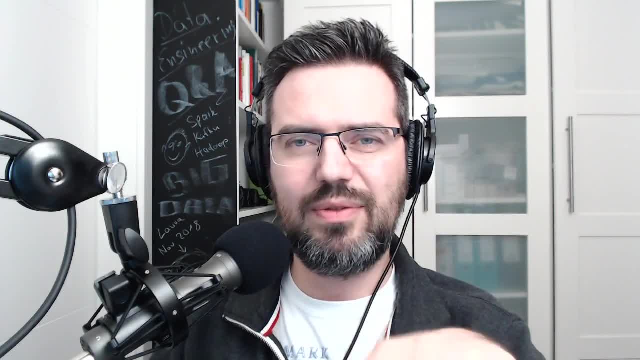 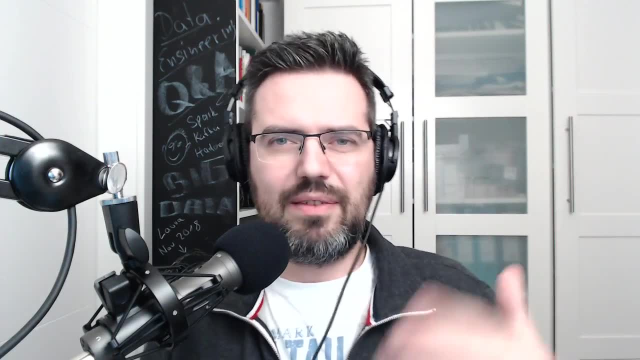 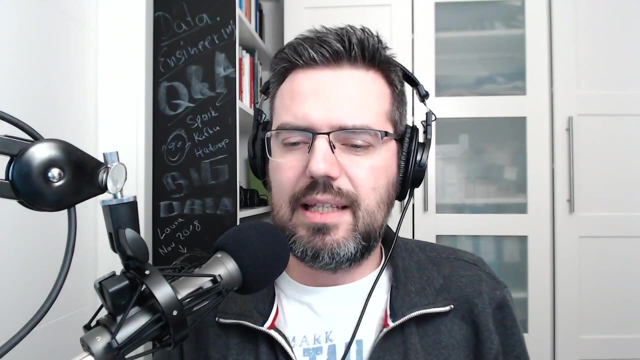 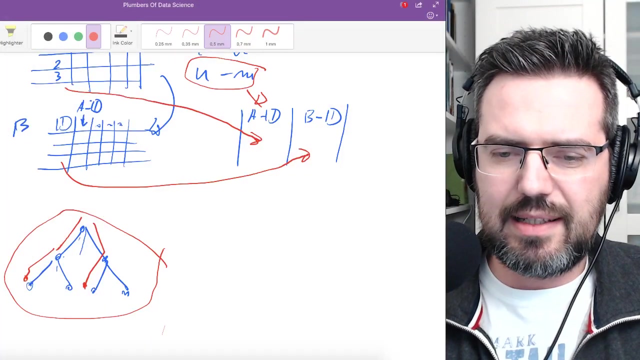 And it takes a long time for the actual database to find the rows that you're looking for, And this is a bit of a. this is a problem with huge tables with billions and billions of rows, And so this is one issue that you have, that the whole index thing. 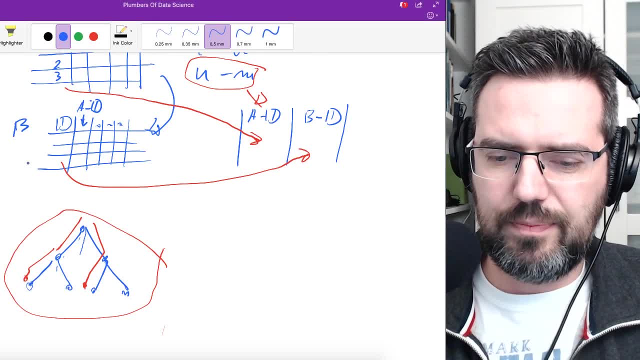 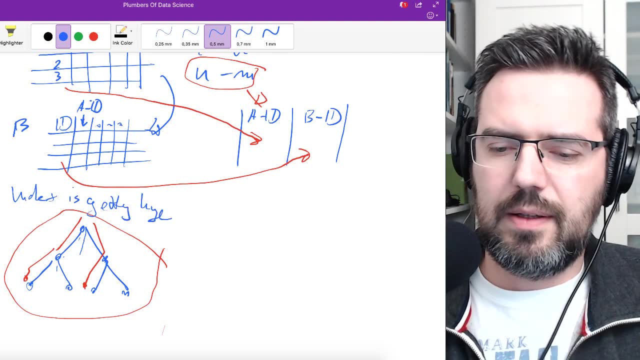 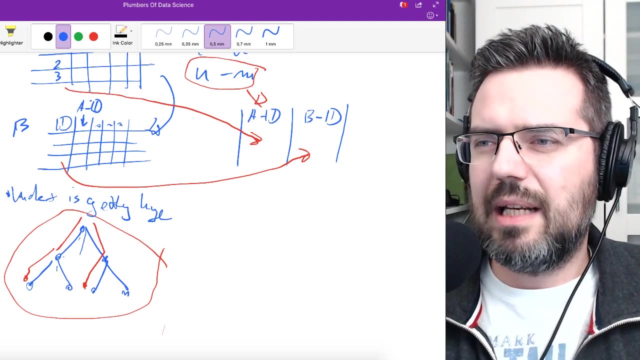 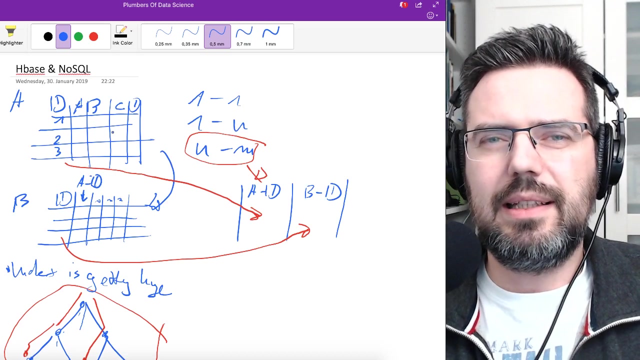 So the index is getting super huge And index is getting. This is one problem. Index is getting huge and it's taking a long time. The other problem with SQL databases is that you have to know the complete structure of the database and of the columns and of the tables before you start inserting data. 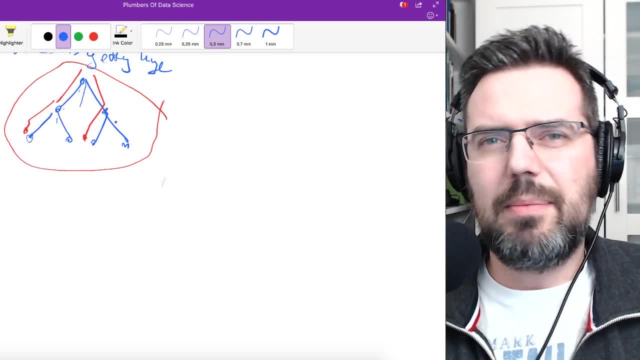 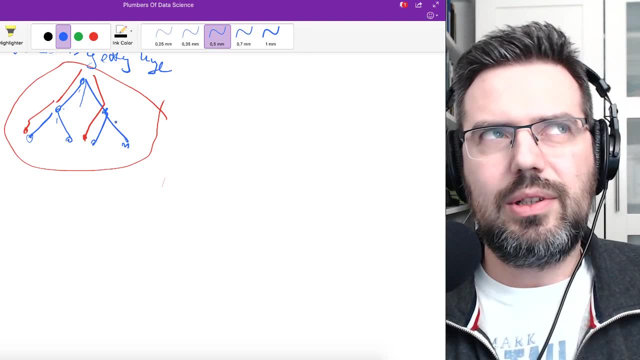 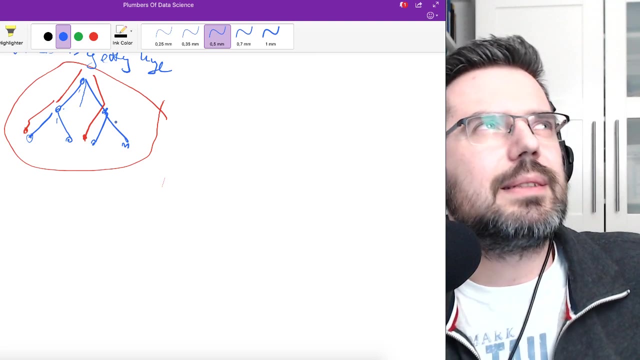 And this is a bit of a problem if you have. If you have, let's say, your system that is filling the data is how do you call this? It's very dynamic, So you can have, for instance, if you're working with sensors on something. 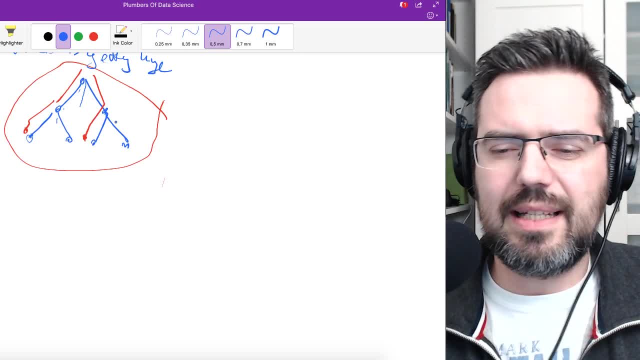 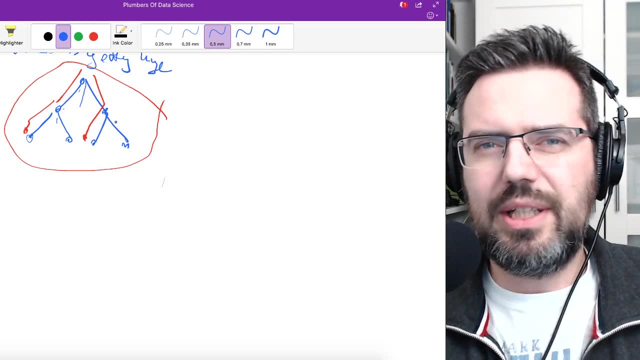 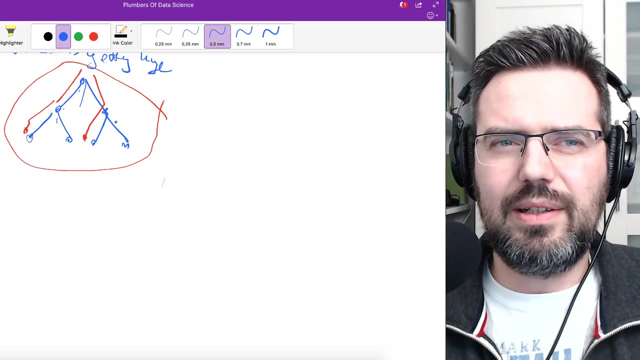 you have different devices and every device has a different type of sensors, And then you would need to set up a table for each device And each device type and define the columns and so on. And then if you are- if, let's say, you make a revision of a device and it gets a new sensor- 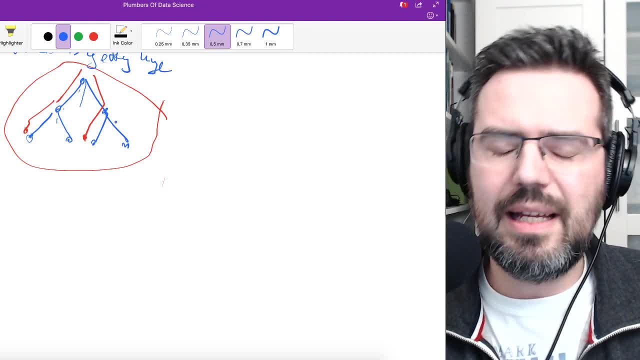 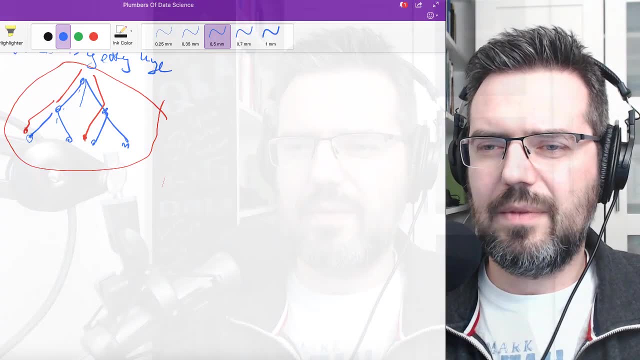 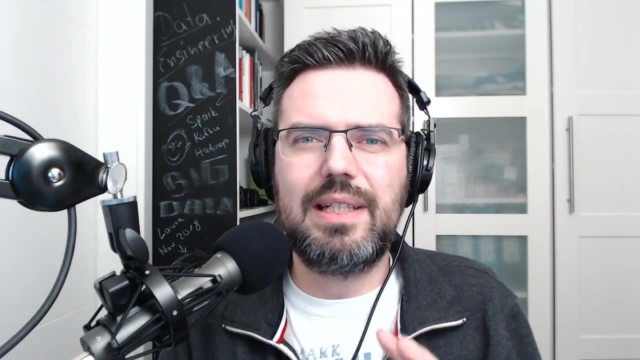 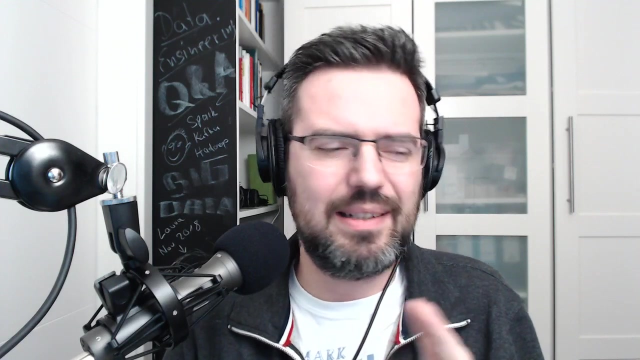 then you would need to modify the table and put in another column, And so it's getting very, very messy. to actually find the or have the structure of the table in the right, In the right way, or have it dynamic. This is more or less not really a good idea to do. 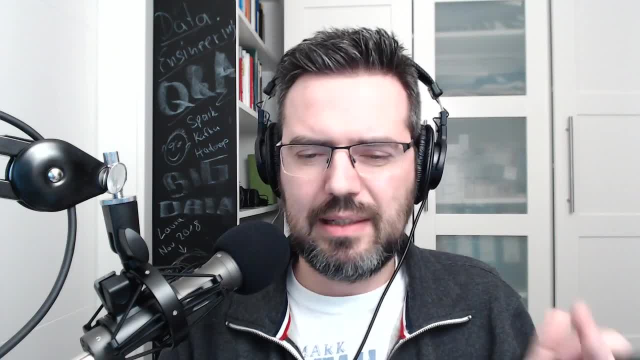 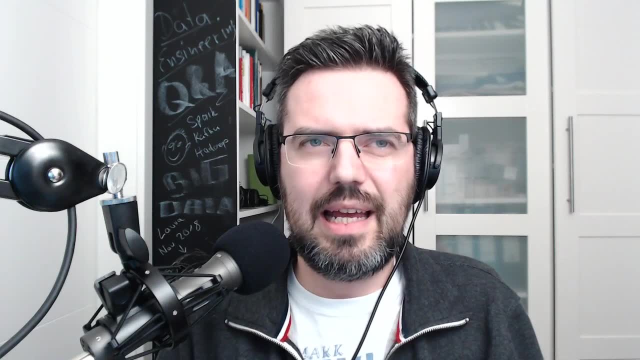 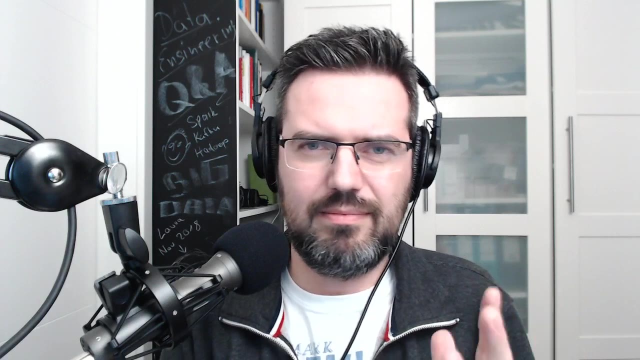 So yeah, The problem with SQL is the index problem. You're getting a huge index if you're having billions of rows in a table, or multiple billions of rows, And the other problem is the fixed column or the predefined column size or column. 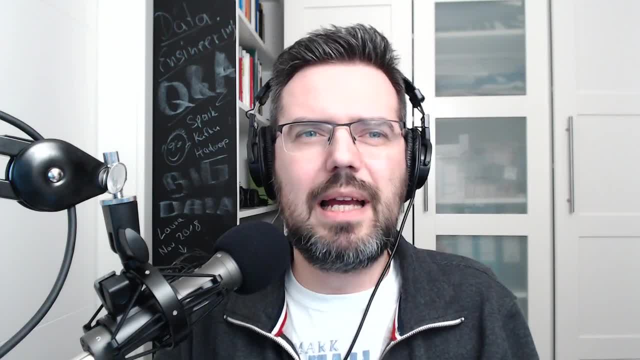 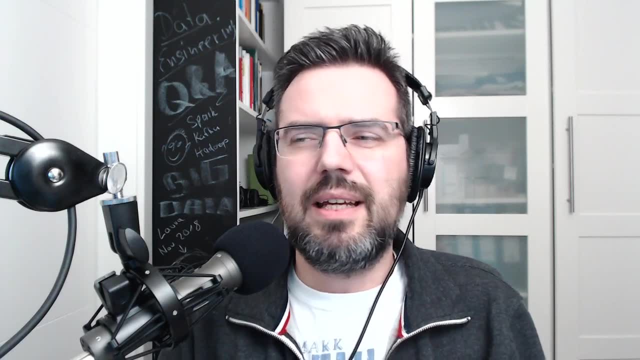 And this has to be done with the right type of data, And so one way out of this is to go with a NoSQL database, And a NoSQL database can be a lot of stuff. One thing that I'm very familiar with is, as I said before, is HBase. 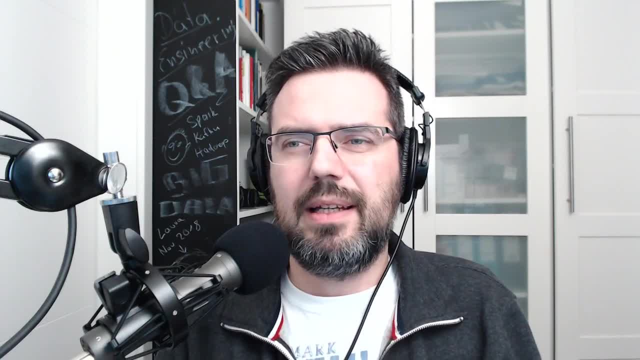 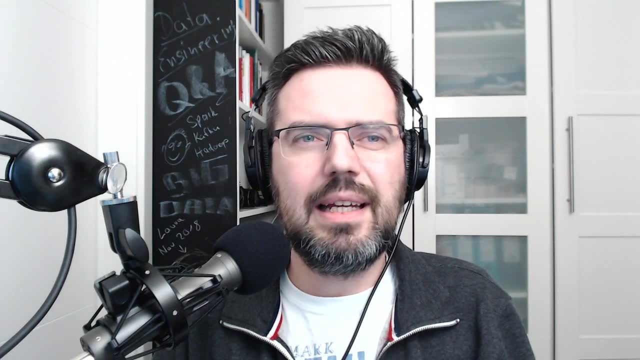 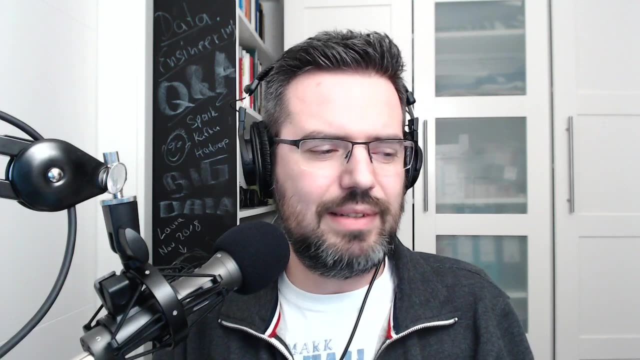 HBase, a database based on a Hadoop, And it's using Hadoop and HDFS in the background, But we're going to come to this in a second And this is made- Yeah, is made. basically, so you can put in as much data as you want and retrieve it in. 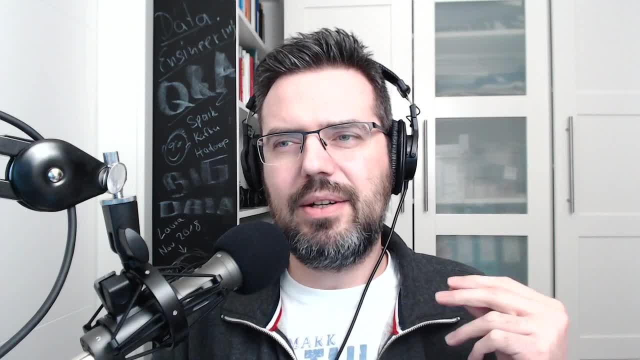 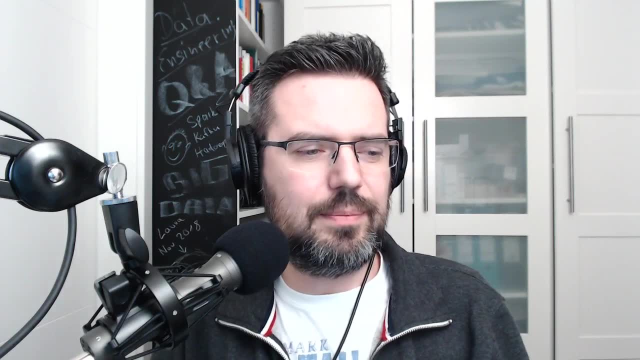 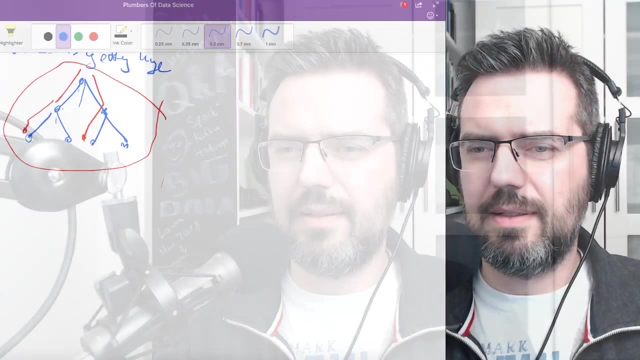 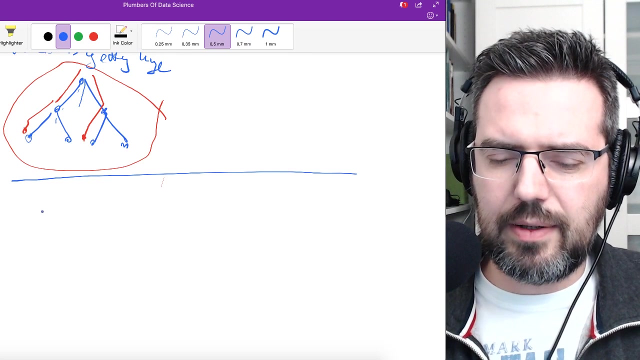 in bulk and retrieve it in a way that is very good for parallel processing. and how this, how all this works, is? it's quite simple. let's go back to the okay. so with HBase. okay, so what you have usually is, or what I said in a SQL: 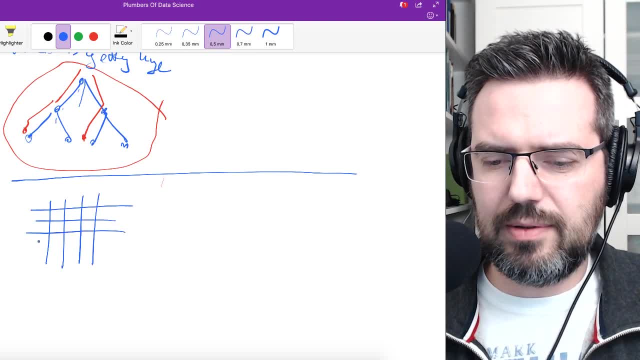 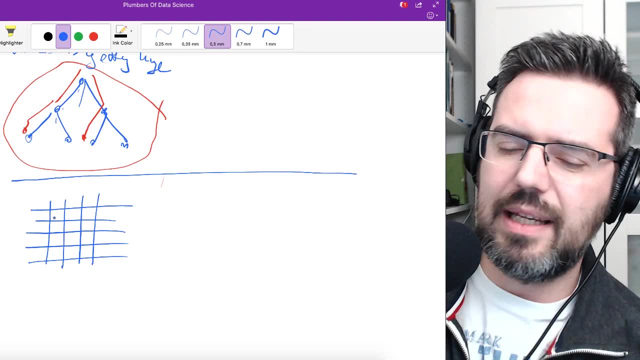 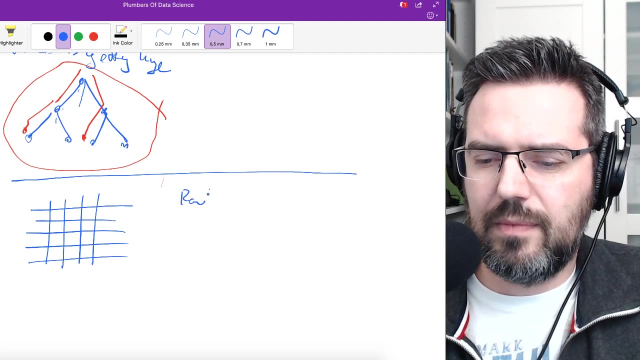 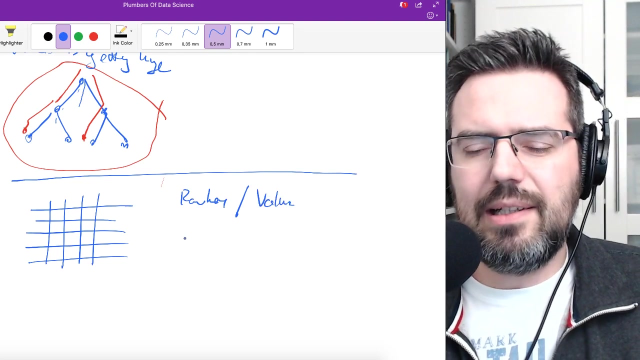 database. you have your columns and you have your rows, and what you can do with with a key value store, like HBase, is you can reduce this to having a row, key and, and basically a key and a value, and the idea here is that you're basically 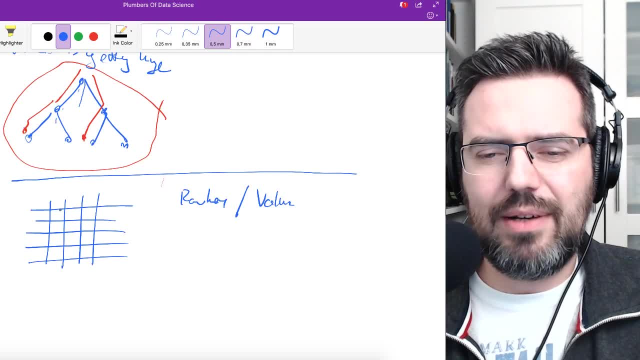 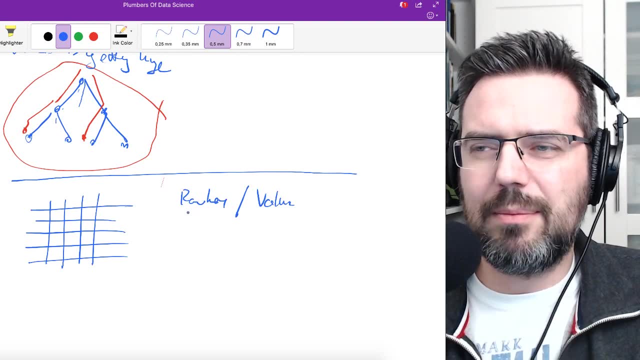 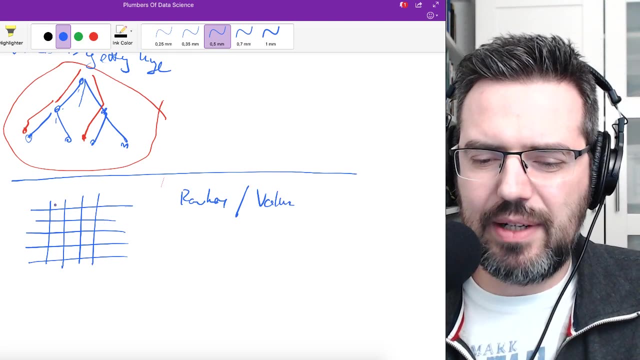 bringing. you're bringing everything together and make a very, very simple structure of it. so how this works is your. the row key is getting more complicated. it's called a composite key, and with a composite key, this could be, for instance: let's call it here: this is column A. 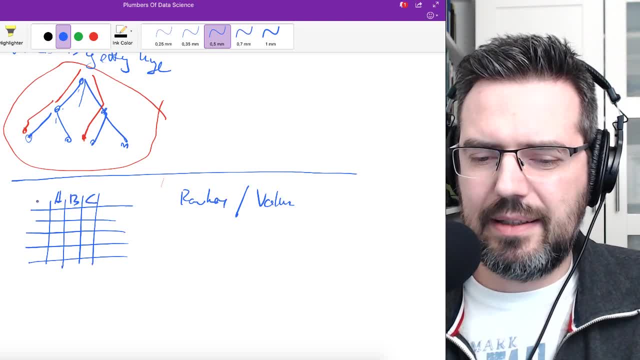 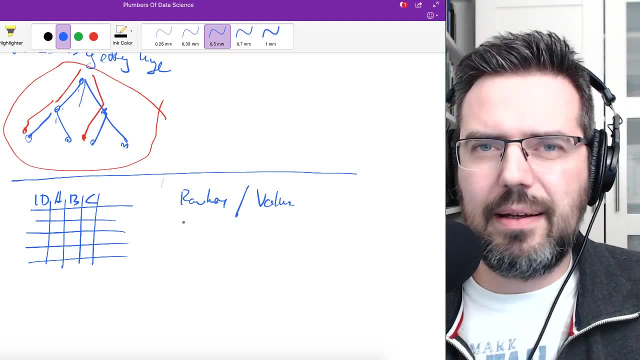 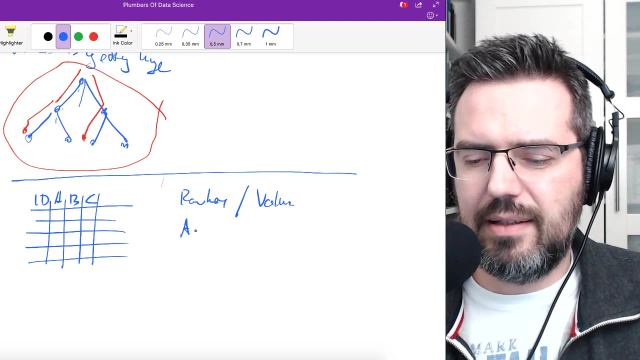 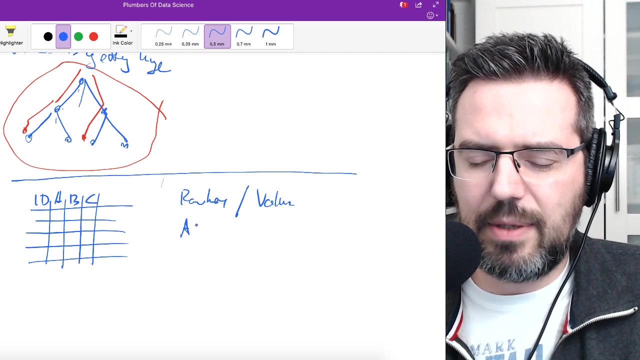 this is column B and C, and this could be an ID, doesn't matter. so what you're, what you could do, is you can put in the. you create a composite key with column A and then you're doing something like this: could be a signal or a special. 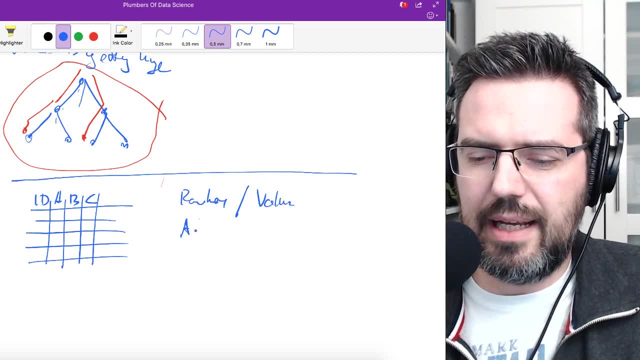 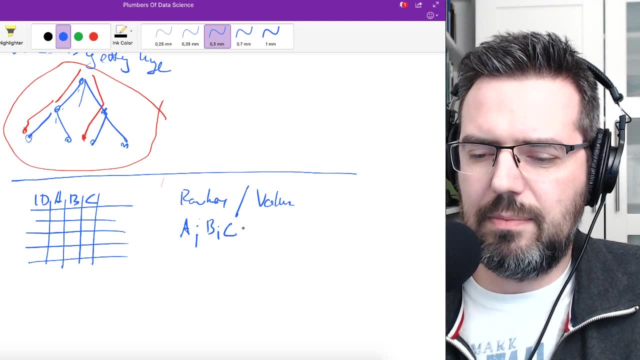 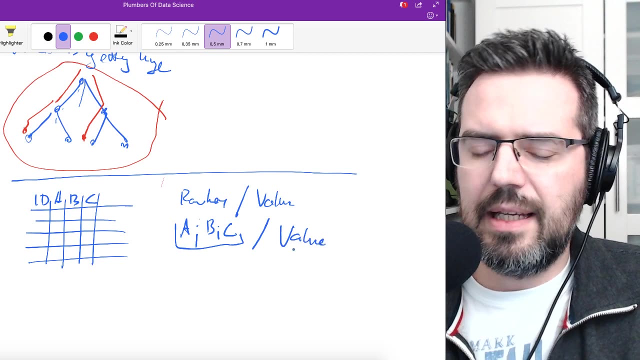 character like a slash or a comma or a semicolon, so you could do a semicolon A, B, semicolon C, then this would be your, your row key, your new row key, and then this could. and then comes your value. and the idea here is, with HBase, that every 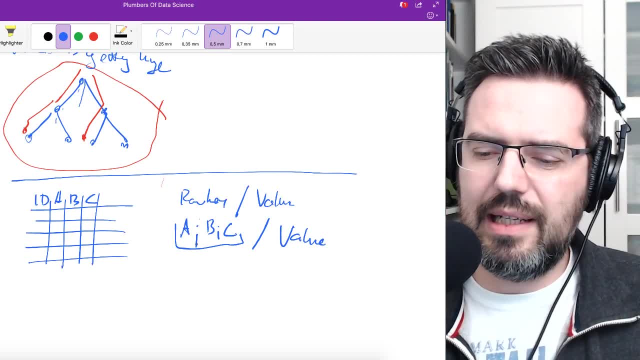 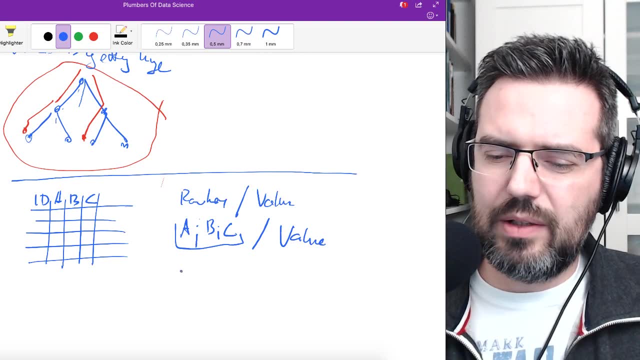 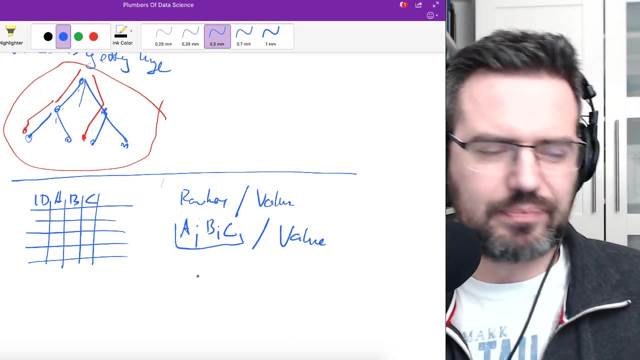 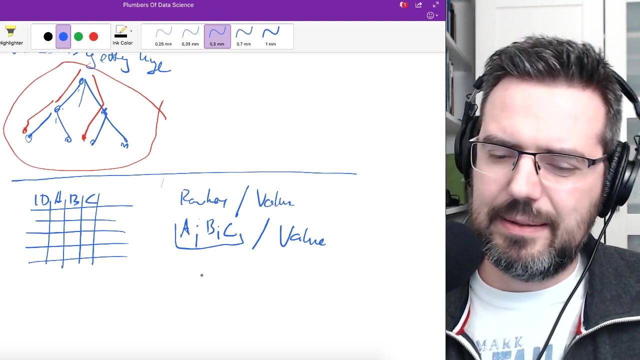 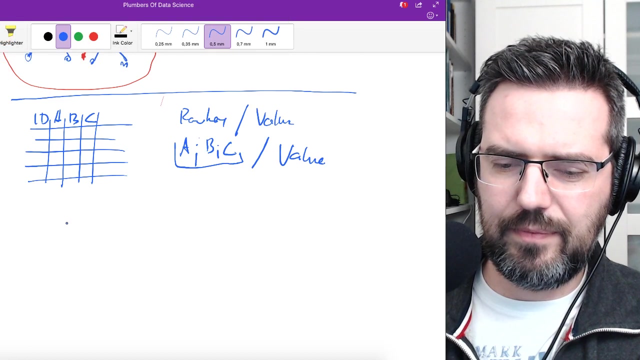 every row you're filling in, the filling in the database is getting solved. It gets sorted lexicographically. so you're filling, you're filling in, yeah, it's so. basically, the key gets sorted in a way. and why this? this makes sense is- you can look it like this: the what the system is doing is, let's say, or: 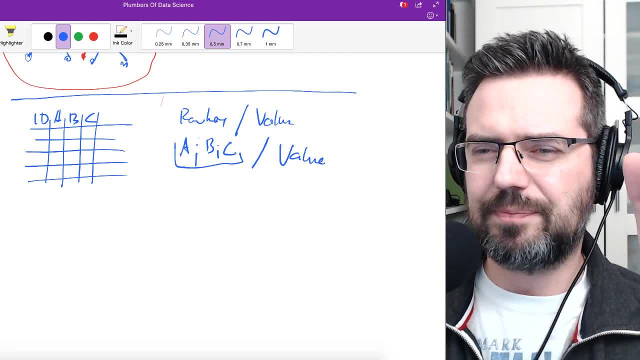 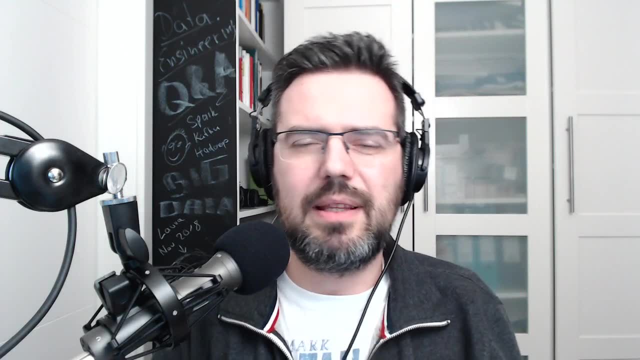 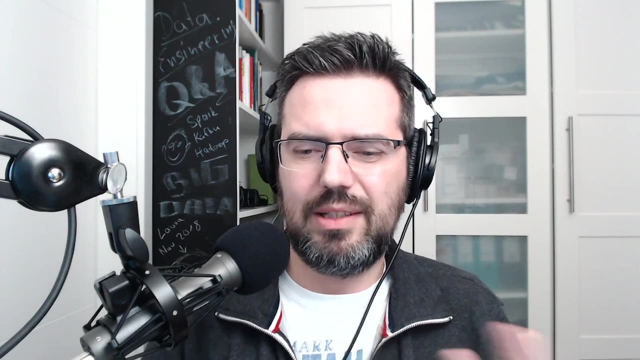 or let's, let's go like this way. you are now, if you, if you would have one table within HBase and you're filling this table with a lot of data and at some point you need to query it, so you need to get some data out of it. and how do? 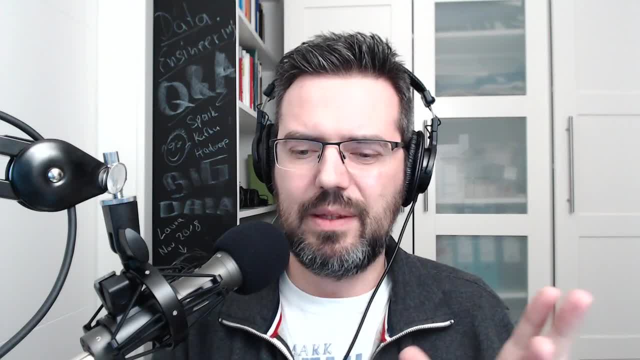 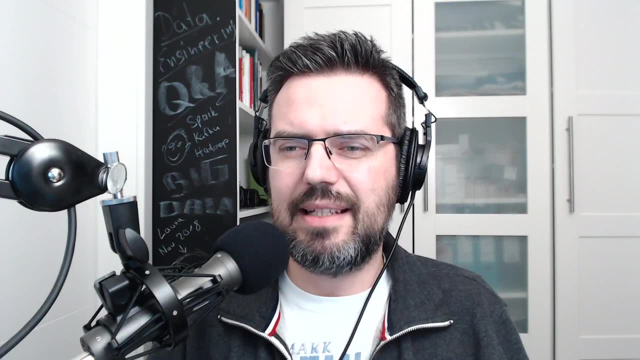 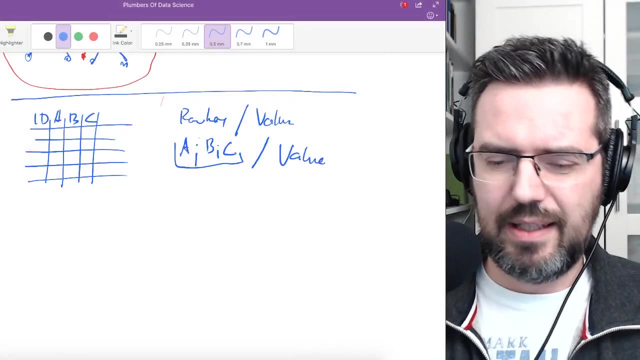 you find this with SQL database. you have an index where, like with a binary tree, as I showed, and how does HBase handle this? and it's. this is very simple. HBase is doing regions, and how this works is you have the row, keys and HBase is basically. 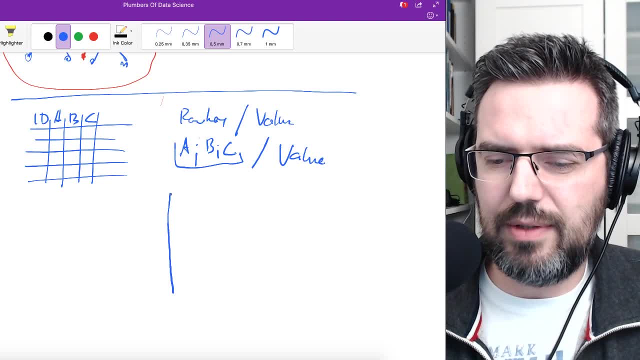 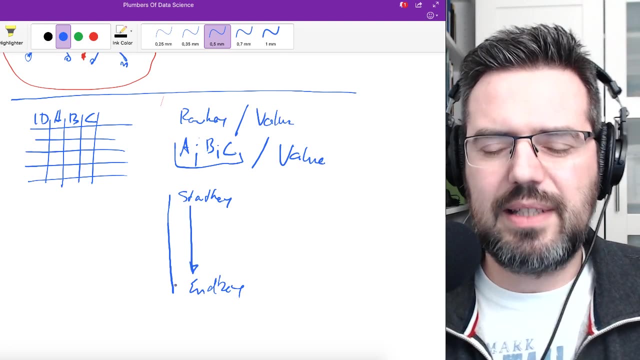 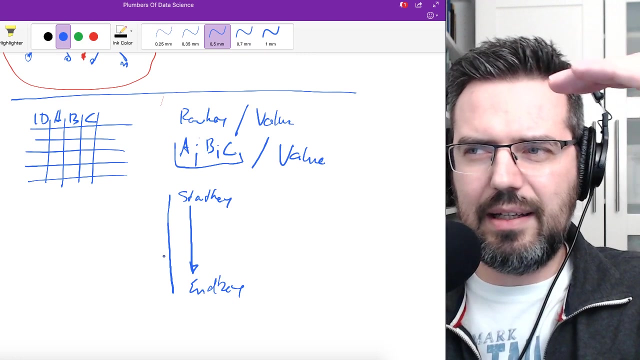 putting them together so you have a region. this region has a start key and an end key and within the region everything is sorted. and so if you say, now you have a, you have many, many regions. and the idea is, when you're you're querying uh data for, for instance, a batch job, then the system knows in. 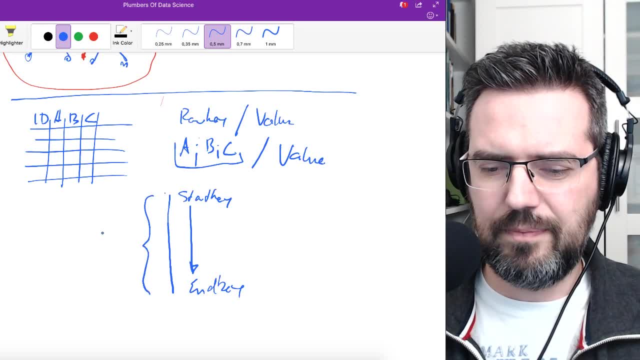 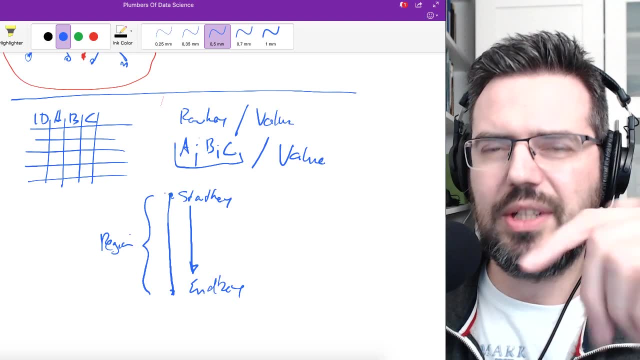 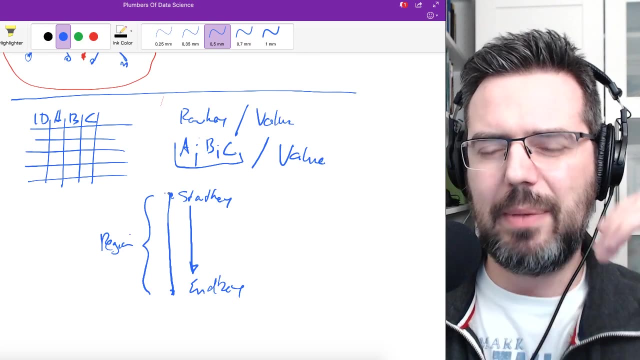 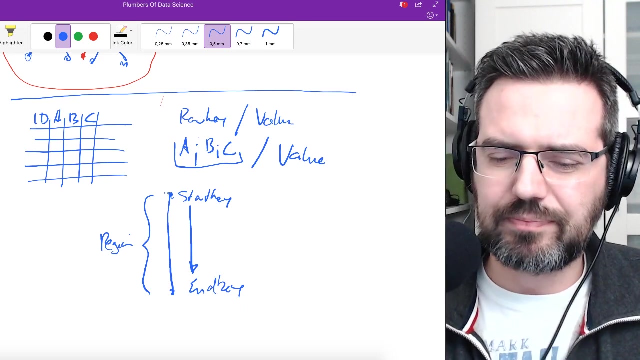 which this is a region here. so the system knows, um in which region it has to look, and this is a very interesting concept- so that um you, basically you can fill in as much data as you want. at some point it's going to switch to a new region and then the system knows which region you. 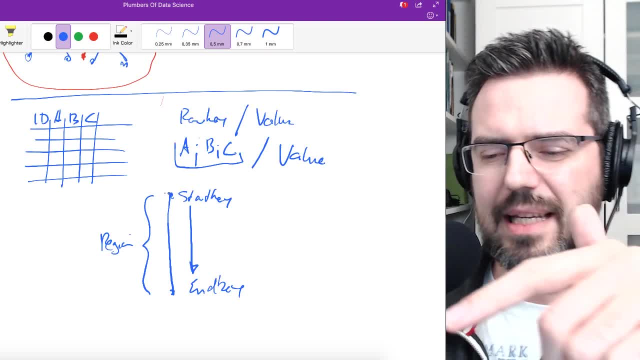 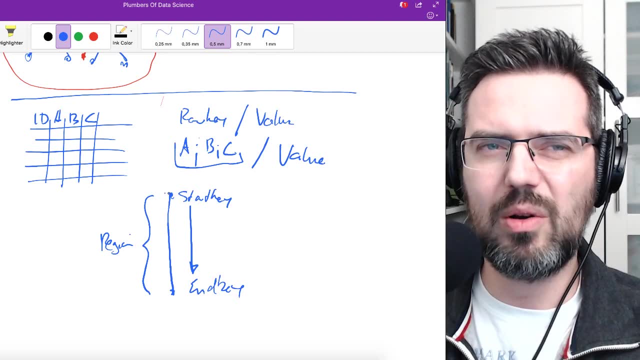 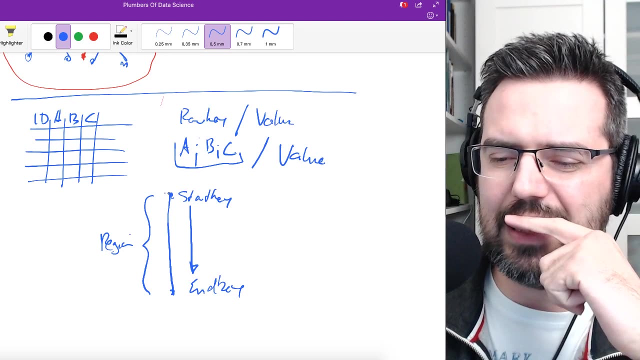 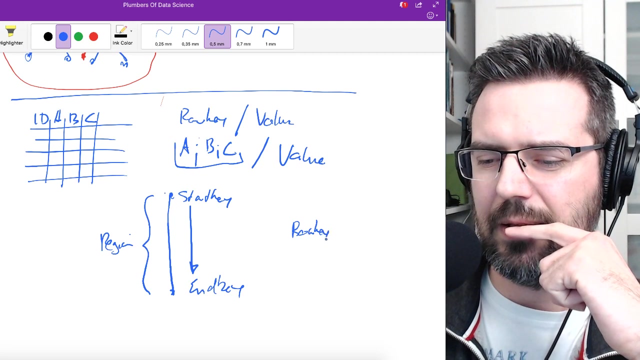 you want to query data from and how this works is you can it? hbase is a is a key value store. you can have also columns within this and and the columns are packaged within column families, and so the idea is you can have, you can have here a, you have your row key, your composite key, you have a column family. 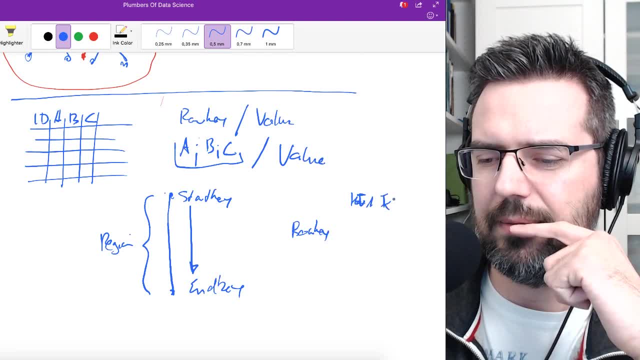 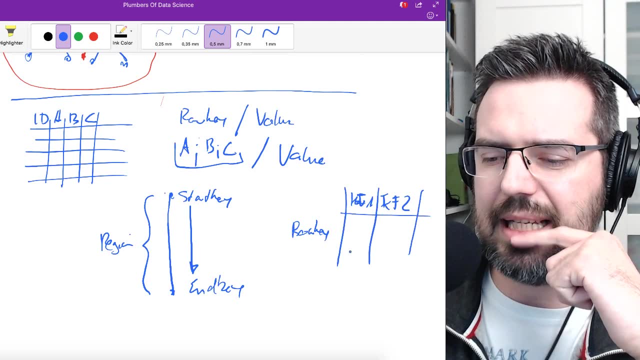 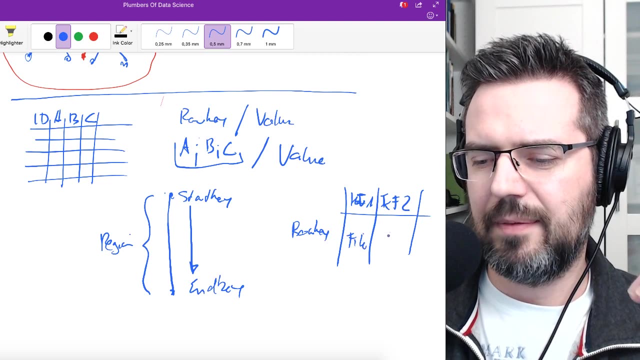 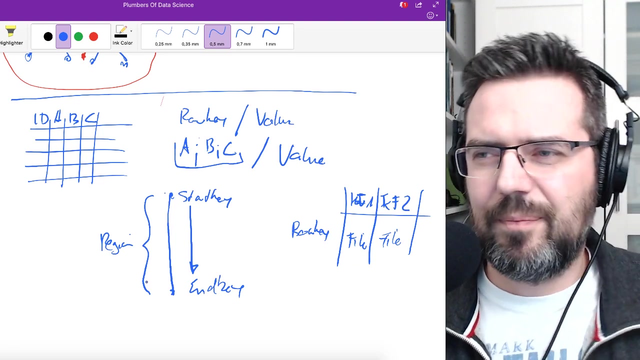 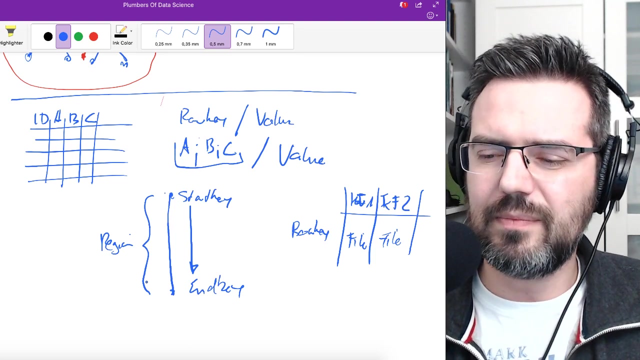 column family one column family, column family two, and each of these column families has its own. basically is is its own file in hdfs and you have regions for each of those column families. so um, basically you're because in the background of hbase is running um, is running hdfs and data is stored in hdfs in files. 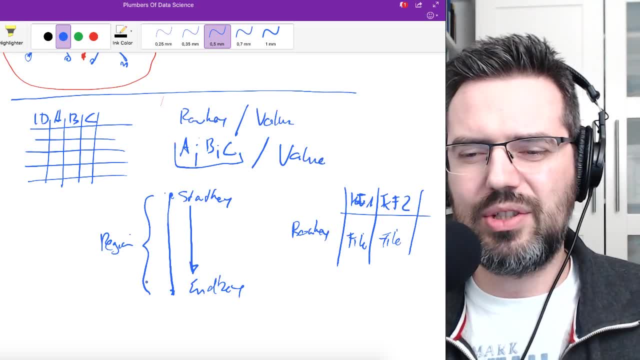 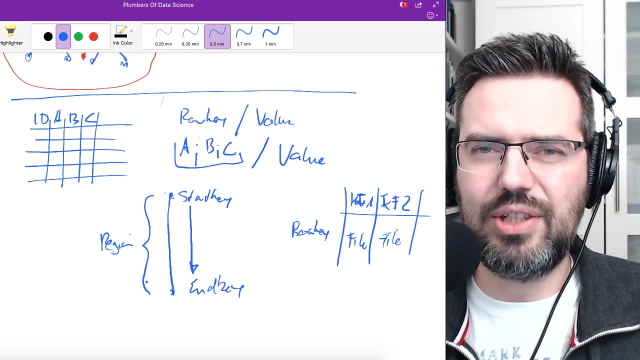 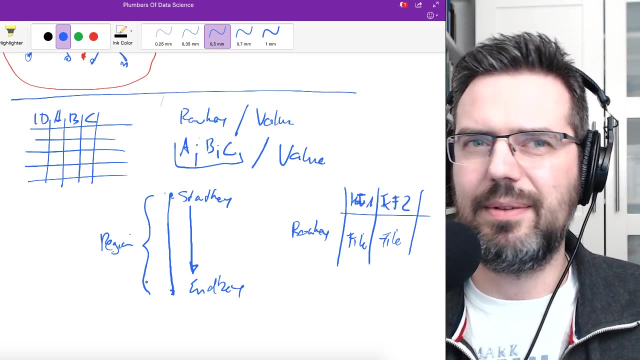 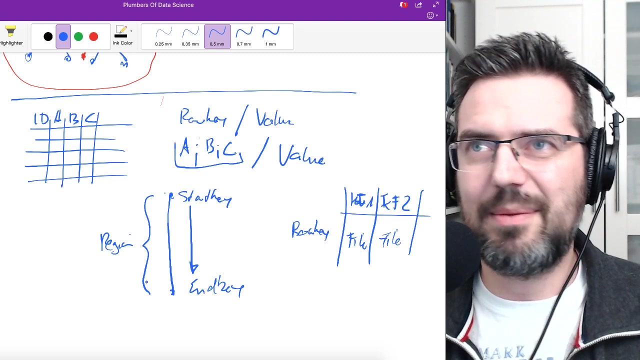 so if you're in in on the system and you're going in hdfs, you can go into the hbase folder and look at the data that is stored within each of the regions and you can basically see it in raw text. so, hi guys, if you have any questions, don't hesitate, ask questions. i'm going to get into it. 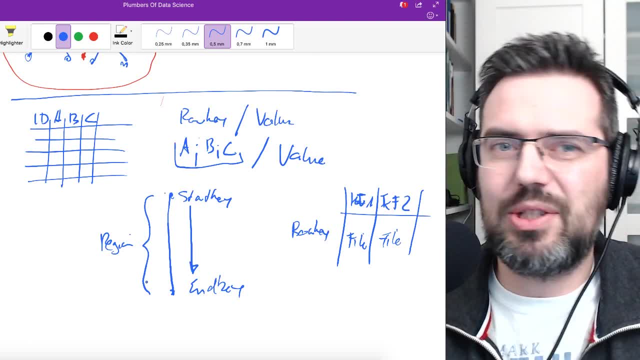 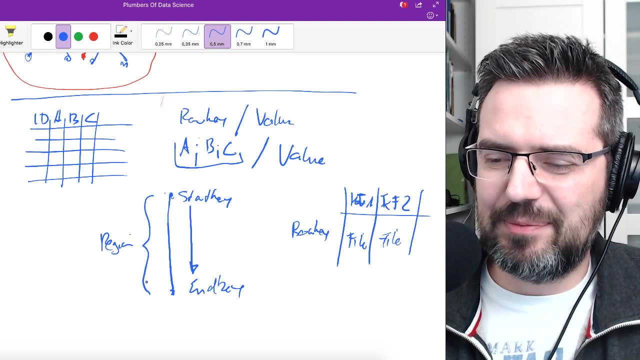 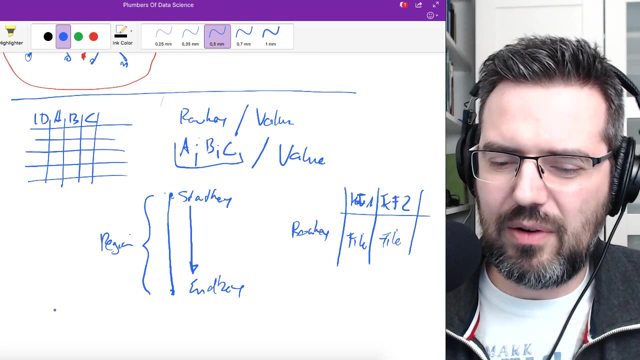 i have a lot of time today, so no problem. any question you have, i'm trying to answer it as good as I can. yeah, so this is the the idea here, without behind this you have, you have all those regions and the the cool thing- why is this done this? 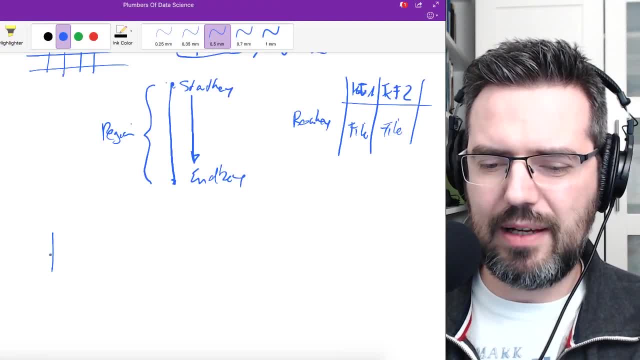 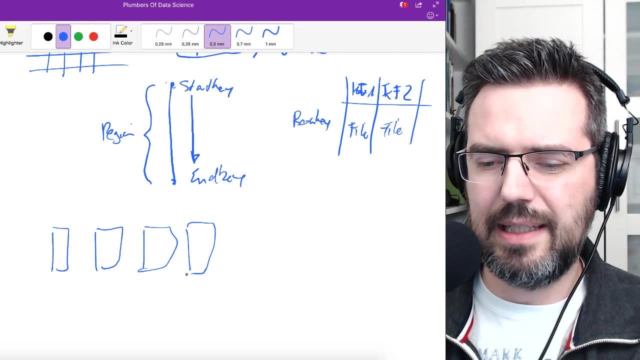 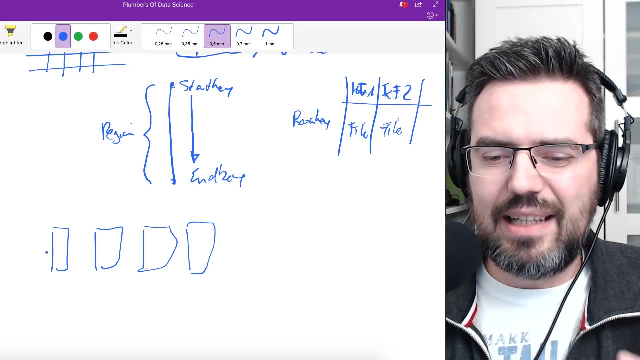 way. it's done this way. so you have your regions- let's say you have three regions or four- and you want to query data from the regions and you have a lot of data in the regions. then you can parallelize it because data is in. HDFS is on. 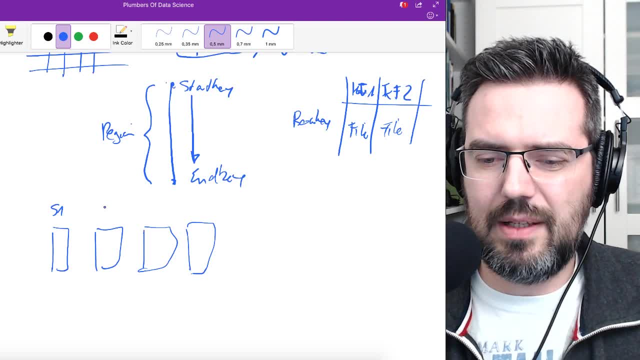 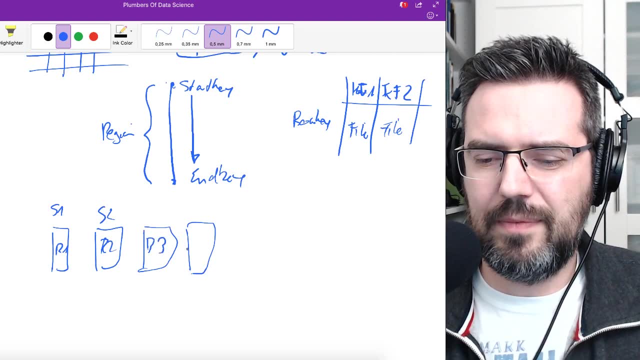 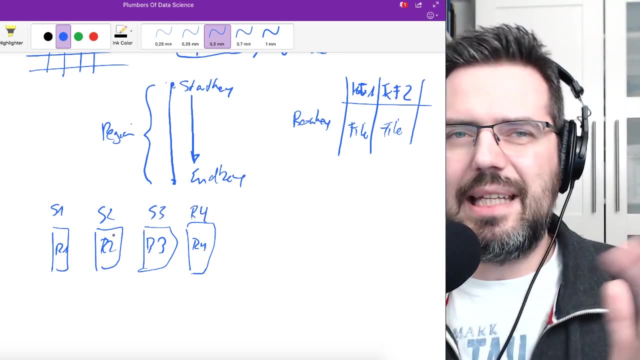 multiple servers. so this might be server1, this might be certain. so region one which in one region to reach in three region, for this might be in server three, Litchfield, four, might be several seven, be in server 4.. So the regions are distributed over the servers and usually the regions are. 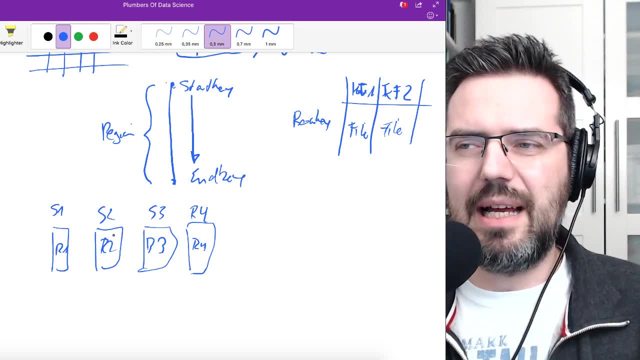 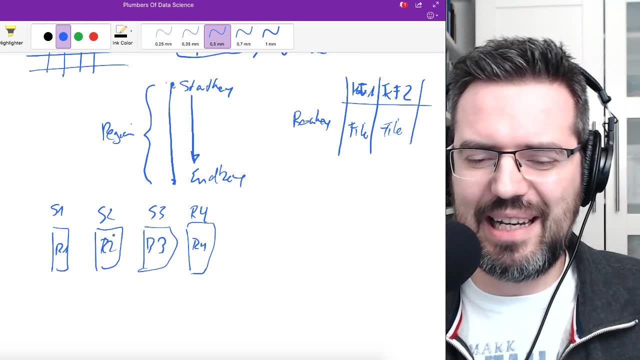 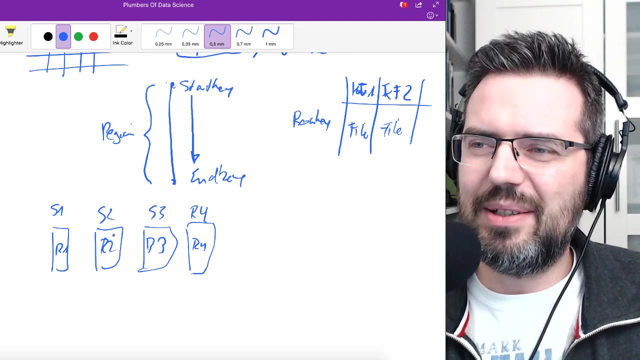 also distributed multiple times, so you cannot lose any data, although the data is also replicated within HDFS. But now it's getting too complicated. So the idea here is to have your data very, very parallelizable. Is that a word, parallelizable? I have no idea. 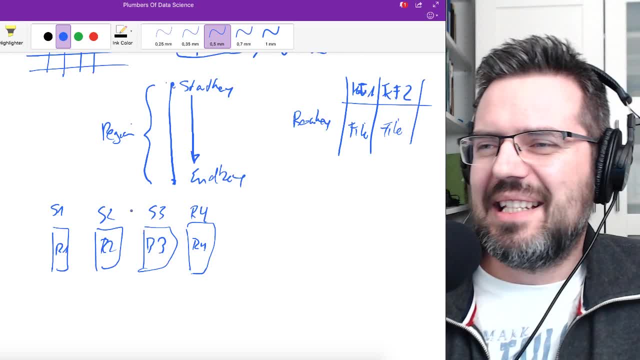 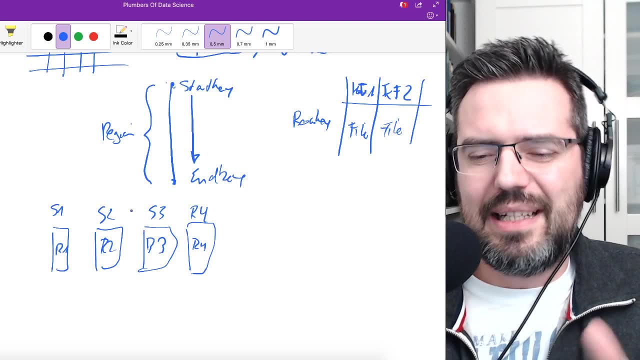 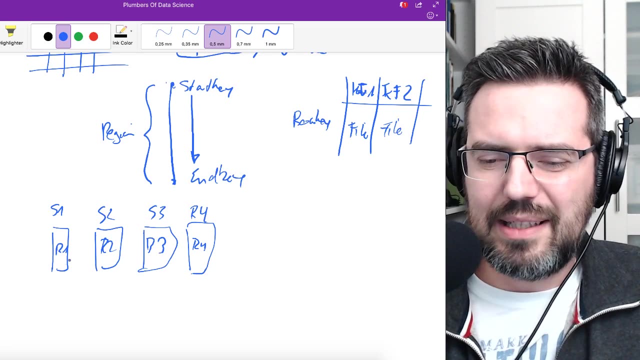 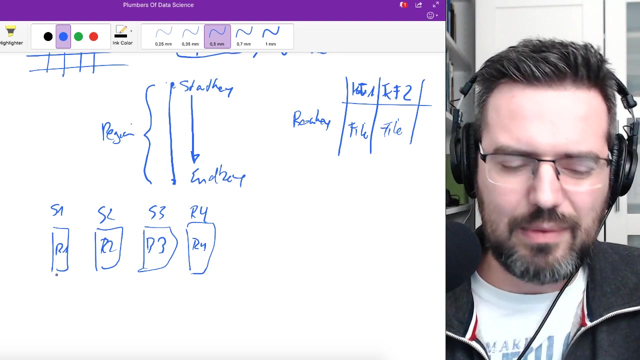 Yeah, so this is then the idea. This is why it is so quick and why you can't process so much data within HBase at a certain or at one time is because it's already in parallel and you can do very, very simple the processing At first or in the older days you've done it with something like: 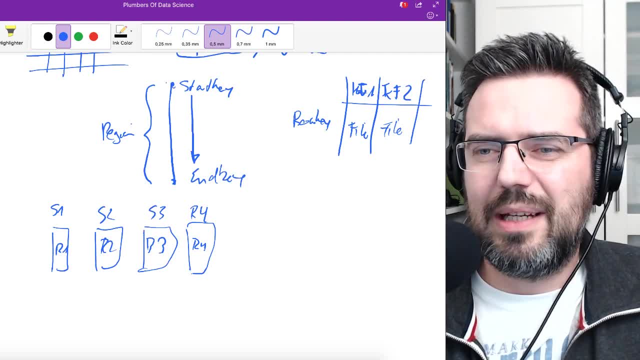 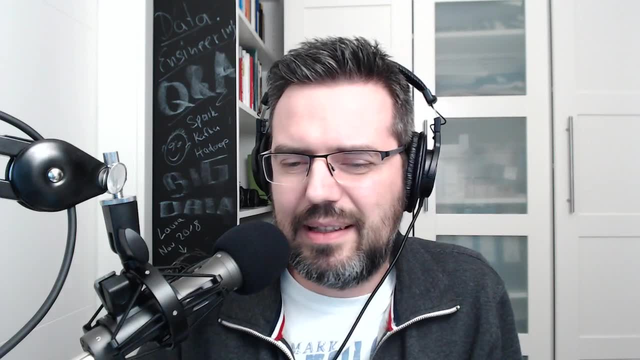 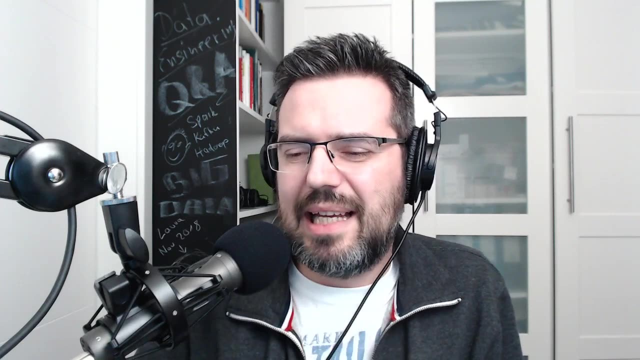 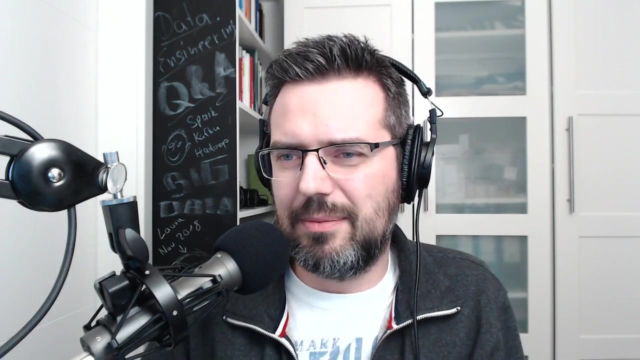 MapReduce. Today you're doing it with something like Spark or something. So this is basically how this is working. The only thing you need to be wary of is now, when you're you need to think about. let me go back. One problem with HBase is you have the regions. 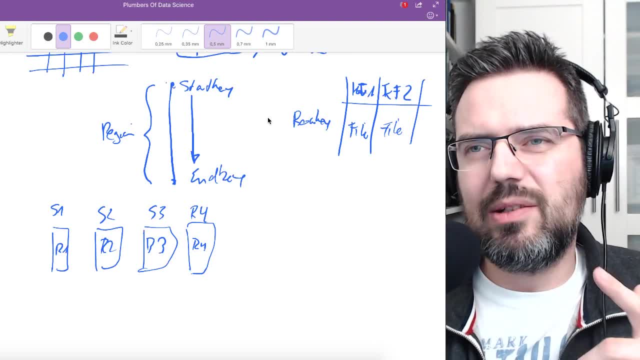 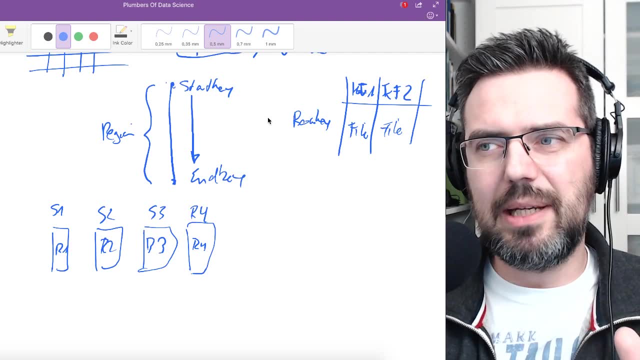 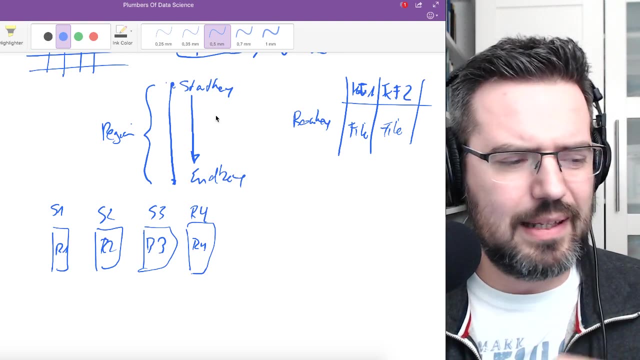 and the data gets fed into the regions, and so you need to, before you start working with HBase, you need to think about how do I, how does the data come in, and how do I want to query the data, because what you can have is something I think it's called region hotspotting, region hot swapping. 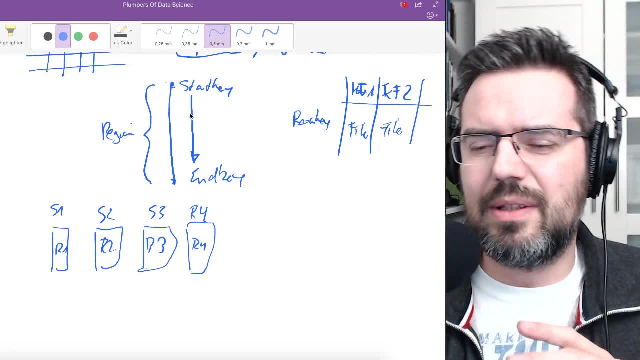 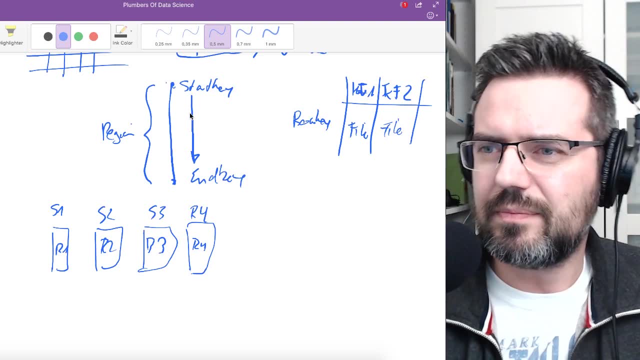 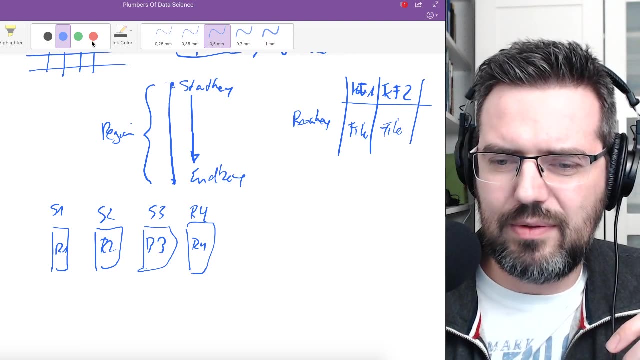 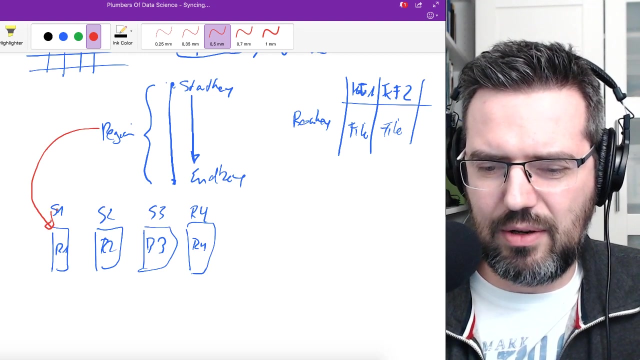 no, I think it's called hotspotting. So you have regions that are that are very, very, very much utilized. A lot of data is coming into one region and if that region is running, regions are only running on one server. So let's say, this region here, this is living on server one. 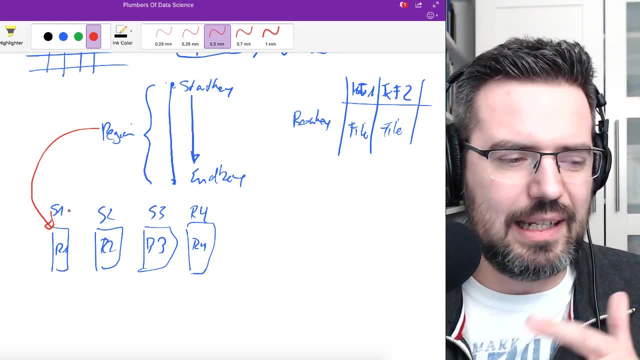 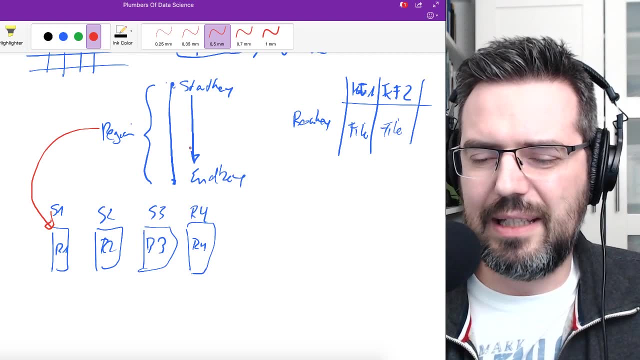 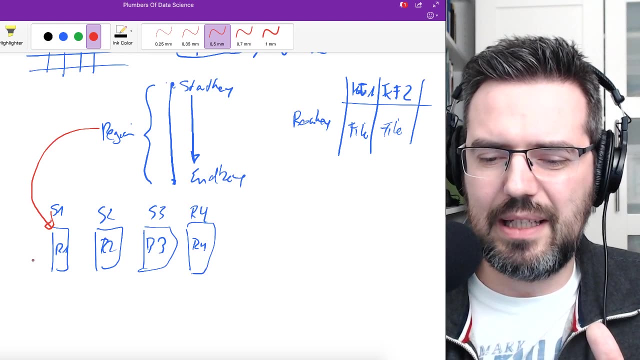 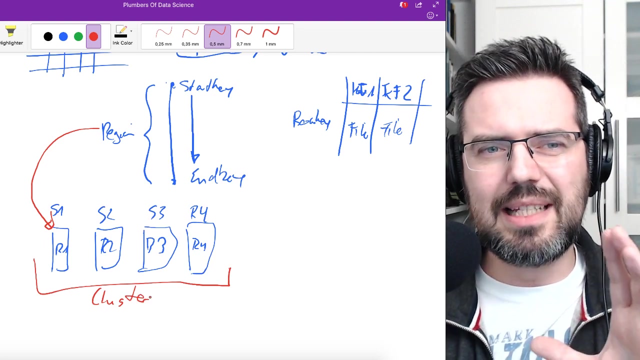 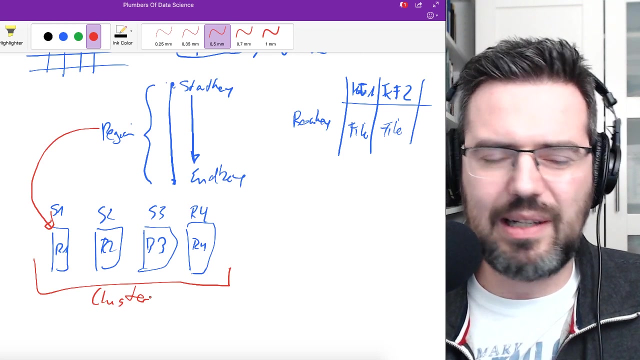 and server one gets all the load and you're getting into trouble with server one because your design of the of the composite key is not optimized to have the data distributed over the over the entirety of the cluster. And this is one thing to to make sure about or to think about when you're, when you're starting with. 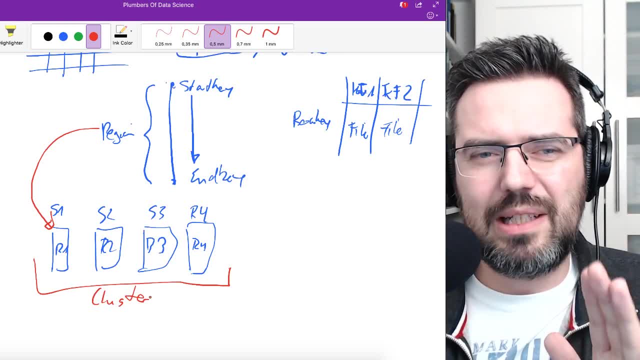 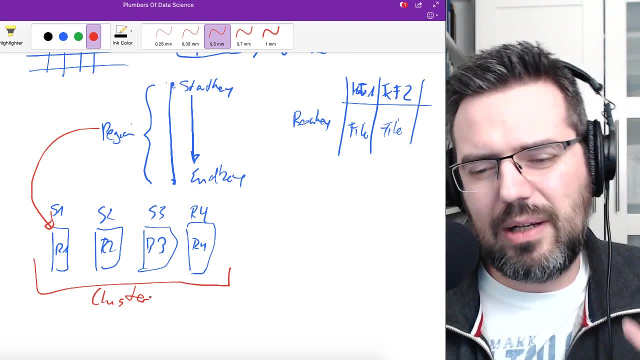 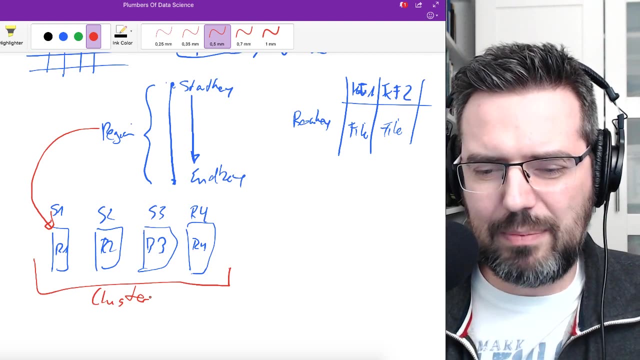 with something like HBase. So you also need to think before beforehand, before you start with something. how do I, how do I want to send the data in, because if you're doing the composite keys wrong, you can overpower one of the servers- and how do I want to get it out? because if you do this, 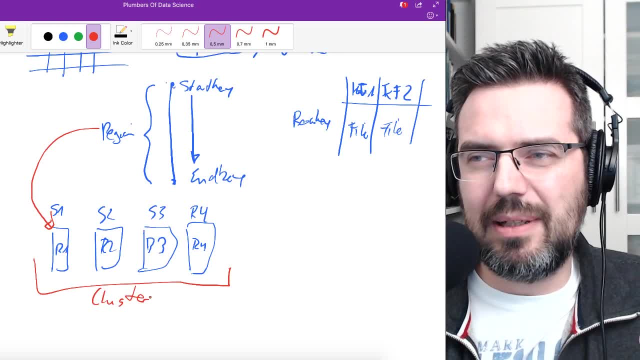 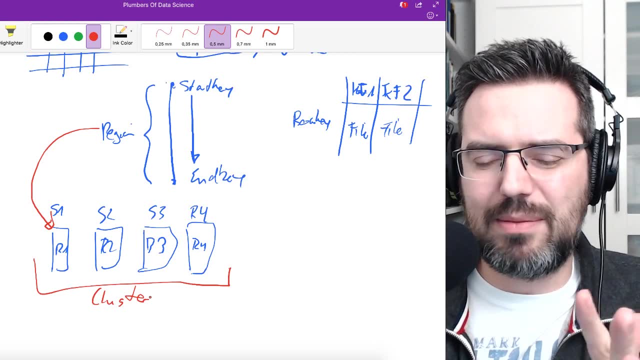 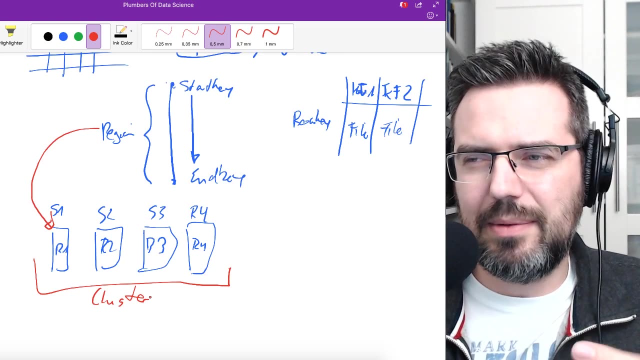 the wrong way, you're also getting in trouble. The thing is this is always a trade-off. You cannot limit or you cannot get out of this problem At some. sometimes you have to live with the problem that inserts are are a bit tricky. sometimes you have to live with that dating data getting out. 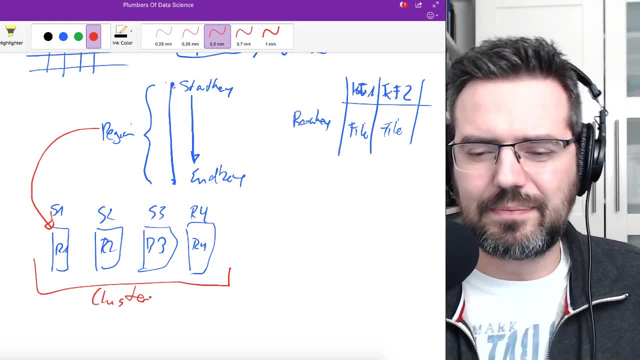 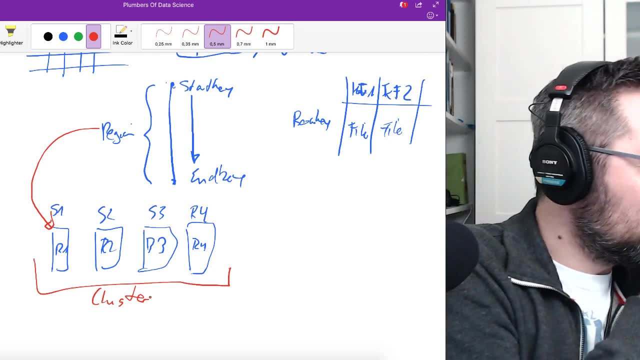 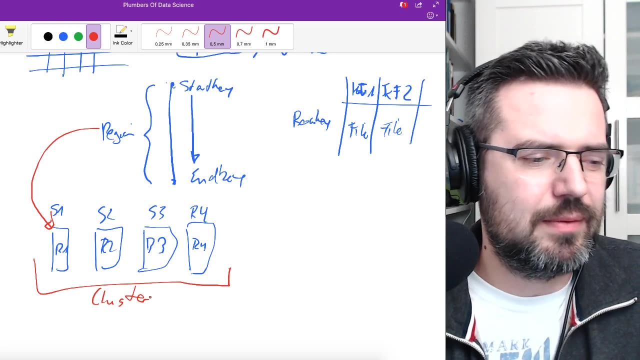 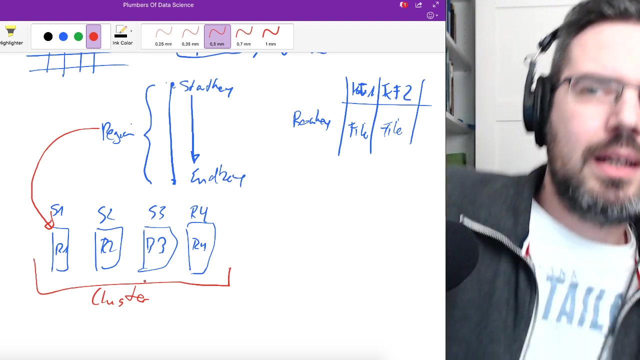 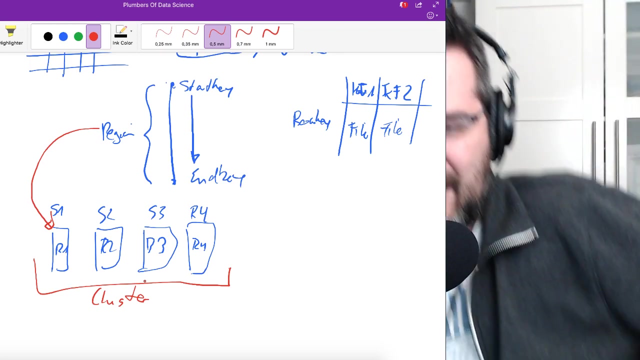 can be a bit problematic, but this is, this is something, yeah, you have to, you have to basically live with and and need to plan for. yeah, all good so far, guys. so i think i think this is a. this is a very, very interesting concept with hbase, one other cool thing that you can do. 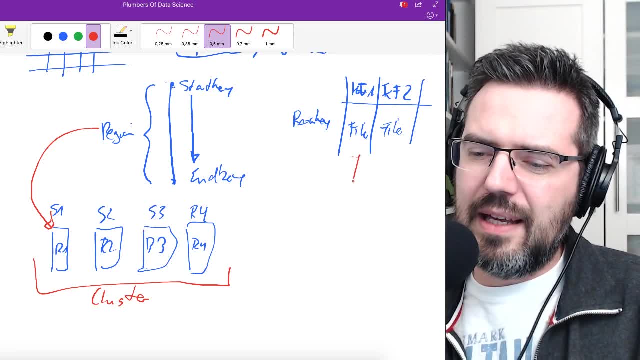 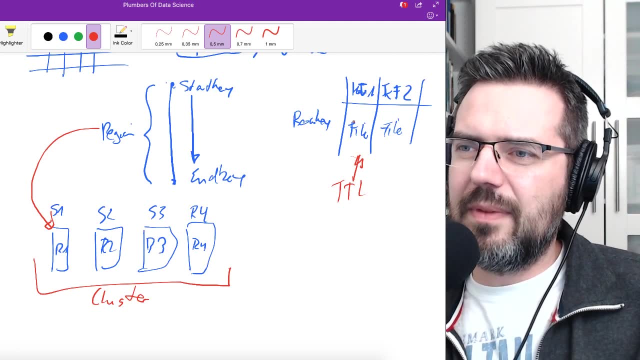 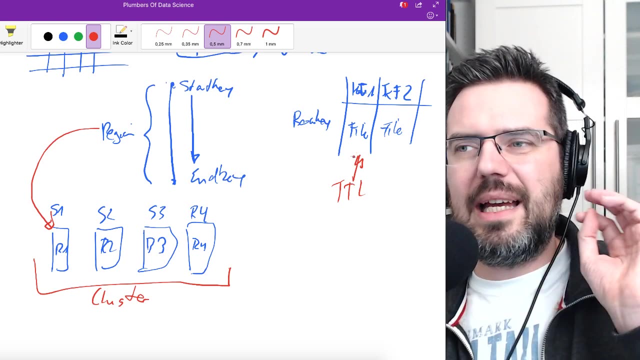 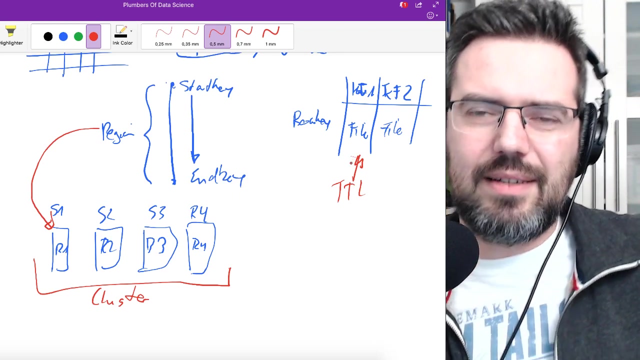 is with the column family. every column family. you can set a time to live so each so. so, for instance, you can simply put in data, put in data into the column family and set data. set the time to live for three days and then it's gone, so you don't need to write deletes or something. 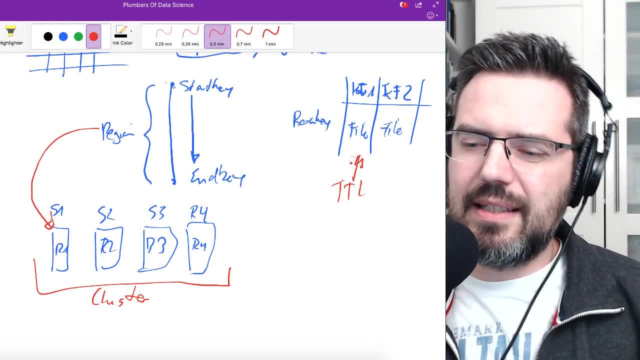 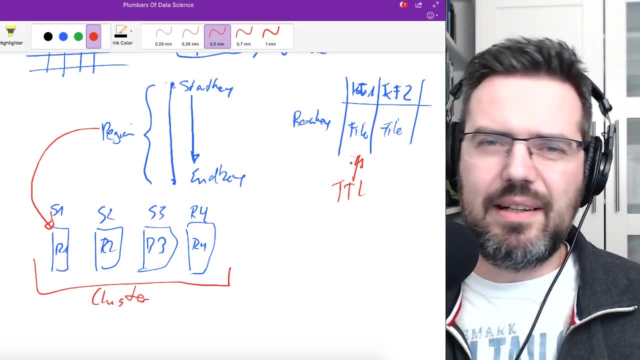 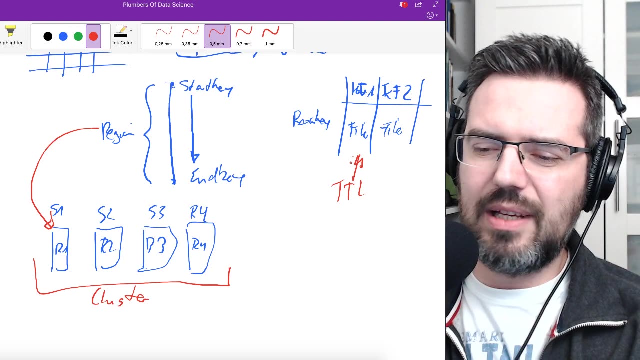 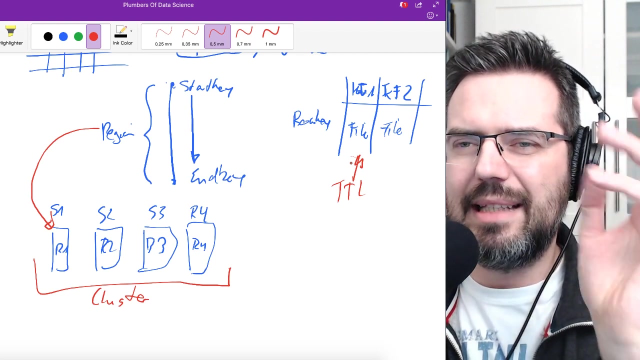 just set the tdl and it's gone, and this is very, very comfortable. another thing is that if you're doing inserts, you can just insert. for instance, you can. there are no updates of rows. if you're making another insert with a row, then it's it's super simple that it just gets overwritten. 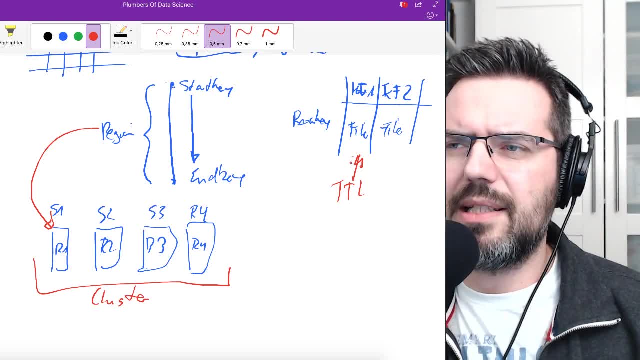 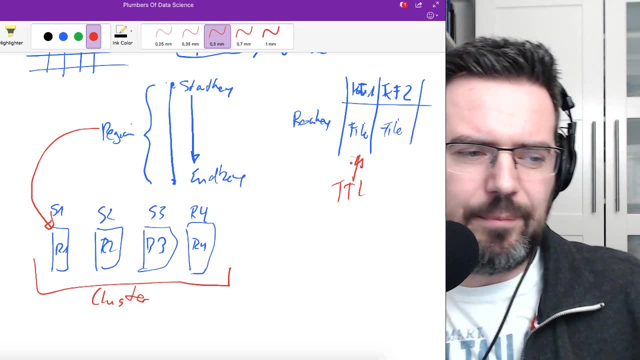 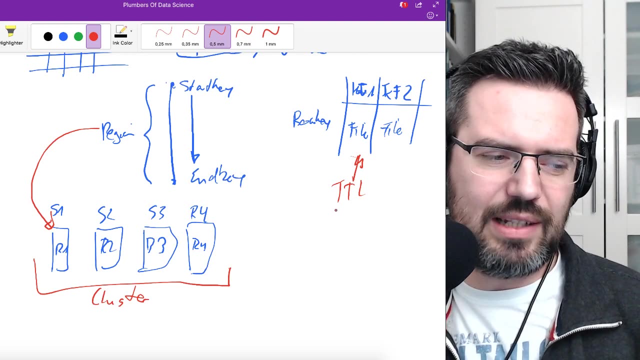 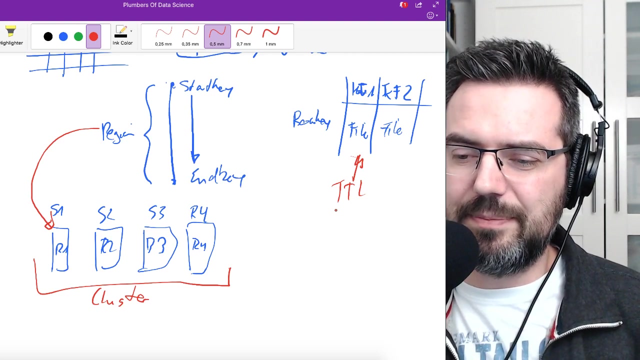 and i think you can have three versions. it stores three versions of one row to uh, yeah, to basically um get out of again. so it's. this is also a cool feature that you can. you have already a built-in a system where you can have the, the past two um. 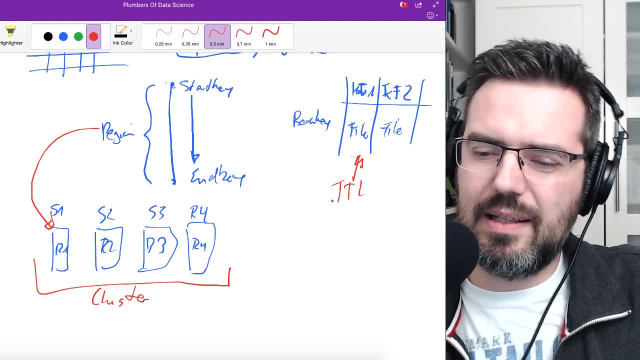 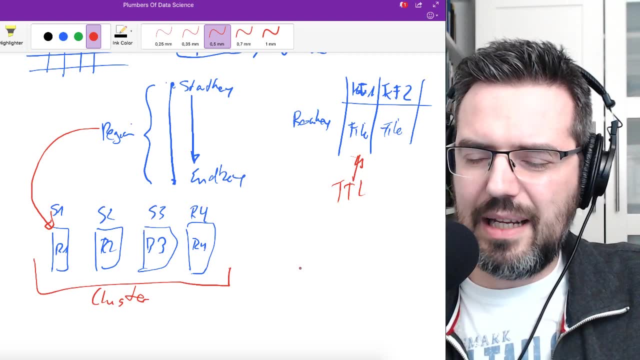 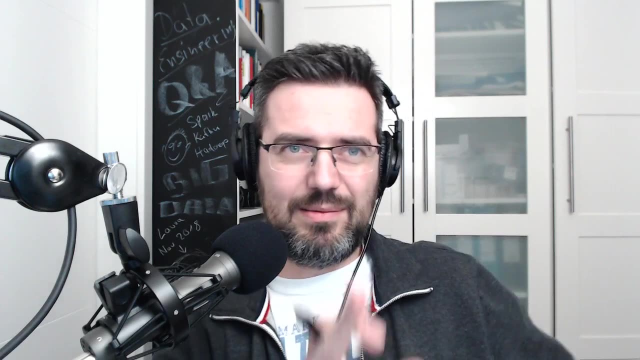 the past two versions of a row. it's super interesting. another very, very cool thing within um hbase that i that i remember um right now i have actually um- i haven't actually wrote this down on my, on my short list, what i want to talk about. 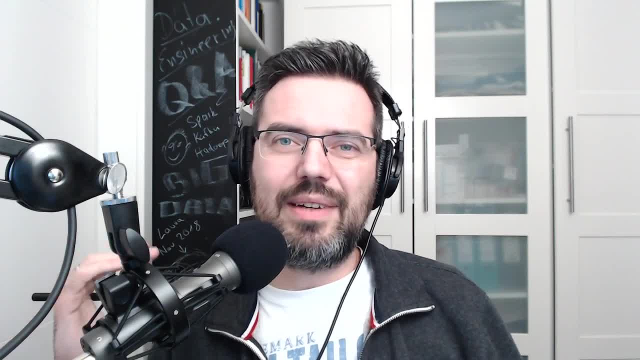 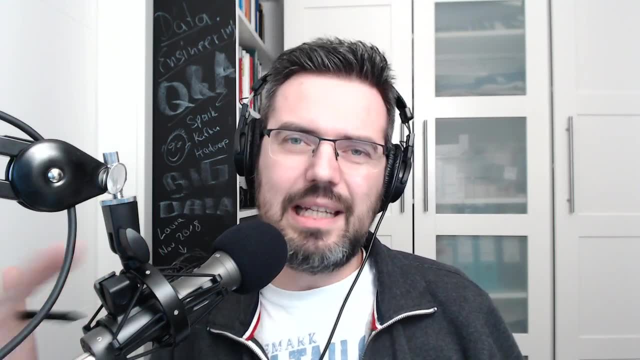 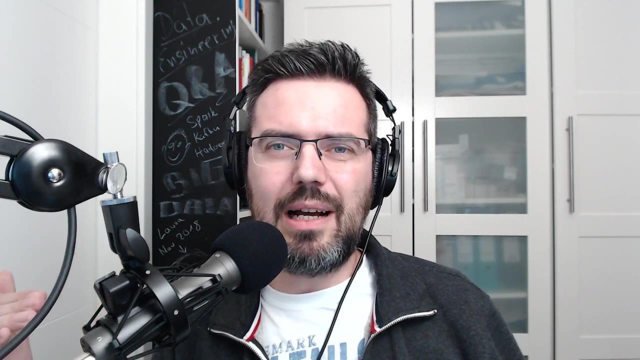 another cool thing about hbase is having counters. you have a, a system within hbase that is that enables you to do counters, so you can increment and decrement. can you decrement counters? i think you can also decrement, yeah, so you can increment counters at will, and this is a very interesting feature that you can also add to your project. 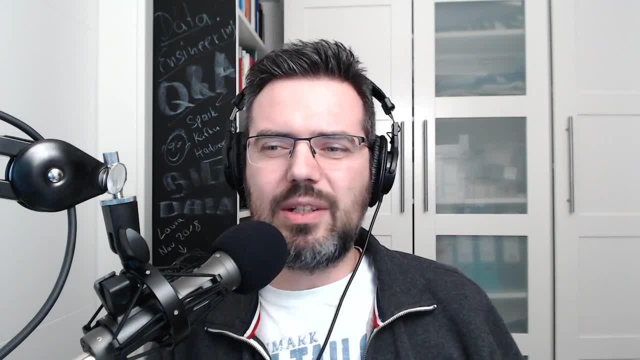 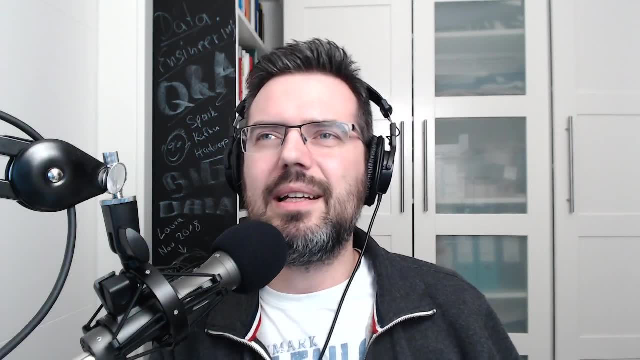 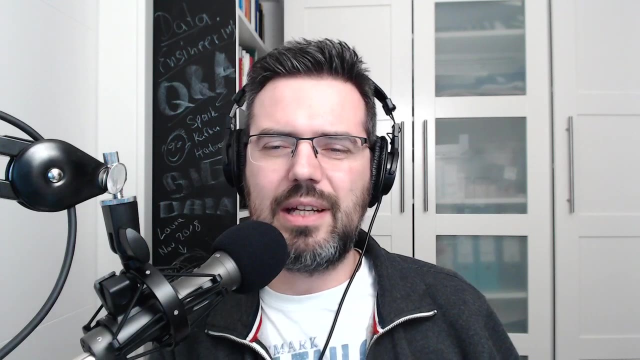 feature. um, so you, you don't need to, you don't need to, uh, get, basically, you don't need to get the counter value. and then, uh, add the counter value before, or, or add something to it and then write it again. you can just say, okay, do an increment of 10 to an increment of a thousand. 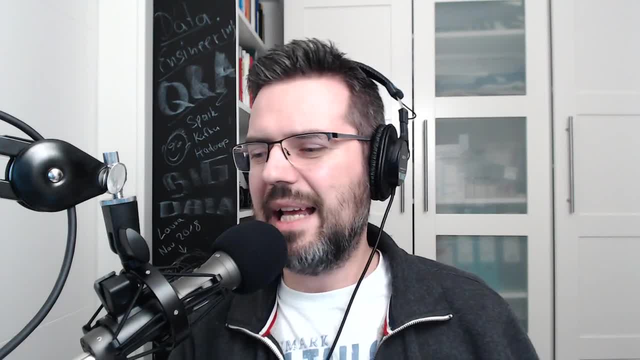 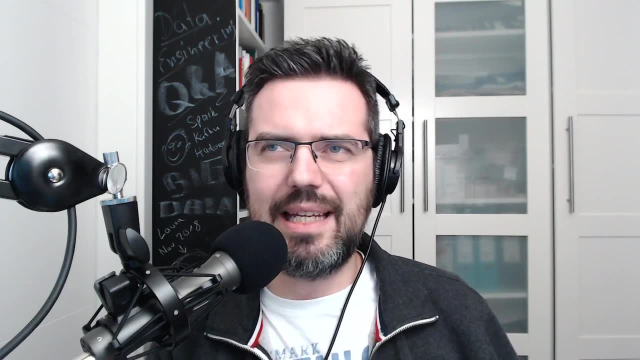 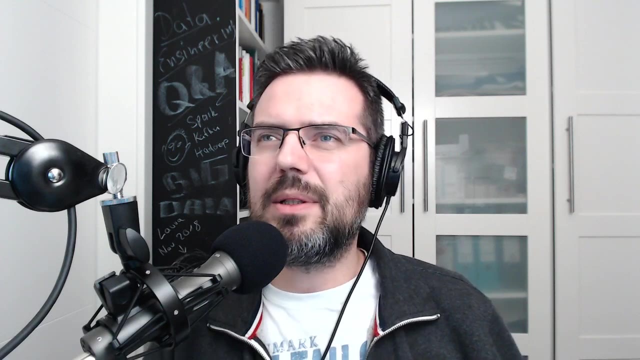 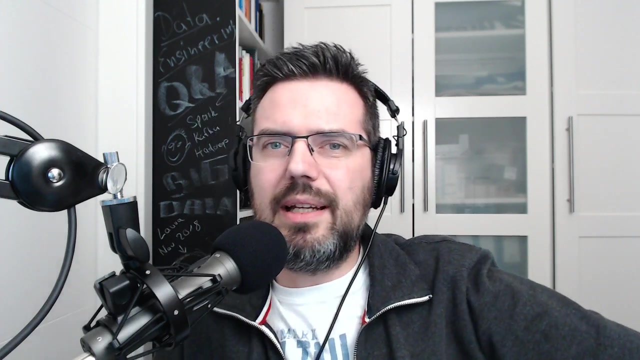 10 000, 100 000, and then the counter is updated and everything is super, super clear and you can do this on on multiple servers and everything is everything is um is done, yeah, uh, one question here is: can we before perform etl with hbase um? you can, basically you can use that like a, like a. 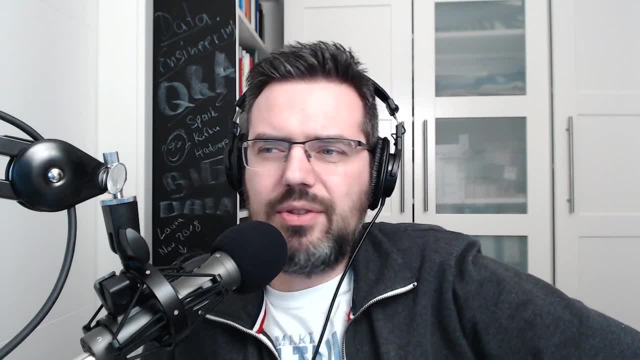 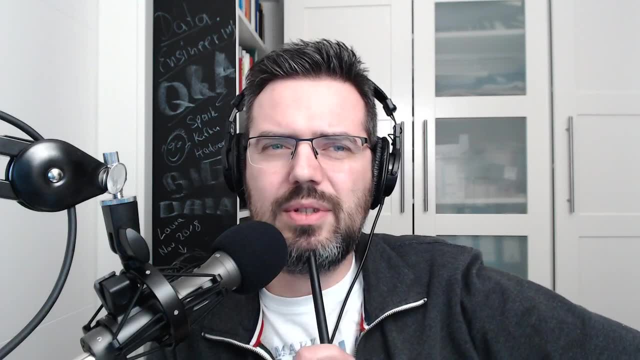 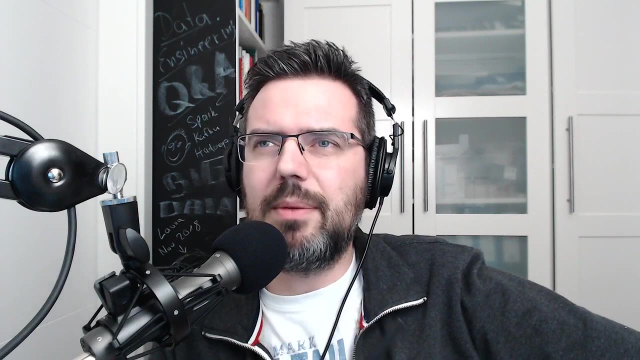 normal database, um, you can, just it's called here, it's not calling select statements. what you can do here is you, you can, you can do this on multiple servers and everything is, everything is um is done. do scans of rows? so you, uh, yeah, scans of uh, is that rows or tables? so you, basically, you can do. 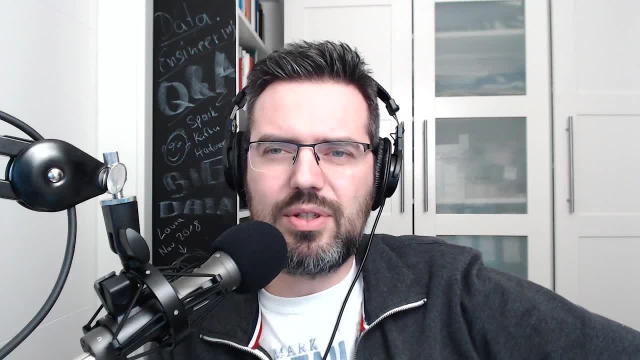 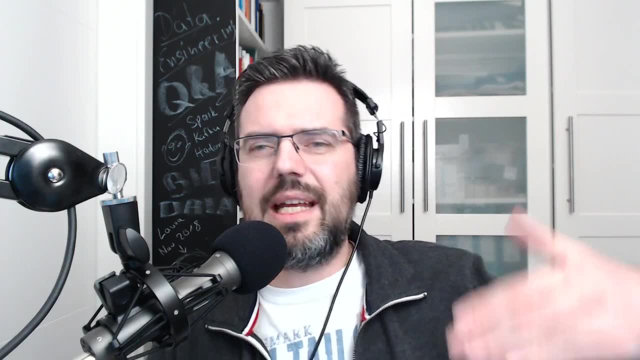 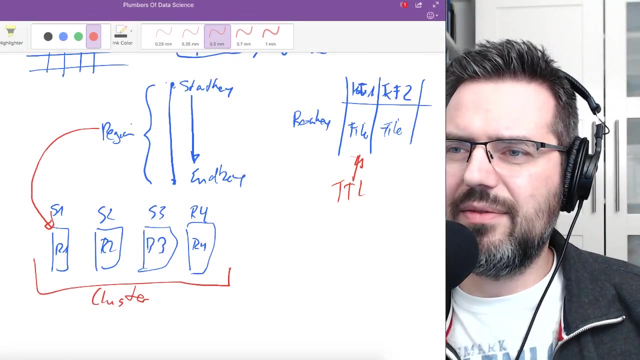 scans. so where you say, all right, i want to have the, the first row, and this is my last row that i that i need, and you can also do some some filter statements, and then you're getting then the, the, what the system is doing, it's, it's, it's searching for the regions that you have and it's basically 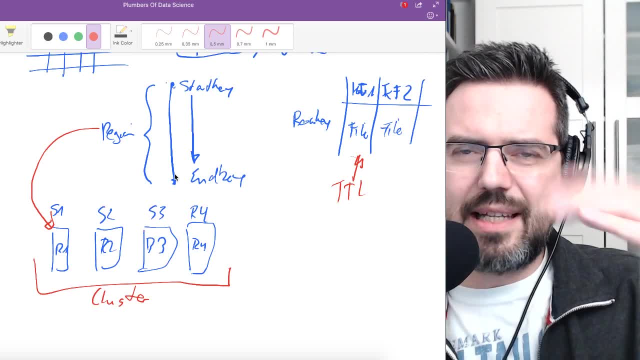 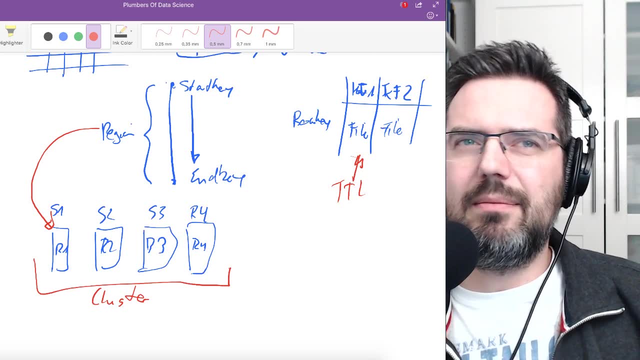 running through the regions and it's basically running through the regions and it's basically filtering and scanning and filtering out the the things you, you don't need, and then it's going to send it back to you, um, in a, let's say, etl manner: very, very simple and very effective. 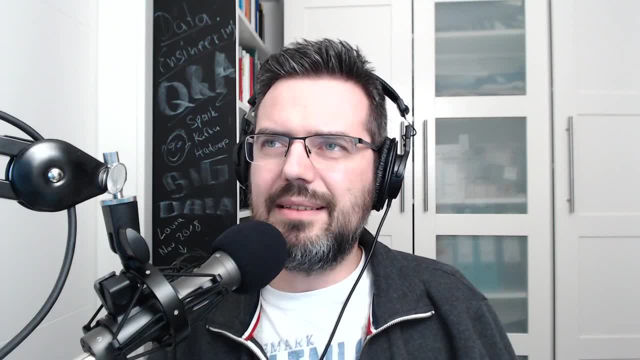 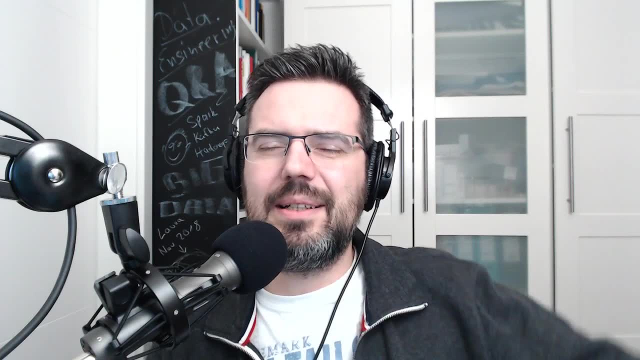 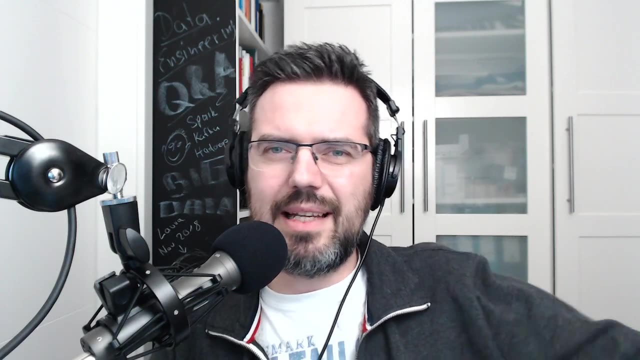 it can can take some time, uh, at some point. if you're doing a, a if the more complex it gets, um, the more time it takes, but it usually it's. it's not going to take a lot of time to do it. it's very, very quick with scans because, as i said, what it's doing it's there is no index, it's just. 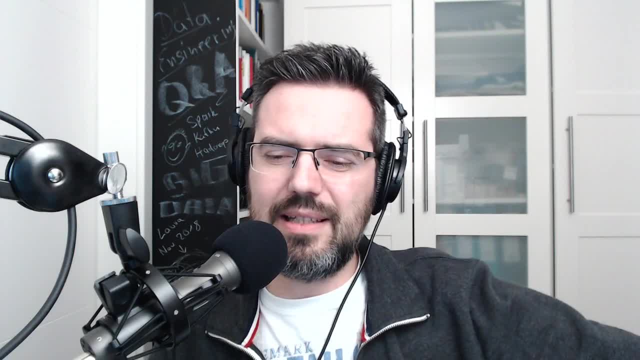 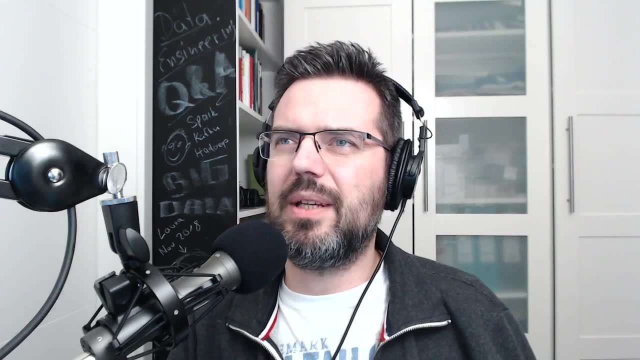 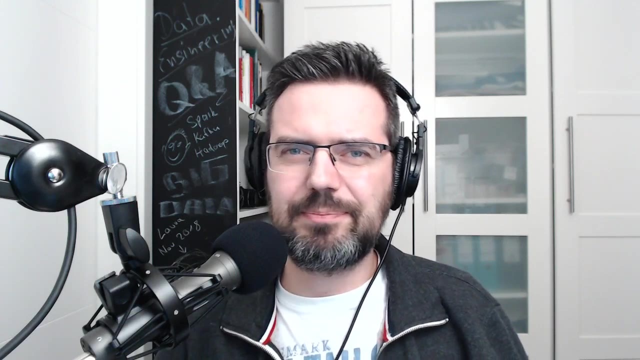 running over the region and filtering everything out that doesn't need, that you don't need, and it's because you know the, the start and end point. um, you can do very, very easily etl, like, like or like, select statements. um, one thing, what was that? i had another. 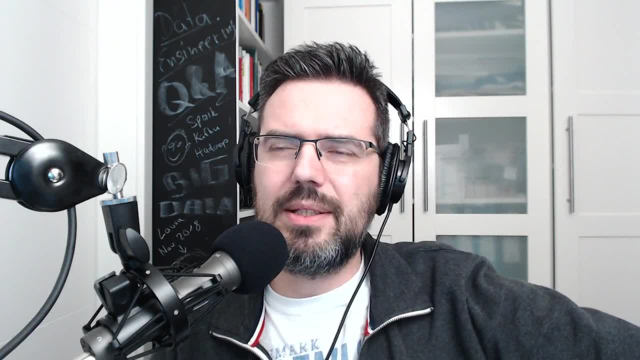 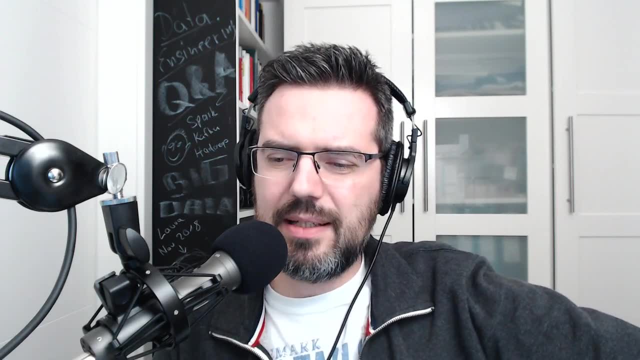 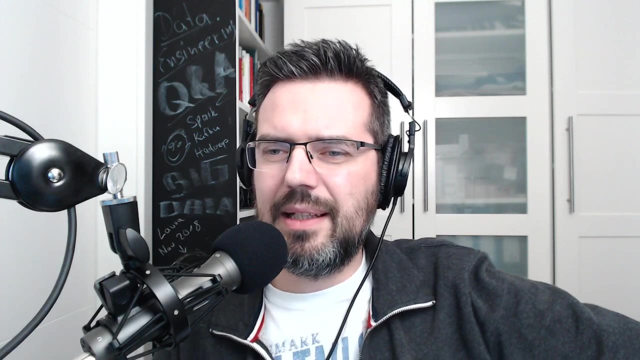 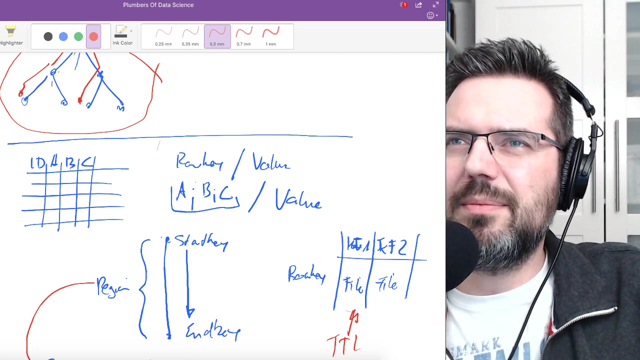 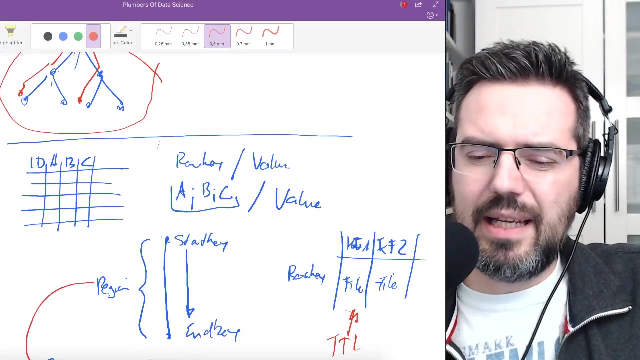 thing here, um, related to the etl question, as one thing that that that people are also do is what you can do. let me go back um the is that is that. uh, is that a a sufficient answer or should i elaborate a bit more? or? um, what you can also do is if you're, if you have something in hbase. 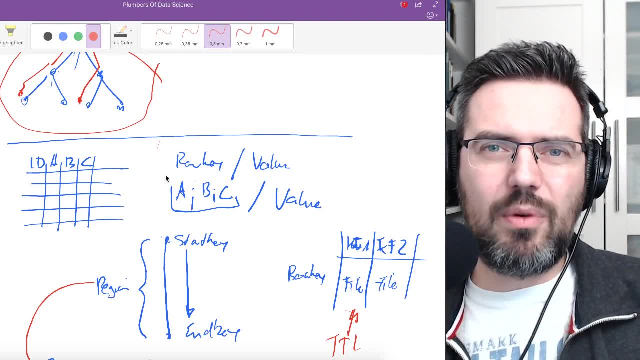 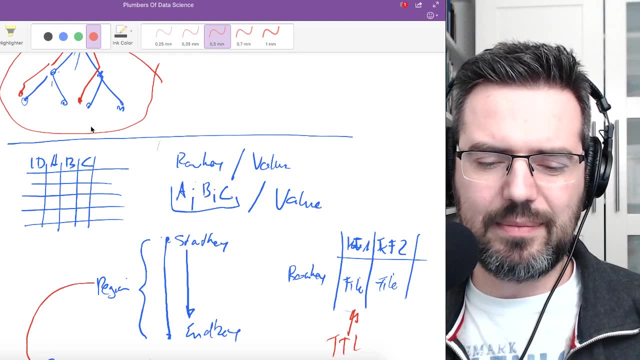 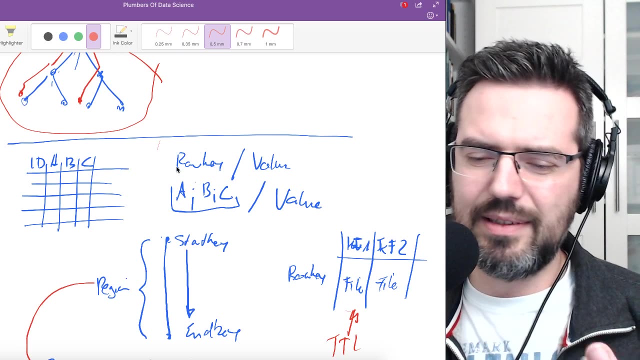 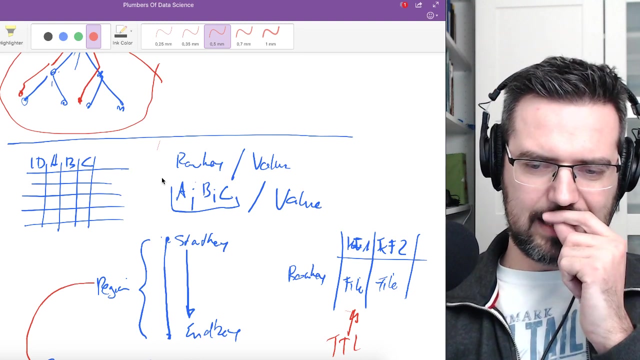 you can basically get it back into a table format, and how this works is, for instance, with something like um- hive- within hbase, you have a, a system that, or a hive, you can create a hive table, and the idea with hive tables is that is that you know the, you know the composite key. 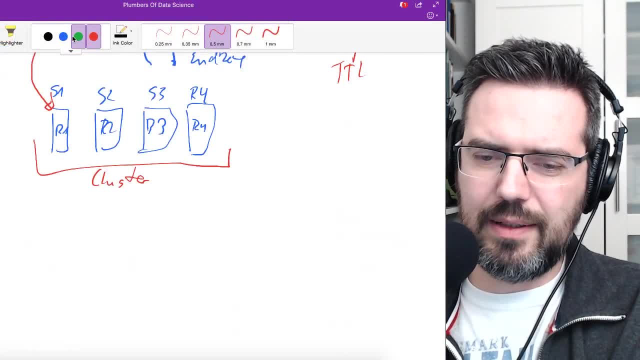 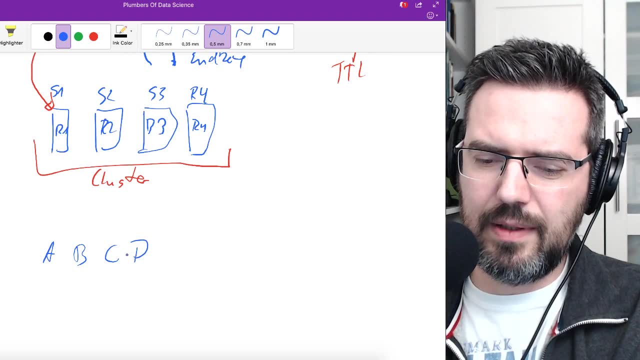 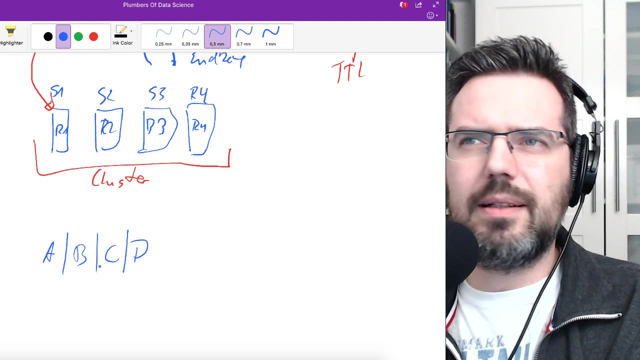 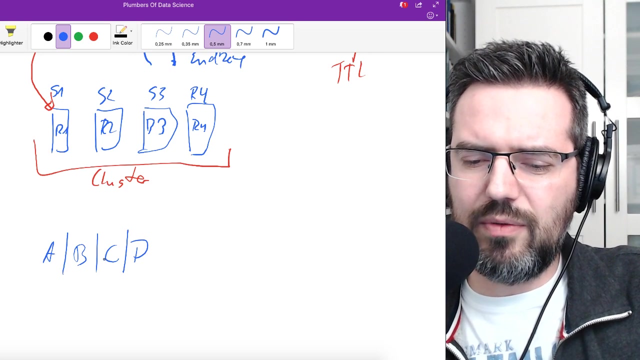 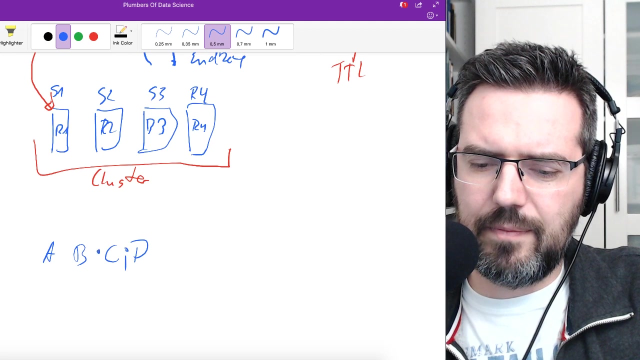 just need to draw this here. new, um, you have your composite key a, b, c, d, with something with a, with a man. how is that called delete key delimiter or something? so what? you, you know this. you, you know the formula. let's, let's stay with. see my, see my columns here. okay, and you know this. and with a. 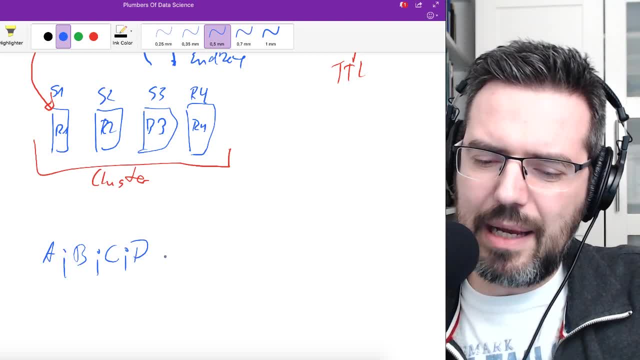 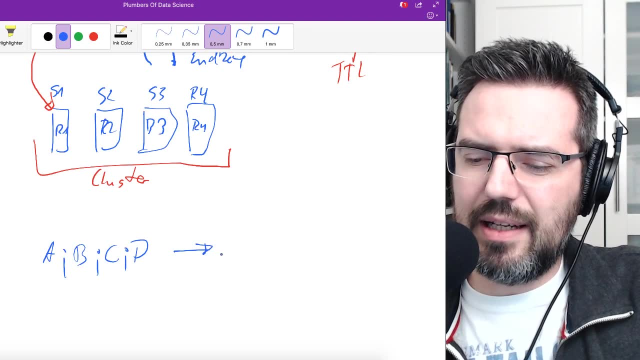 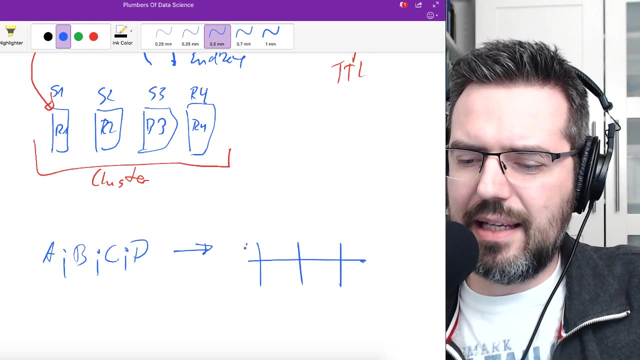 with a hive table, you can basically get this back out, and you can. you can say or, or- the delimiter here is semicolon, and then you can. you can define the columns again, and then what you're going to end up with again is something like a sequel. 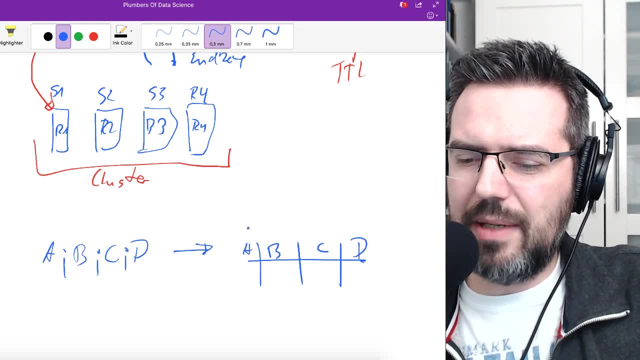 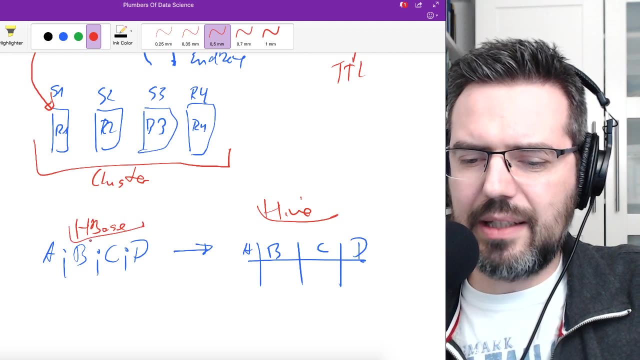 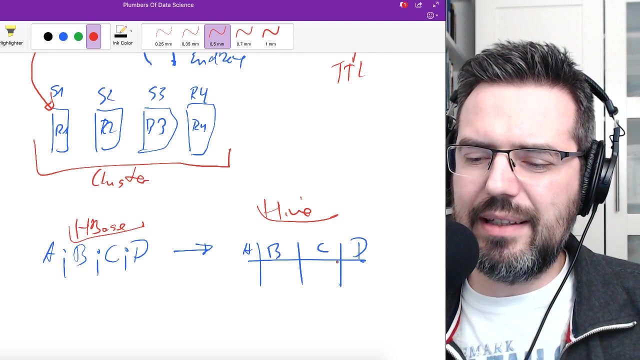 table ABCD and with column names. so you can give this thing a real in and I'm just let's pass, so you can go from H base to hive, because you know the format of the composite key. you can go back into a, into a table format, and then you can use again if you have something. 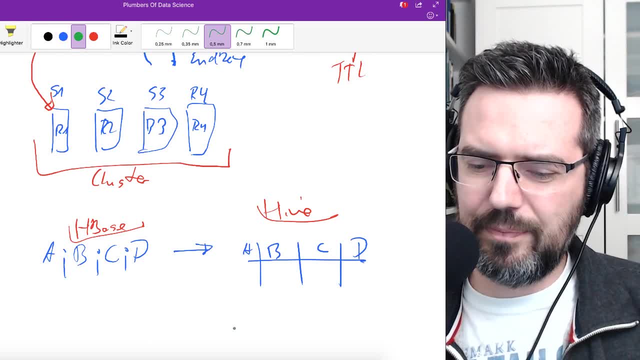 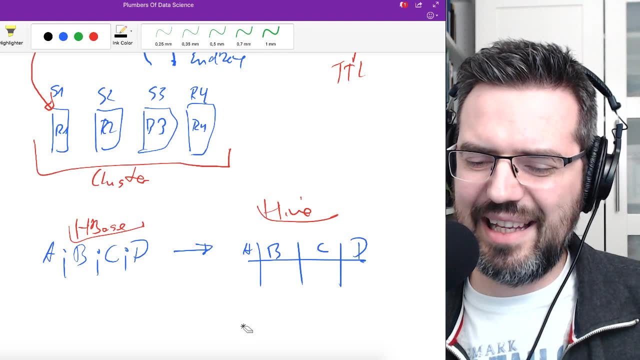 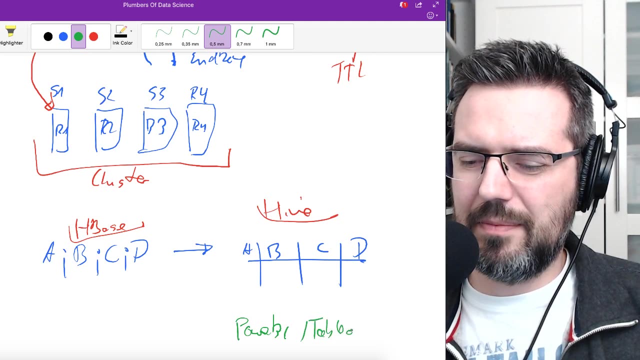 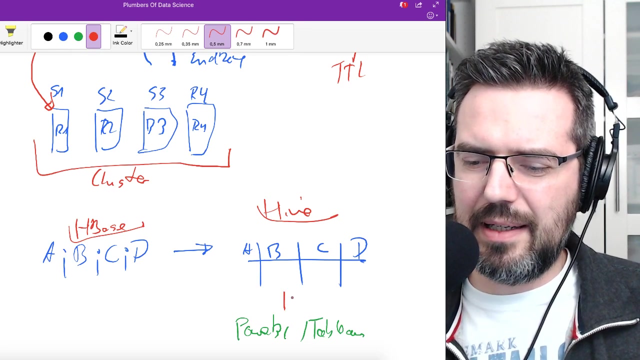 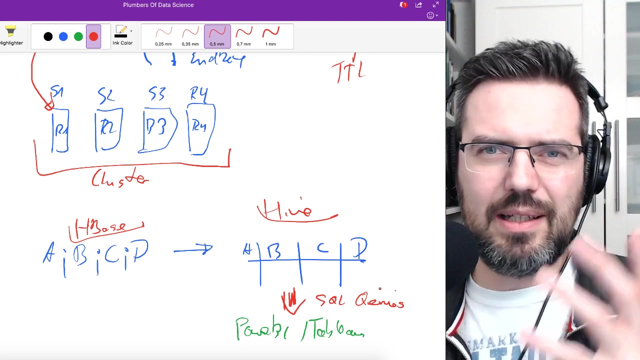 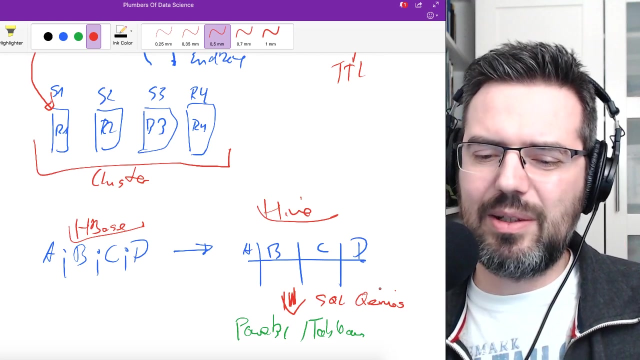 like like power bi or tableau, something like power bi or tableau. you can go and do sequel queries then again on this data in the. what happens in the background if you do this is that if you're running hive and you're doing you, you're doing a sequel selects on top of, on top of a H base table. in the background it's running map. 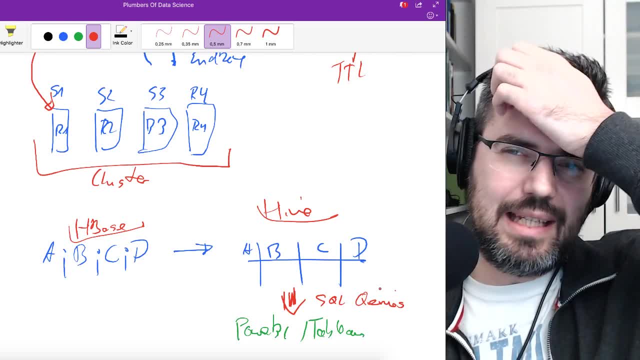 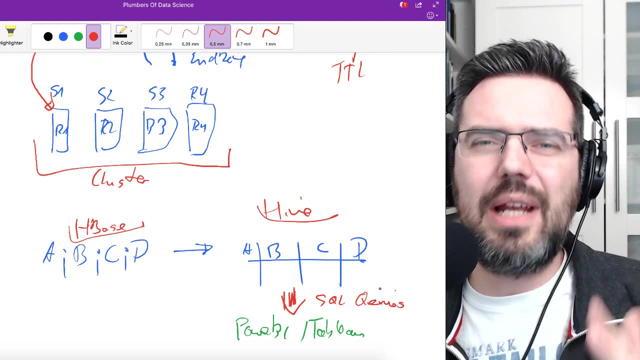 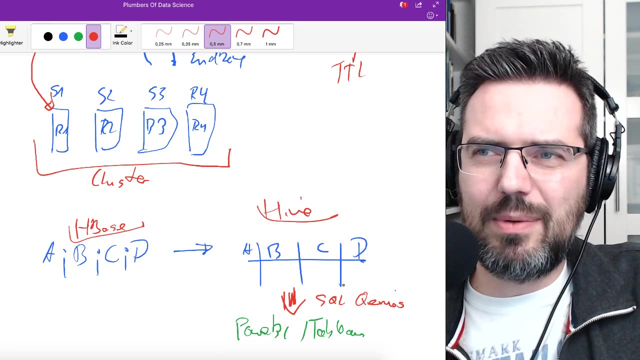 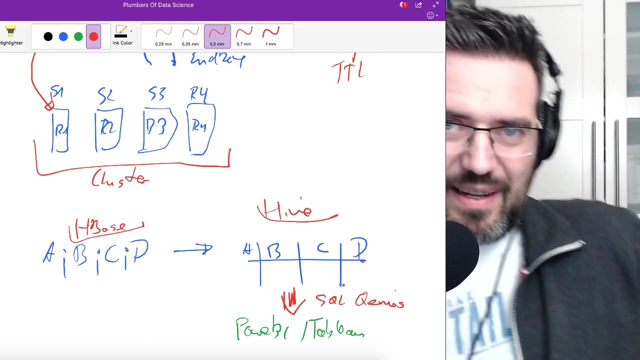 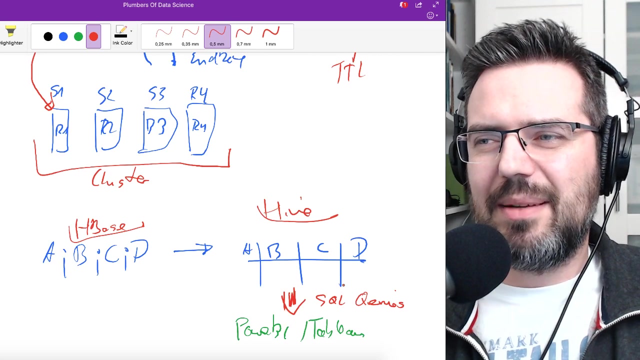 produce jobs and basically giving you the data that fits to your queries. So it's simulating SQL queries. The thing is that those queries take some time because, as usual, MapReduce is not super fast And yeah, so it's taking usually some time to get data out of it. 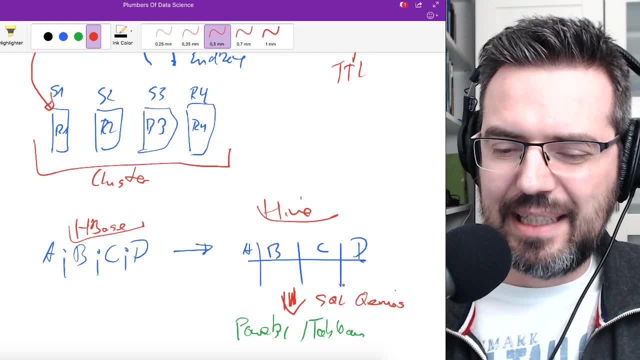 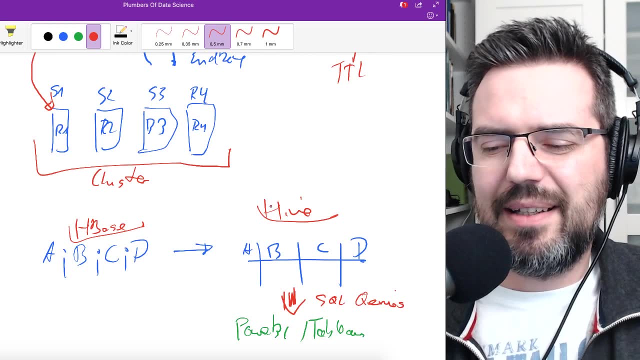 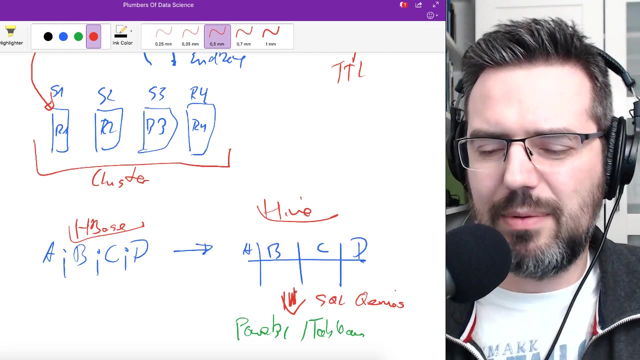 especially if it's a lot of data, And people are sometimes not expecting this, if they are using Hive on top of HBase, because for the user it looks like that you're using SQL, but in the background it's running MapReduce. 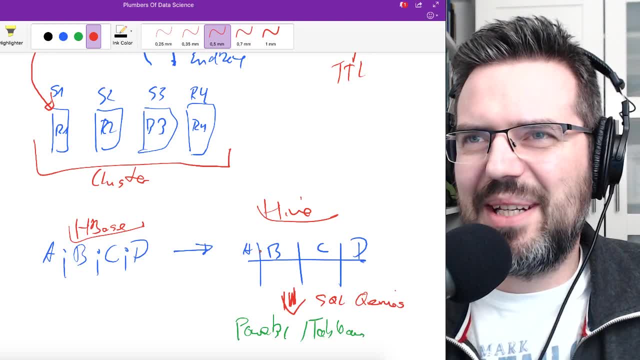 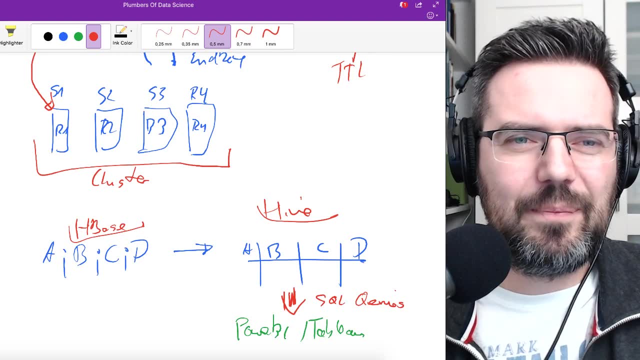 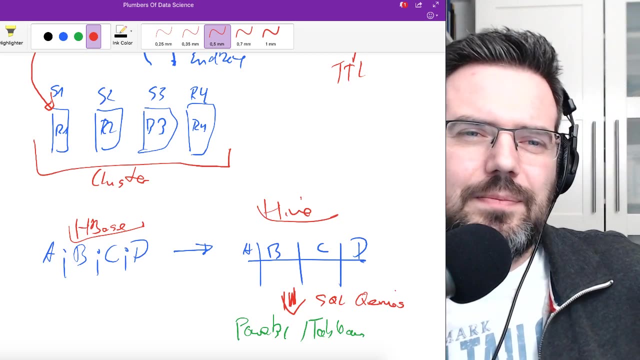 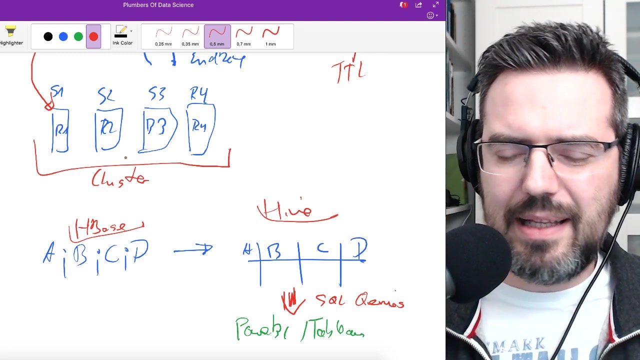 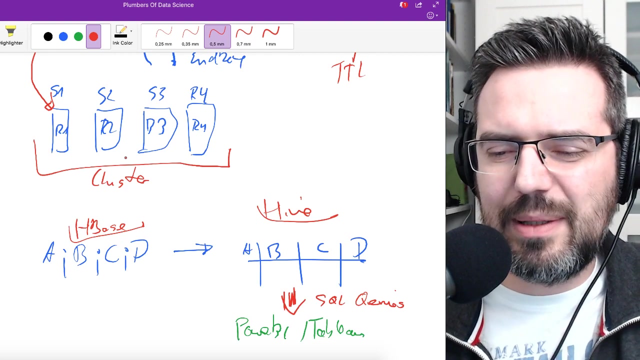 And- And this is a bit of an ancient technology and not always very preferable- Okay, so Exactly. So, Yeah, this is basically. that's basically it, with HBase as a NoSQL SQL. So NoSQL, it's a key value store. 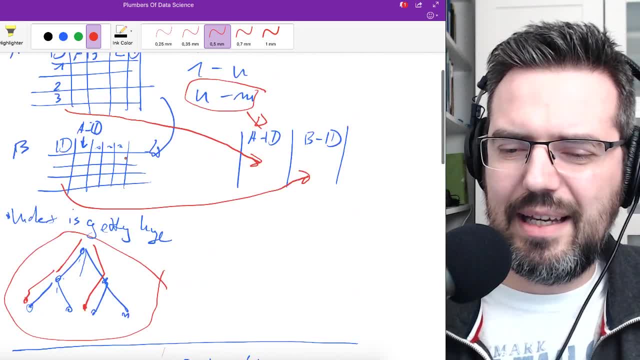 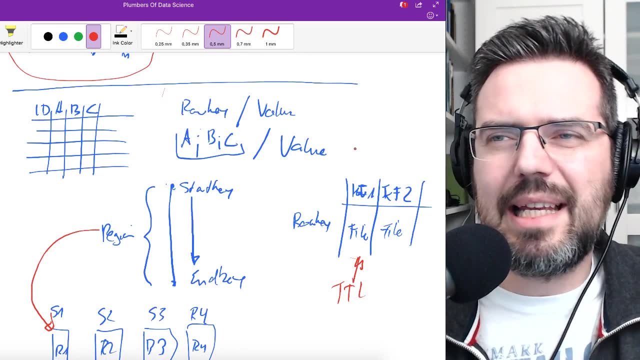 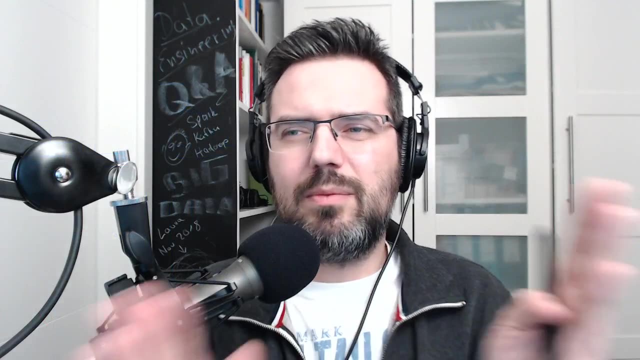 You can, you do the, you have a lot of keys and you are, you are putting in your data and it's it's not about it's not about width. It's not about width, like with SQL database, where you're doing a lot of columns that you need to predefine. 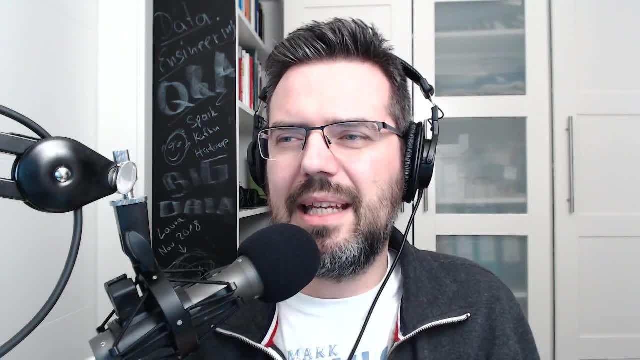 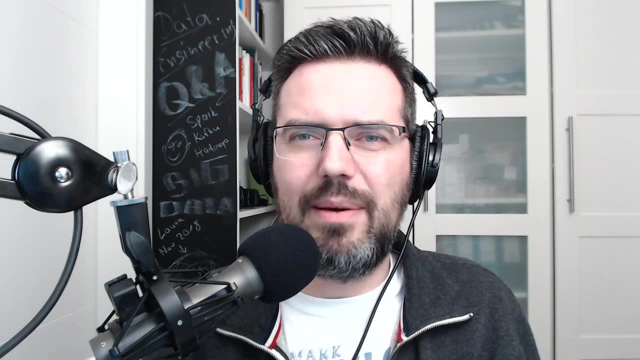 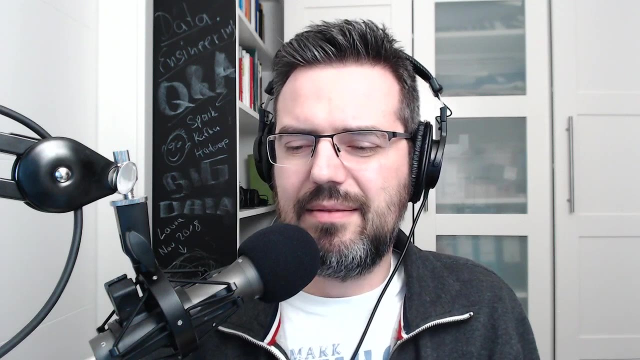 You're doing rows and you're you're putting everything in and you can also, if you want, you can, create column families on the fly and put data into column families on the fly, And it's very, very flexible and also super fast. 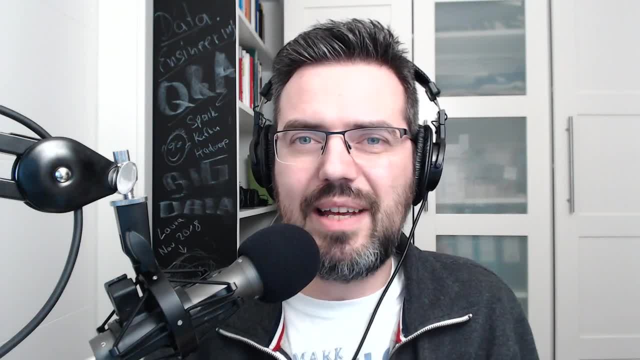 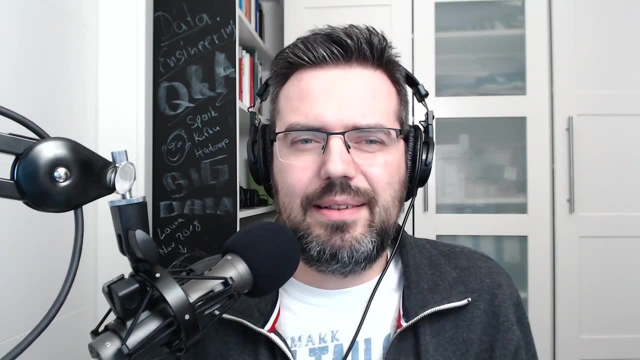 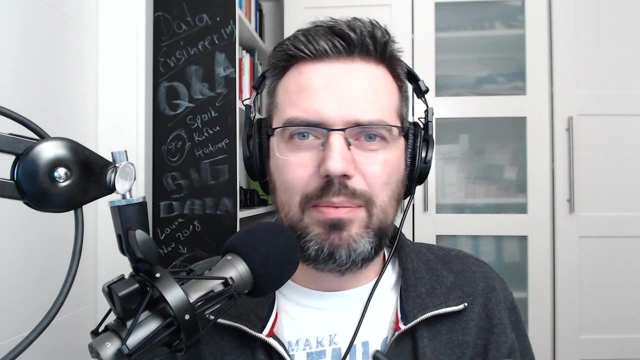 And because it's it's based on HDFS, on running on HDFS, you have the. you have the upside that that you can is that you can use the data. They are very, very good for for parallel processing, because everything, as I said, 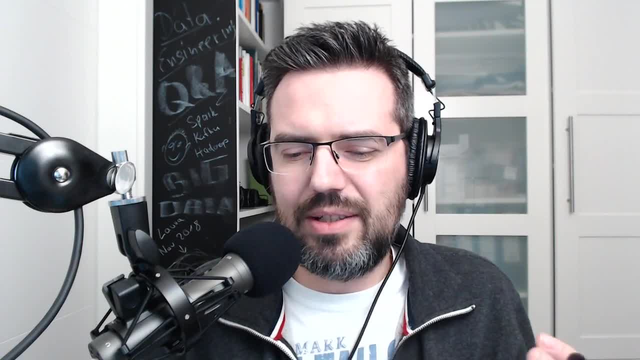 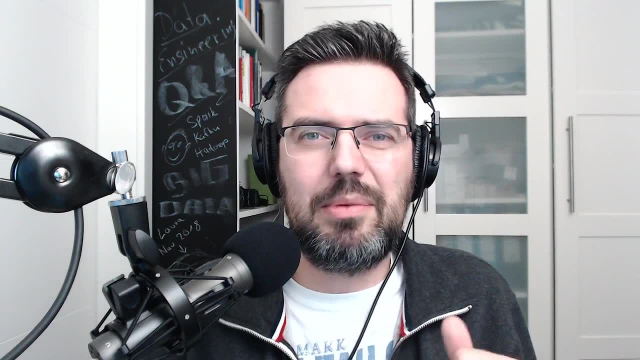 everything is parallelized. You have the regions, and the regions are distributed over the servers of the cluster And then if you're running a Spark job or a or a MapReduce- if you're still using MapReduce job- then you can parallelize this super easy. 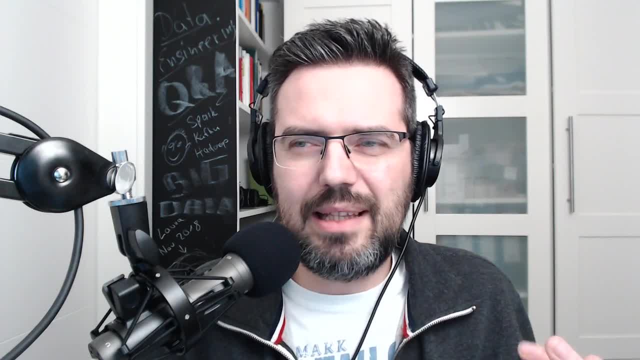 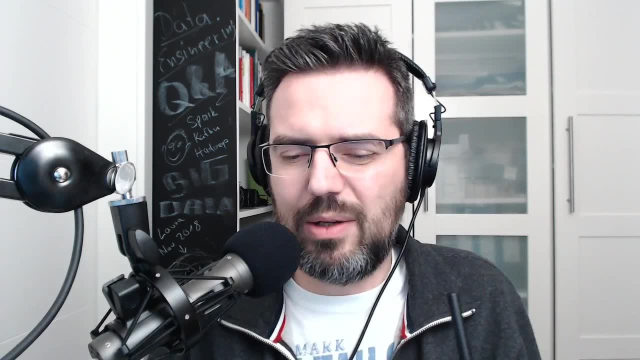 And also those regions. they are bigger than the block size. So within the regions you have a lot, of, a lot, a lot of distribution over the over the whole cluster. Ah, I see I have forgotten to show the one note again. 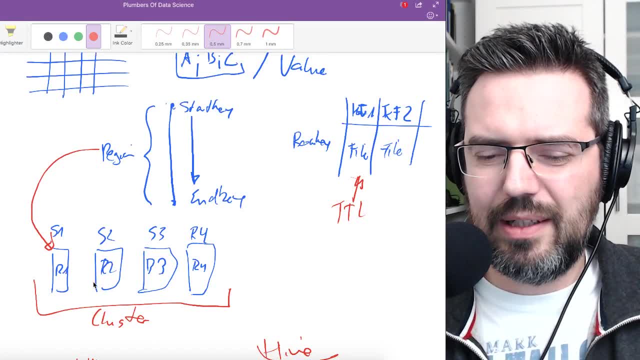 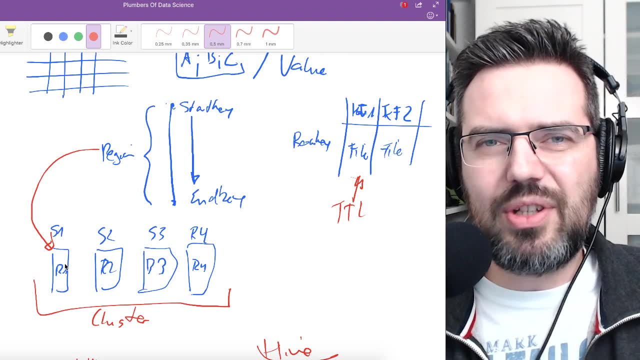 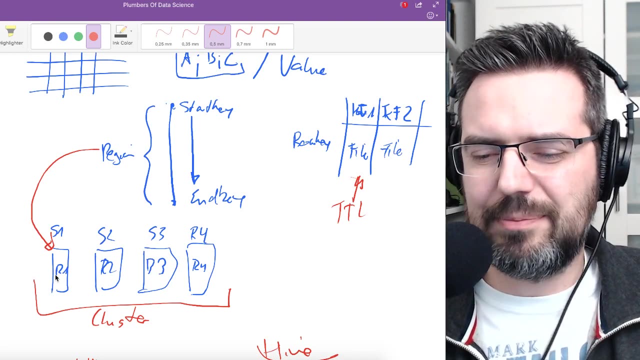 So basically, here you're, this, this one region. this might not only in HDFS- be stored on that server, because the the file below that is, can be stored on multiple servers as well. Yeah, So have in mind with HBase. 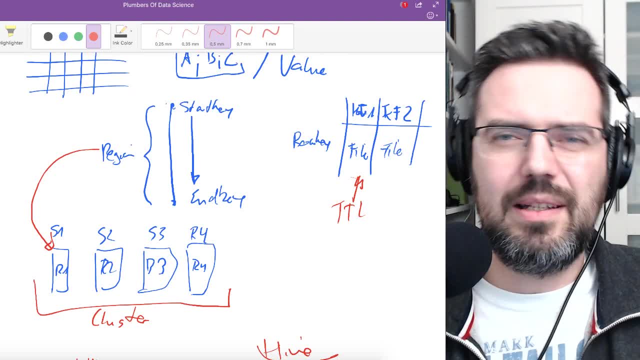 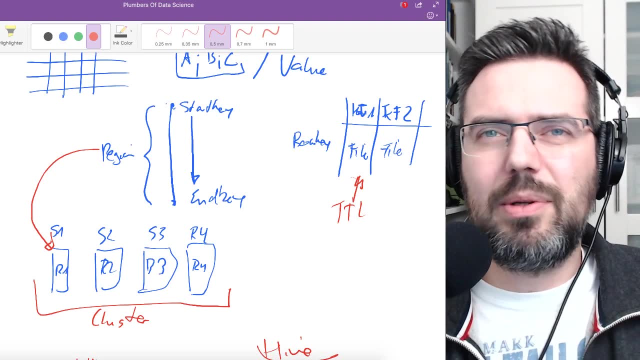 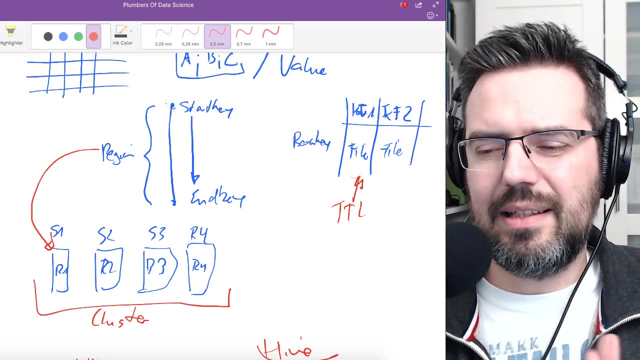 have in mind that you need to work on con, on composite keys. You need to figure out the, the, the, the distribution or the, the, the ups and downsides of the of each key type or key design that you're maybe getting region hotspotting. 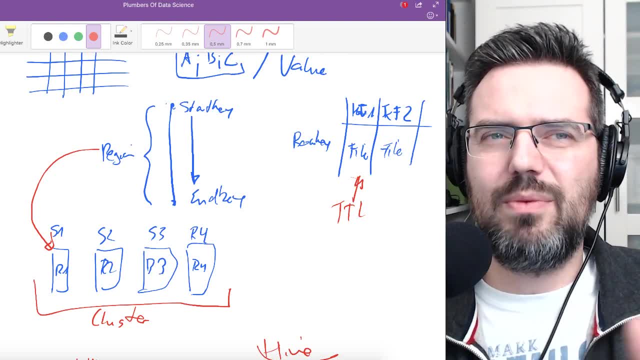 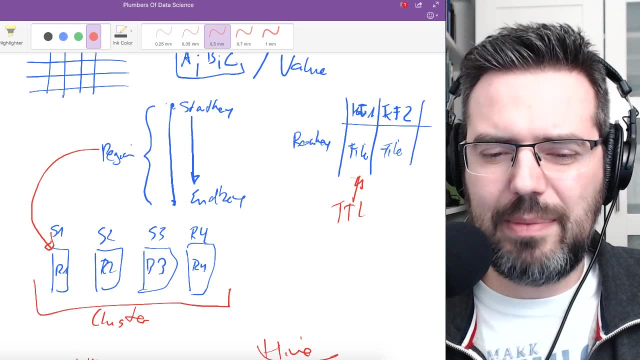 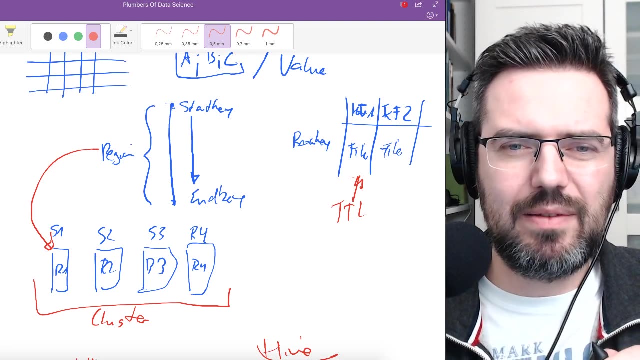 when you're writing, or you're getting too much hotspotting on a region, when you, when you read, and yeah, then you know, then you're, you're, basically I would say you're quite good, This is, this is one of the things. 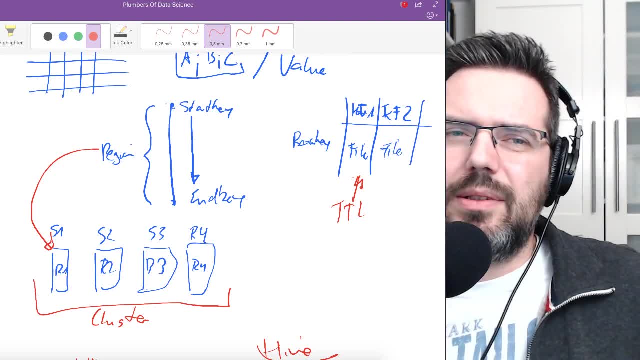 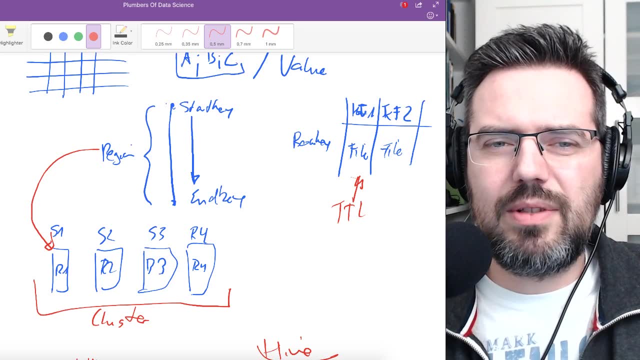 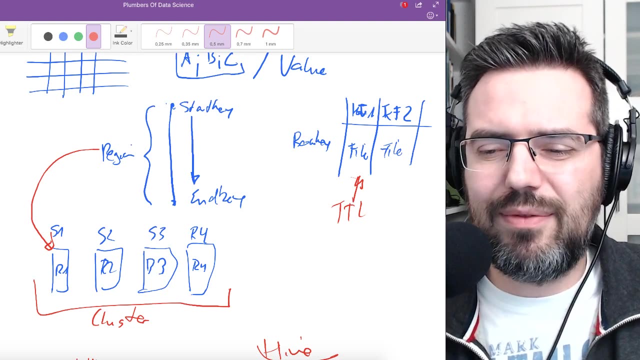 Yeah, What people are. you can use, for instance, you can use HBase in in in different ways. You can use HBase for storing the data permanently, or you can also use the data for storing it, Like with the. 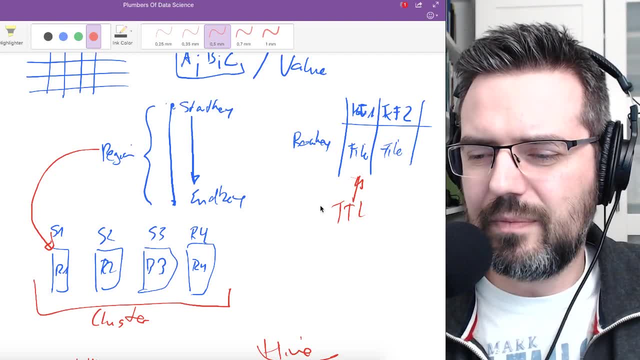 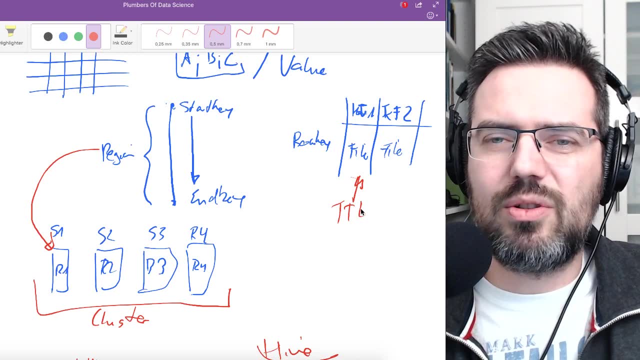 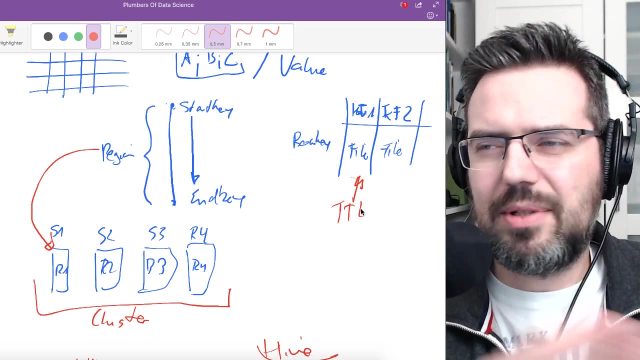 as I said with the TTL, with the time to live of column families, you can store it as a temporary storage. So people are using it, for instance, as storage of data for user interfaces. If you have a, let's say you have some time series data and 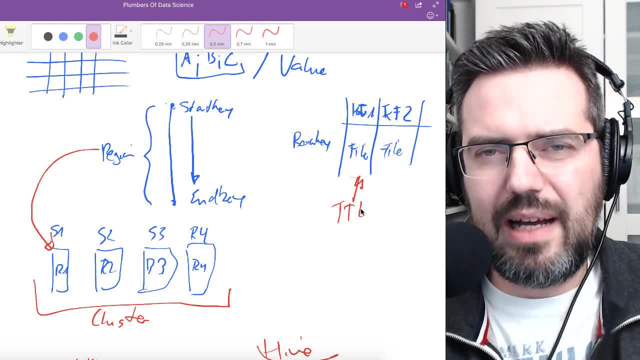 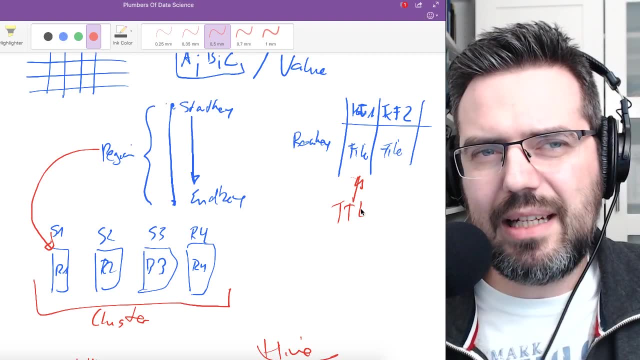 and it's a lot, and you just want to have three or four or five or six days of of temporal storage And you want people to have access to that data. You can use HBase for that And I have seen. 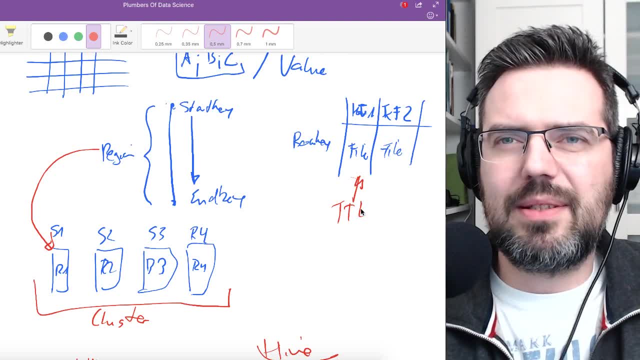 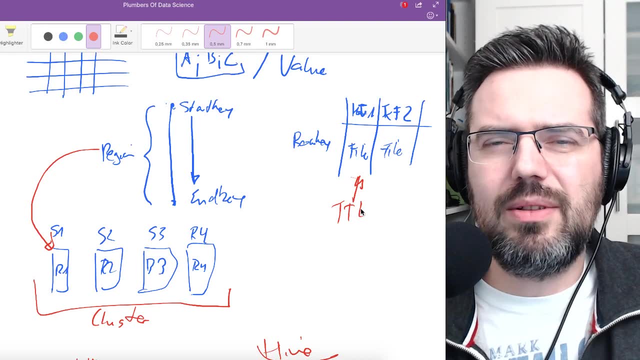 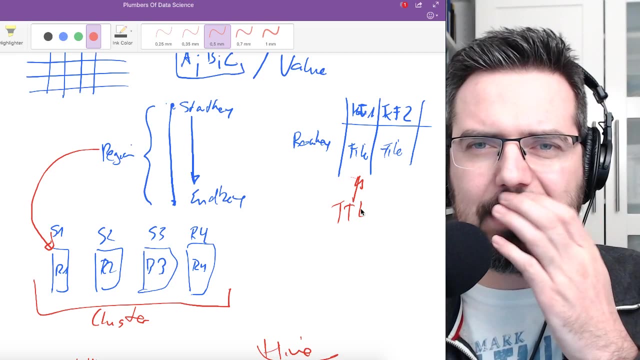 see many use cases, examples on the internet where people are doing this. They some also use Cassandra, which is a bit of a different key value store database, or Cassandra is more. I think it's more called a, something like a linked list or something. 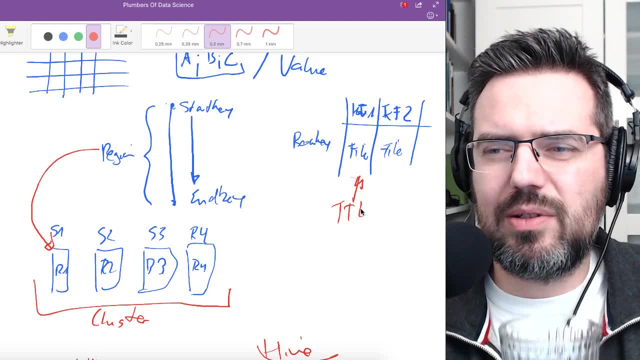 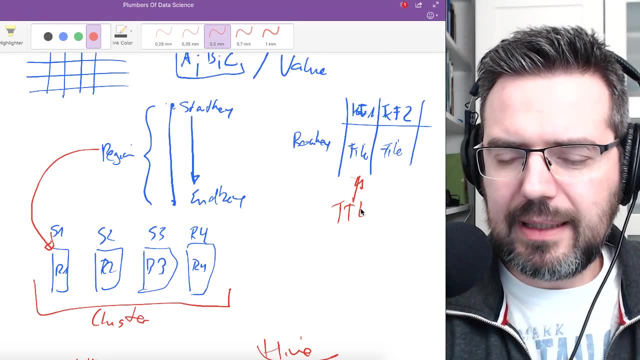 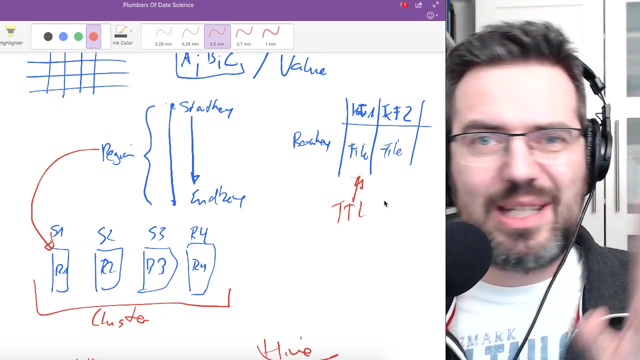 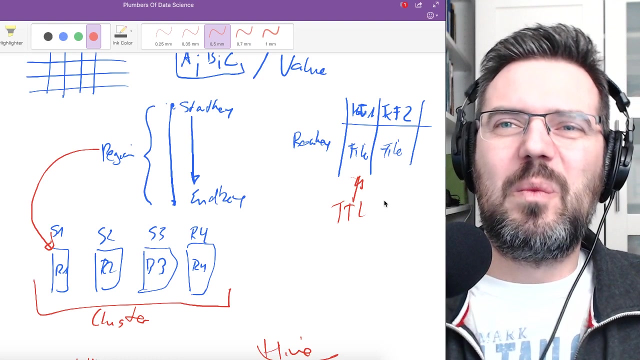 Yeah, But there's also super, super interesting And yeah, One thing: So this all sounds very, very good, Very, it's super cool. And where is the downside with HBase? One thing: with HBase: one downside is the amount of data you're storing. 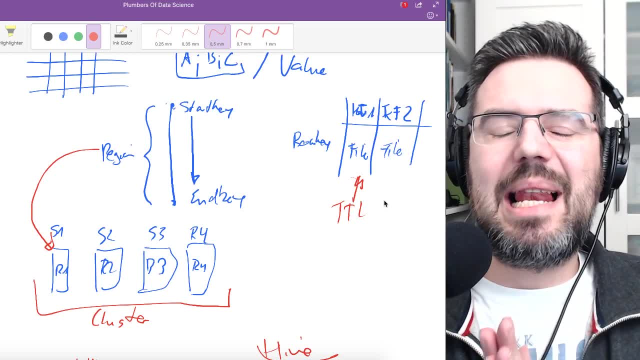 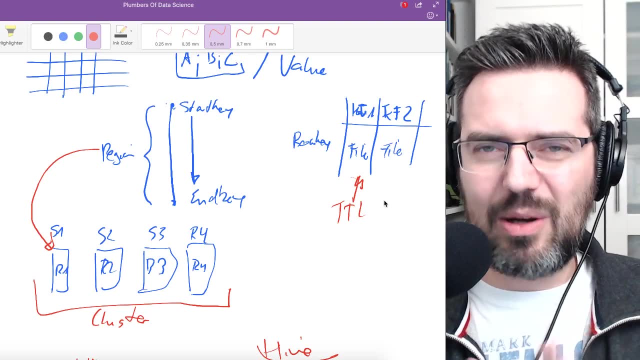 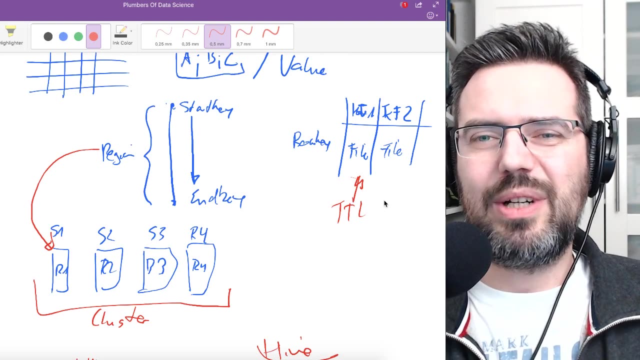 Yeah, The amount of data you're storing is a lot bigger than with a SQL database, because with every value that you're writing, you need to store the composite key and you don't only. you don't only store the composite key, You're also storing the 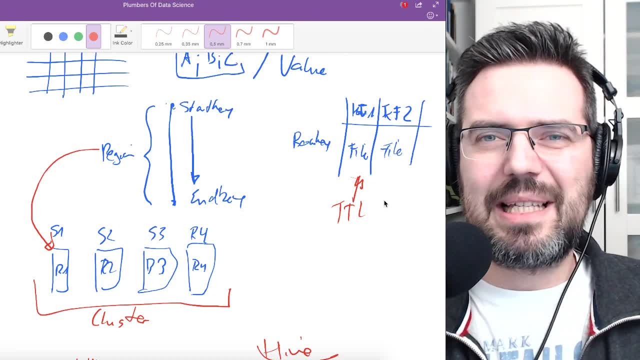 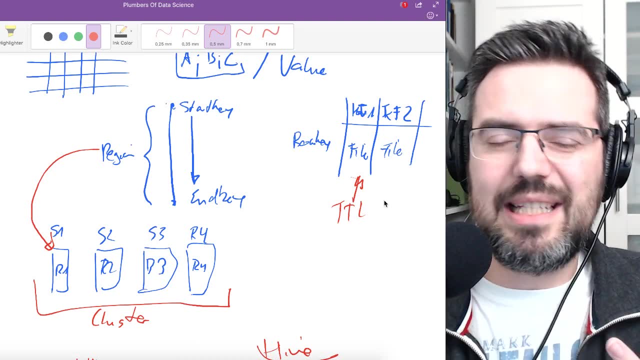 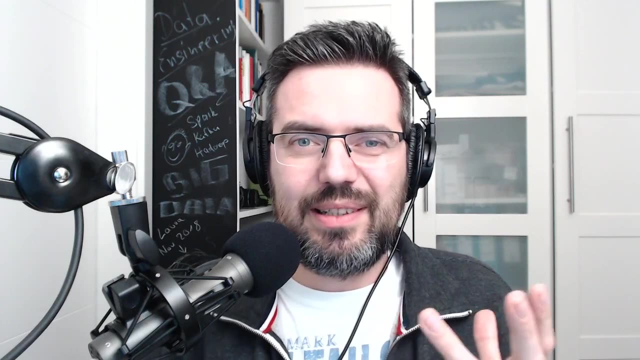 the column family name with it, and so on. So it's you're. you're getting a multiple factors of, of, of storage needs, Which needs to actually to actually store. So it's, it's, it's, it's big. 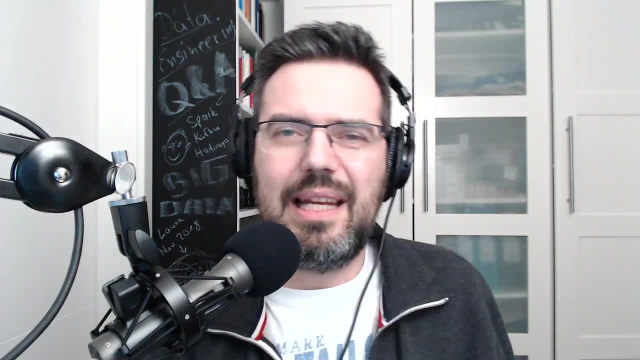 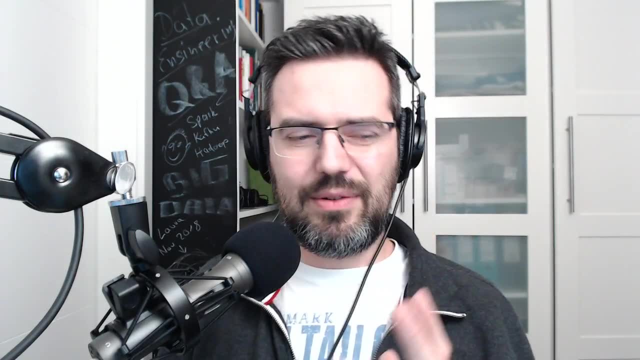 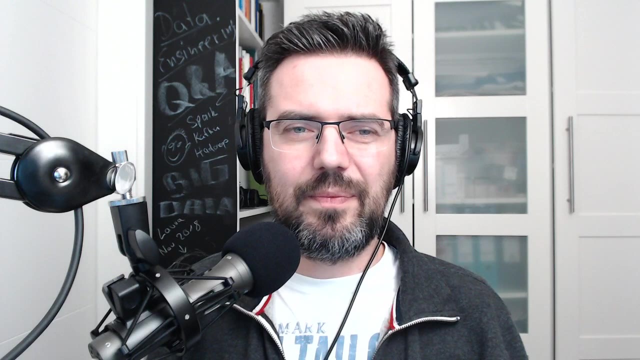 it's getting big. So what? what many people do is they offload then data back into H, something like HDFS, and have only the the super necessary data within HBase. Yeah, So the one, one question that that I had on LinkedIn was the advantage. 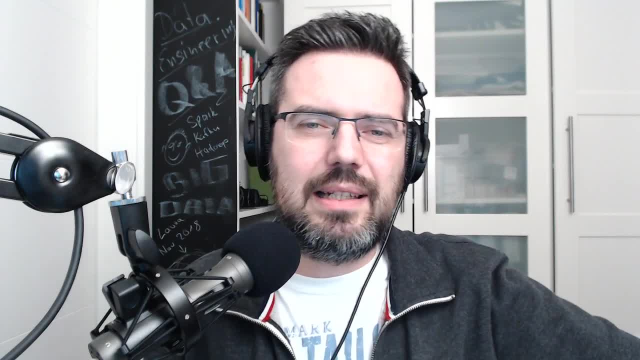 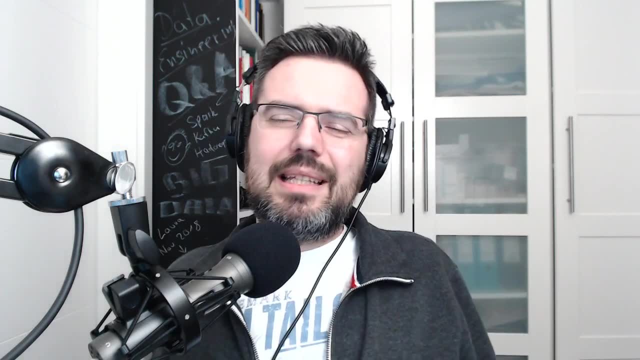 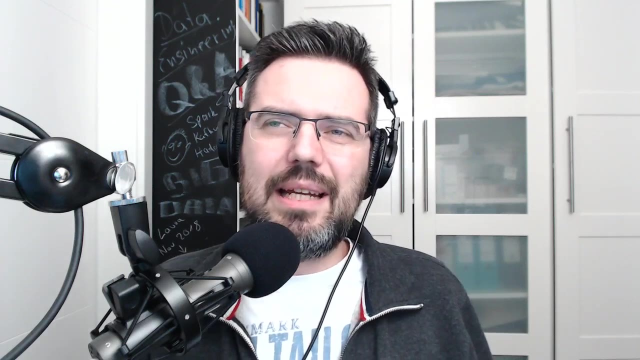 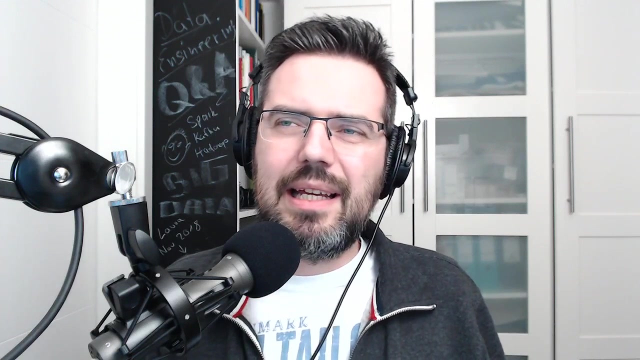 what are the advantages of streaming data and, yeah, of streaming data with HBase? This is a. I wasn't a hundred percent sure what what he meant with the advantages of streaming data and live data within HBase. Of course you have live data within HBase and 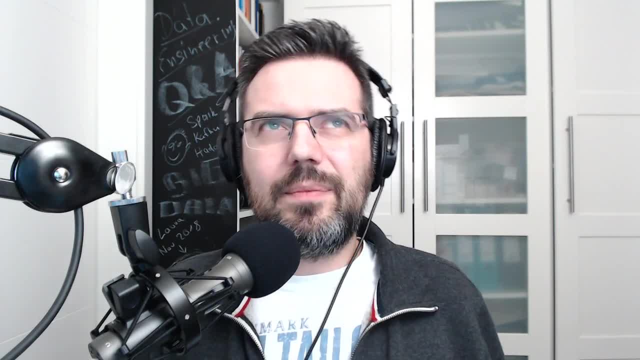 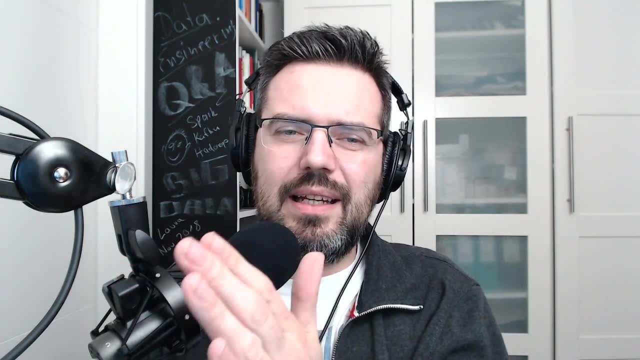 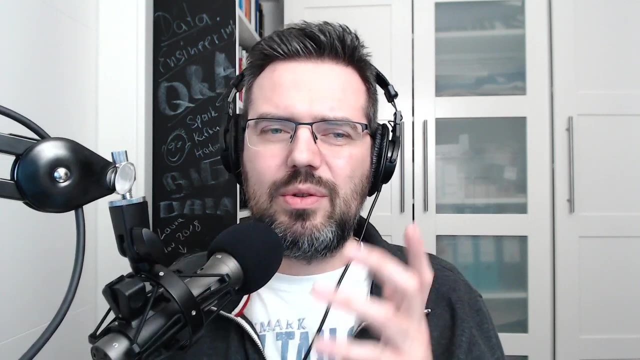 but, um, it's, if you're, if you're thinking about streaming stream processing, what you're doing usually is you're doing something like: uh, you have a message queue and then then analytics and then the storage. So the the actual 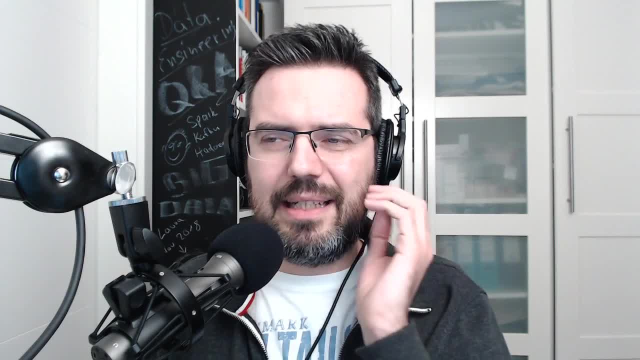 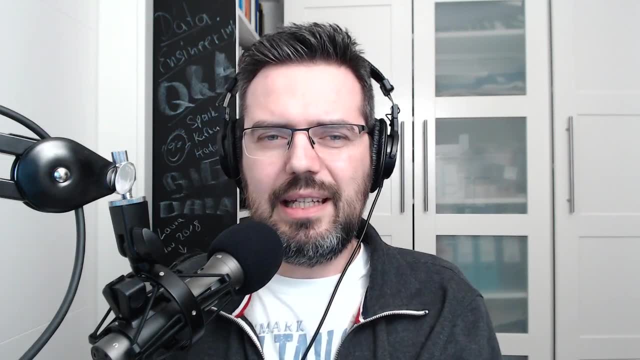 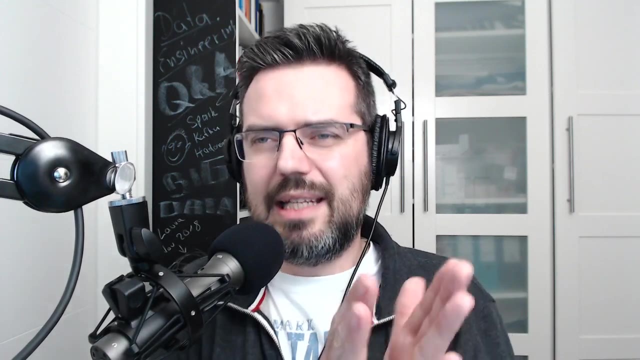 the actual database is coming after the analytics and um. so it's. it's not that the data is coming in, getting stored in the, in the database, And then analyzed and then presented. somehow. It's the other way around that you're getting it. 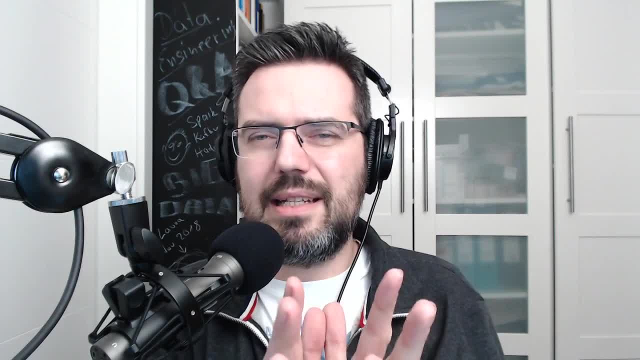 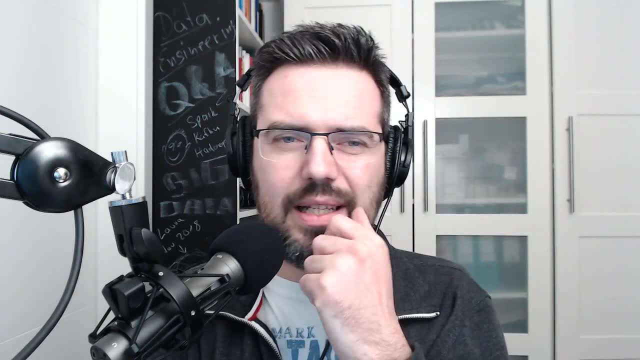 you're analyzing it, getting it, for instance, with Kafka, you're analyzing it with Spark, and then you're you're filling or you're putting the the results into into your, into your HBase database or into HDFS. 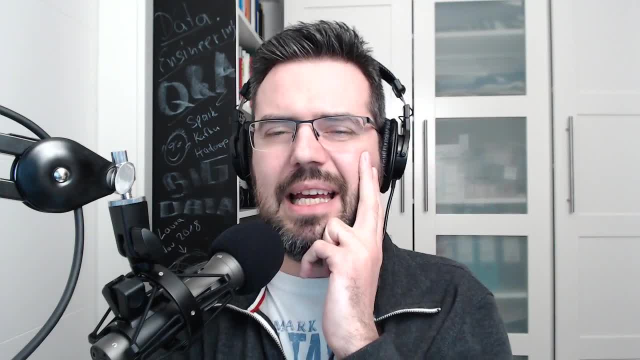 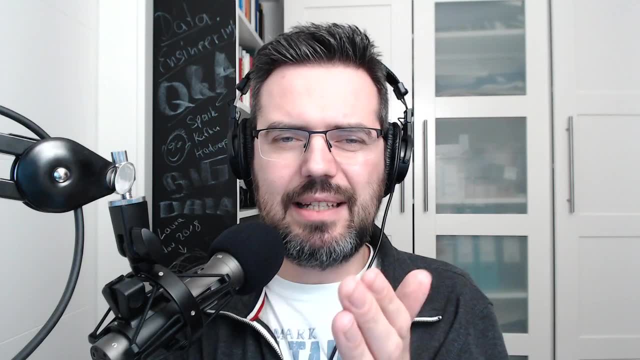 So you, you can, you can do multiple things, Um, one one, really. one upside with with HBase is the good scaling. So you can if you have a hundred servers and you have a good, a good composite key design. 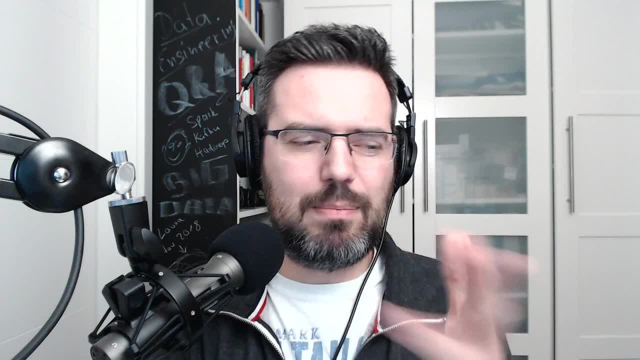 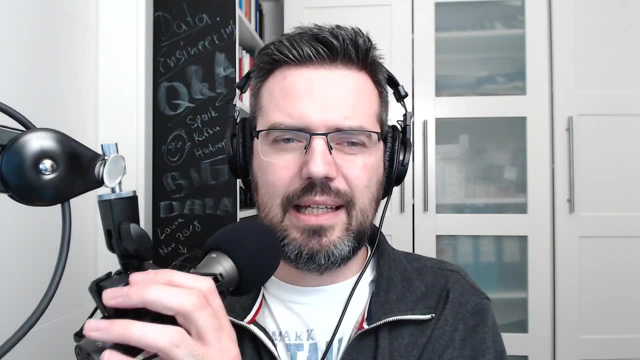 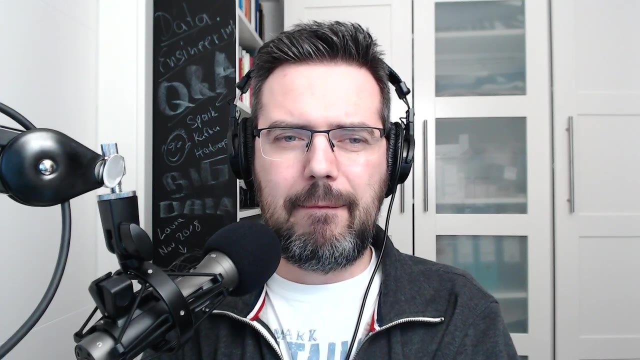 and then your data is just: it's blowing in, it's, it's crazy, And you can also read it very, very, very, very fast, very, very quick and very paralyzed. Um yeah, Real-time analytics, Yeah. 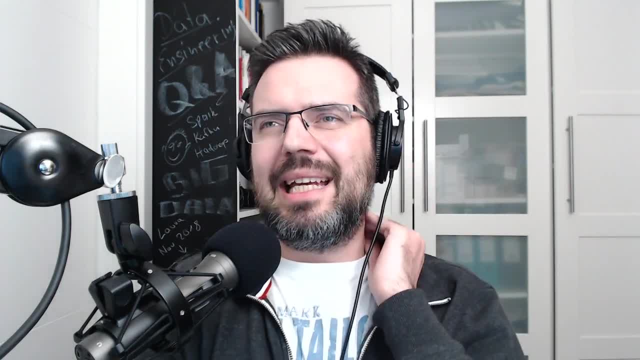 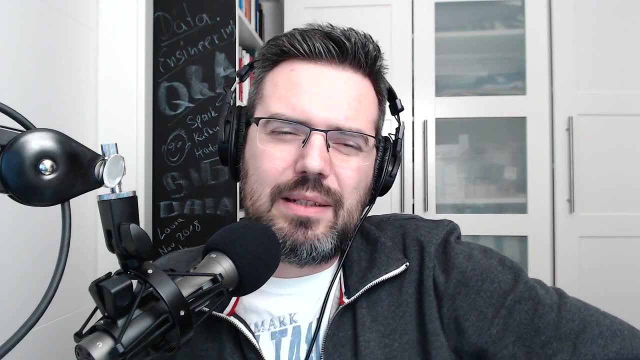 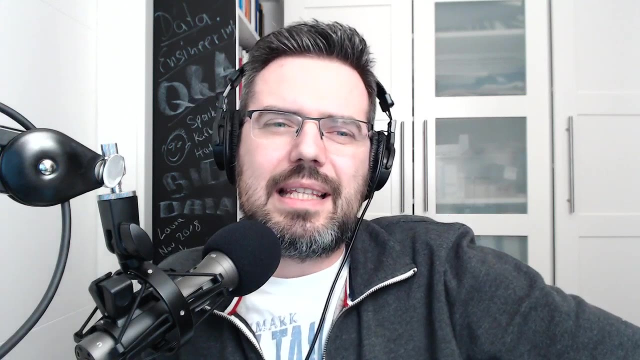 How good is it for Jason or XML data? There was another question. Um, I'm not a hundred percent sure. I haven't worked with- uh, with Jason and XML data within HBase. Um, I think this is it's. 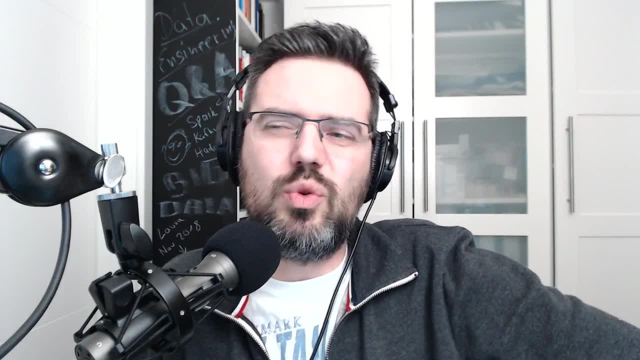 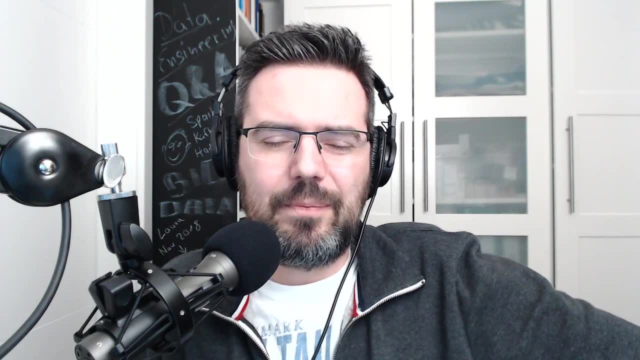 this is again something like it depends on what you're actually doing with the, with your data, and how you're. how do you query it? Because, um, if you want to get to a row, you need to know, you need to do the composite key design. 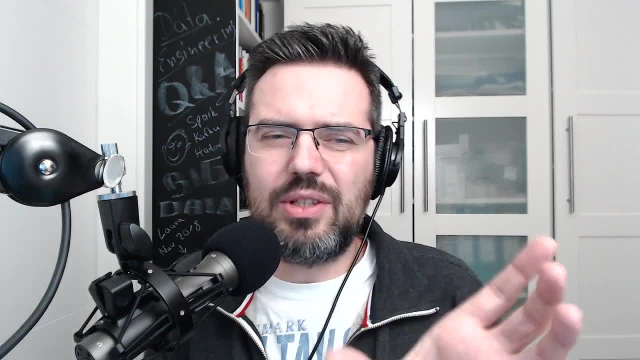 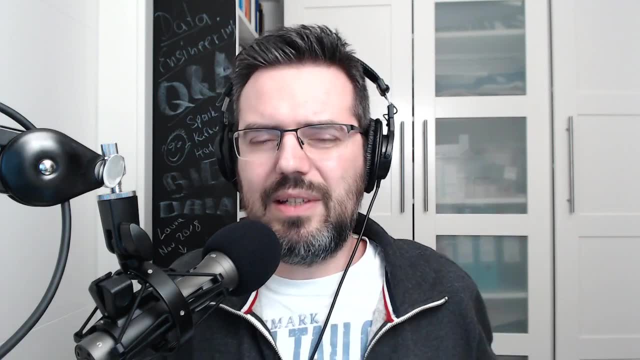 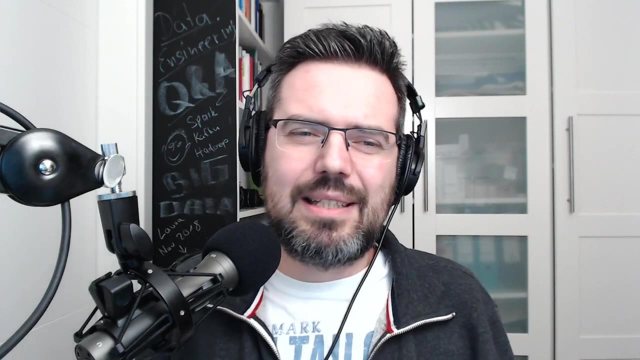 You need to somehow uh extract the data from the Jason, the the the necessary data from the Jason, and put it into the, the key of the of each row, and have that basically scannable for getting data out, And so. 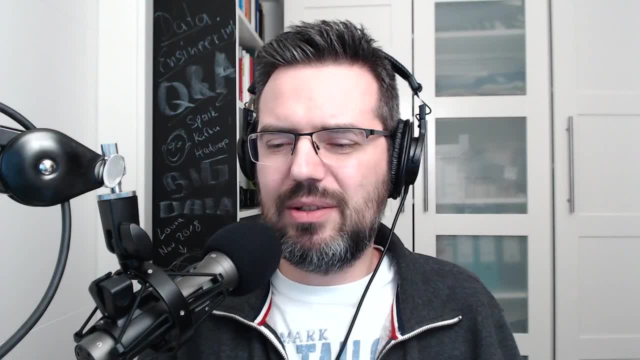 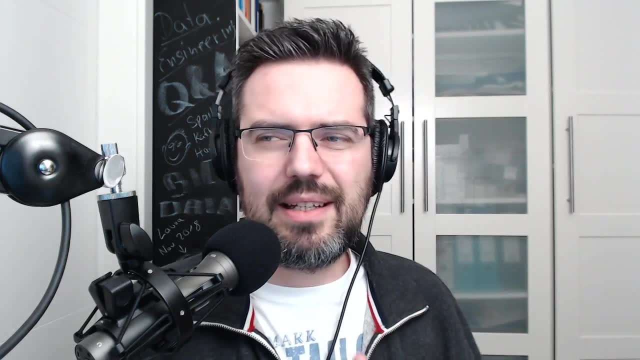 yeah, basically what you can do in in the value that you're, that you're storing, this can be everything. This can be a string, So you could put the, the, the Jason, um, the Jason, or XML data just into the value of the. 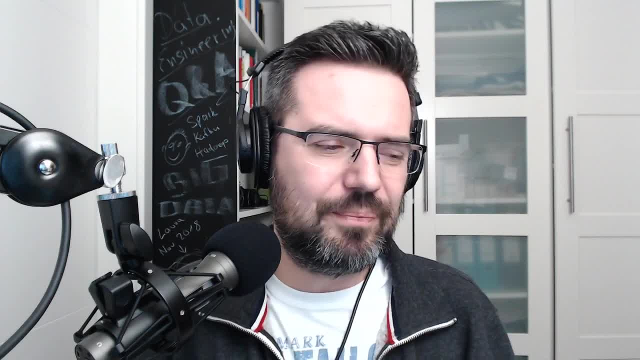 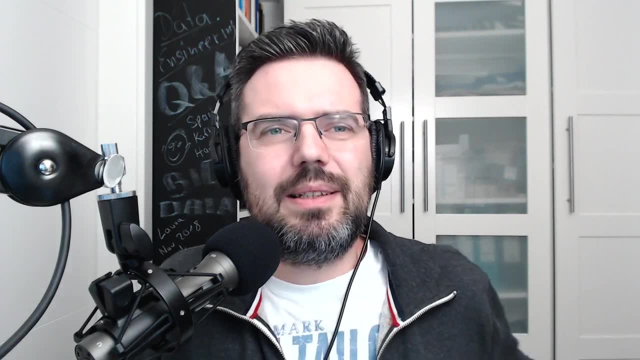 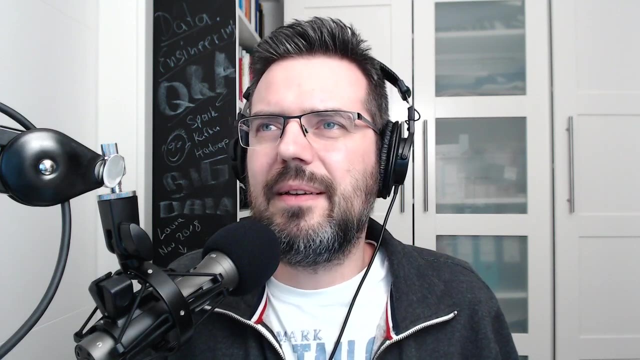 of the row and then have the row key for it. But, yeah, I'm not a hundred percent sure how this is used and how you can leverage this. But, yeah, I'm not a hundred percent sure how this is used and how you can leverage this. 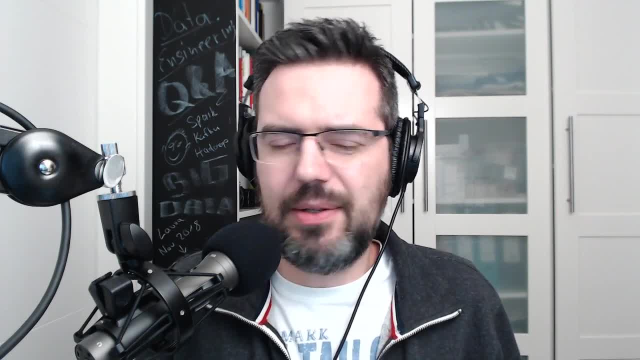 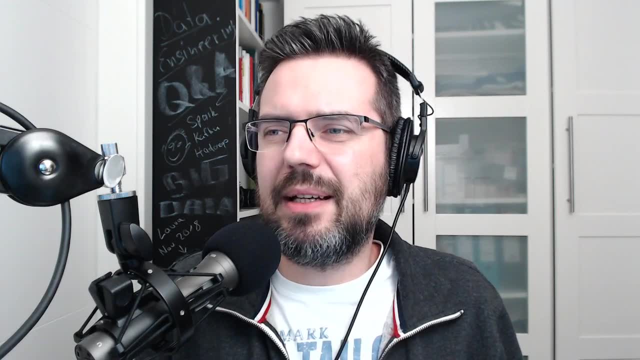 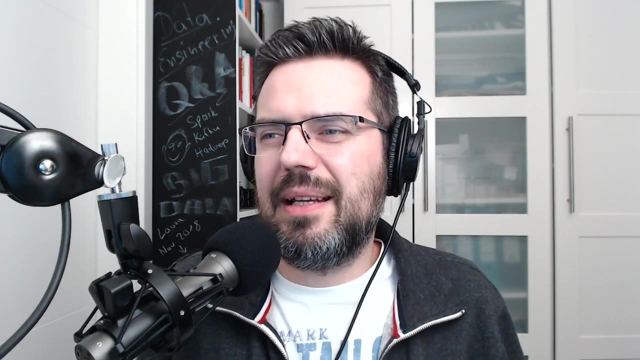 All right, Any more questions? Guys, I'm here, Um, by the way, uh, do me a favor and hit the like button on this one, So we let the algorithms know that, um, this is a good stream and this is useful information, and they. 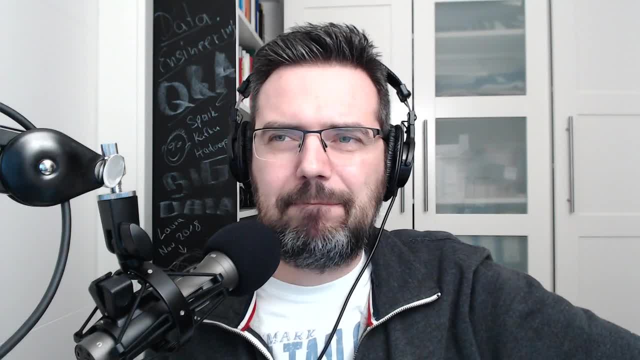 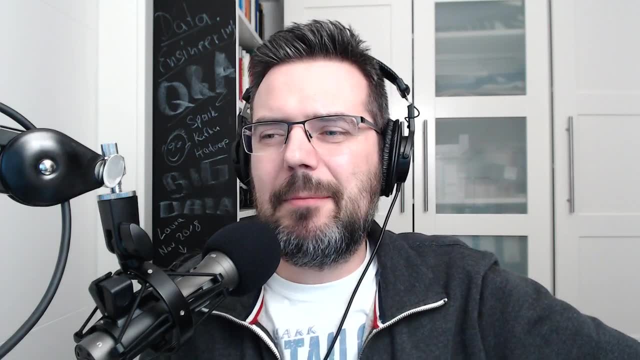 they uh suggested to people. And yeah, if you're old, if you're uh still not on my mailing list, um, what I have is a data engineering cookbook. If you don't uh have have that already, 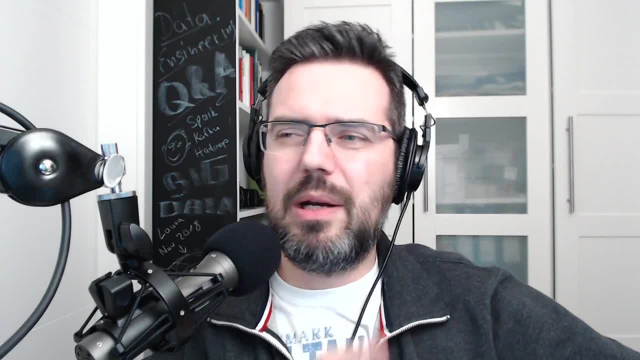 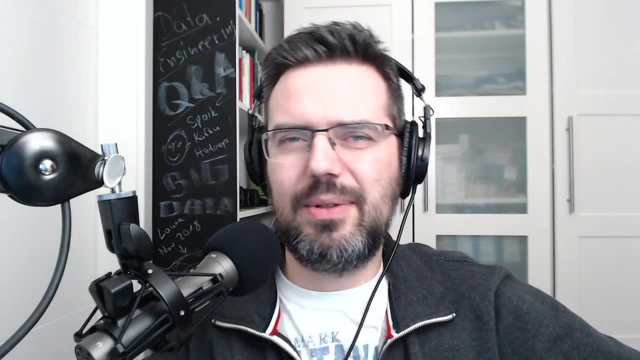 I'm currently writing a data engineering cookbook where I put then, for instance, this information I'm going to put into the cookbook at some point and then, uh, have it readable. So it's, it's more efficient, and you can download this from my website. 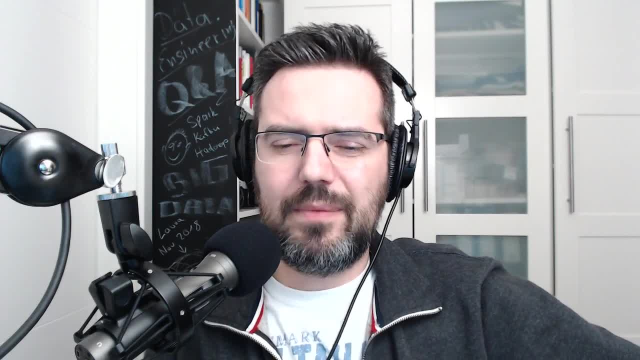 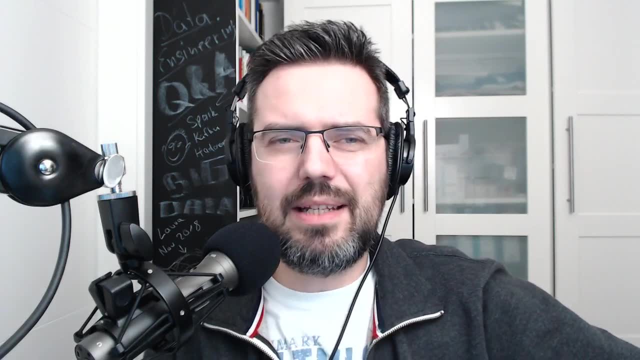 AndreasKretzcom. Um, I have a link. I think I have a link uh below in the in the description, and there is my mailing list and when you are subscribed to the mailing list you get the the. 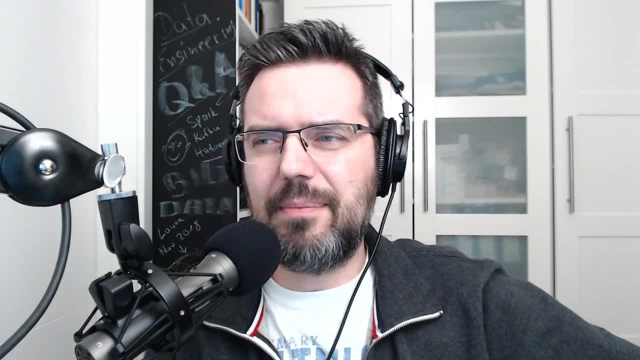 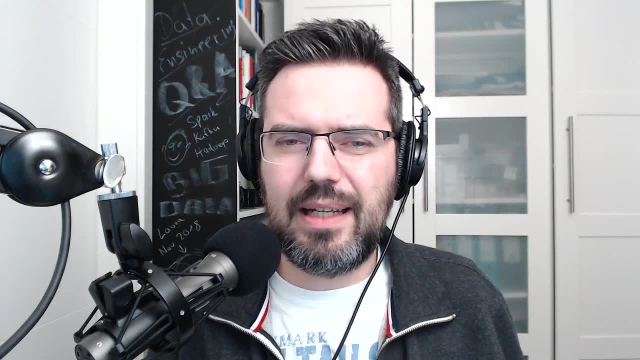 uh, the cookbook, for free. It's right now. it's about 50 pages. I'm I'm in the beginning of variety, uh, in the in the process of writing it and it's- yeah, it's ever growing. 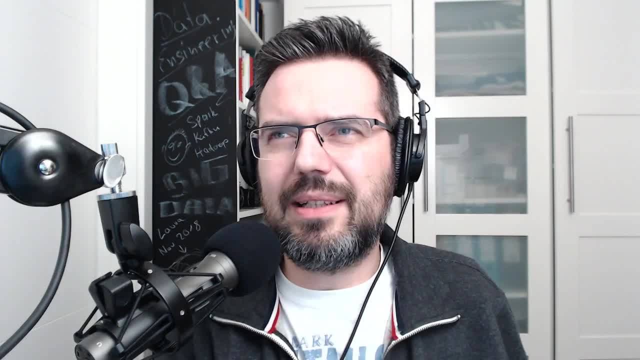 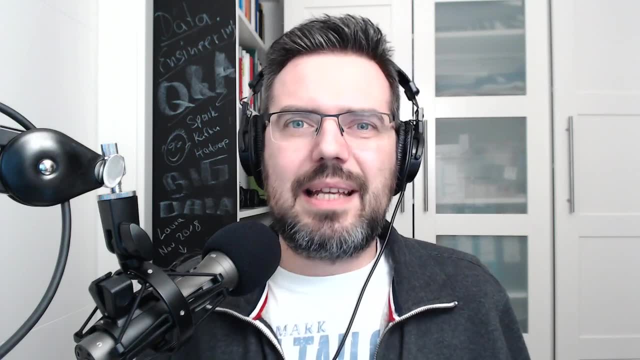 And so, uh, I have it on the mailing list. Uh, I, uh, I'm a little, you know, I don't have the time right now to take this to the full next step, but it's, it's. 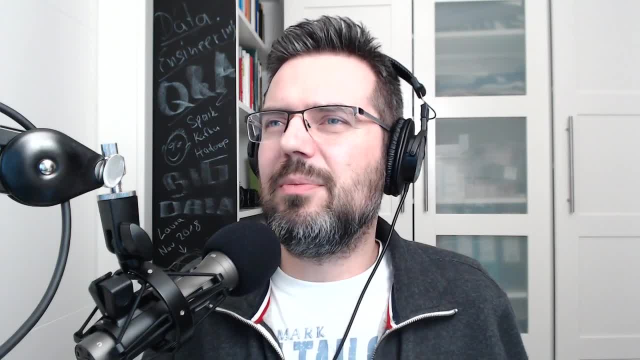 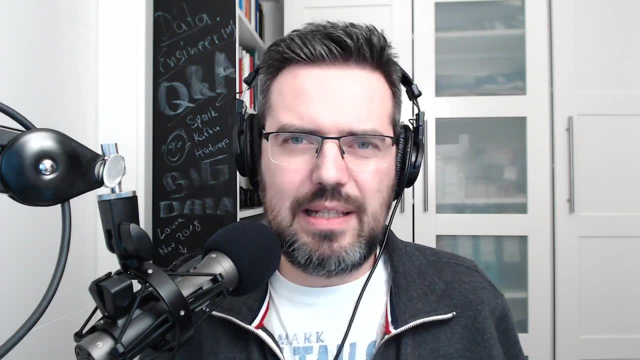 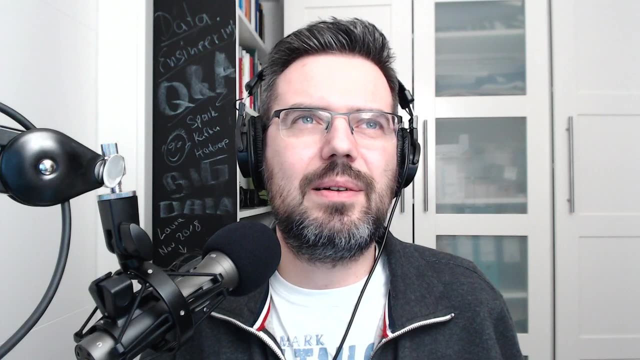 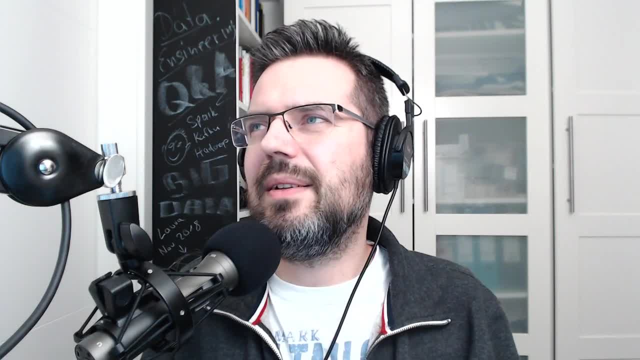 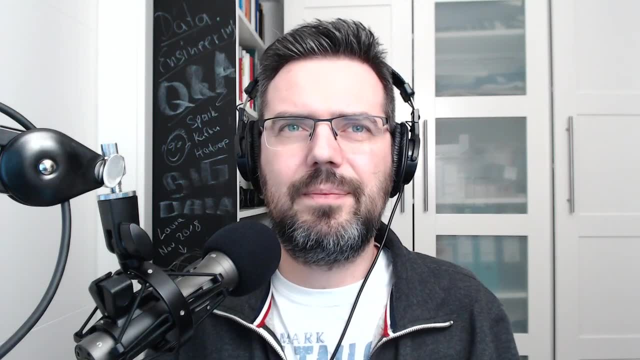 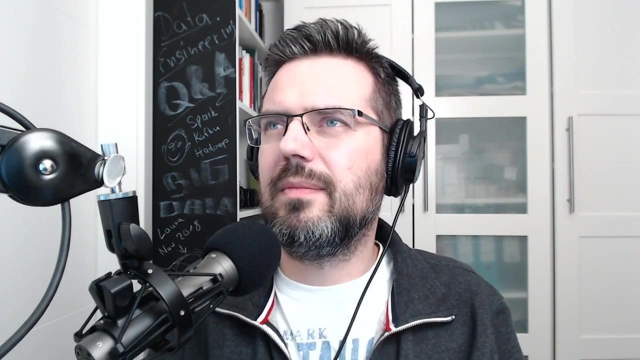 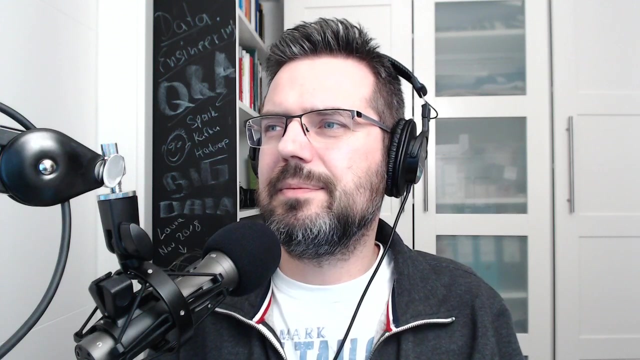 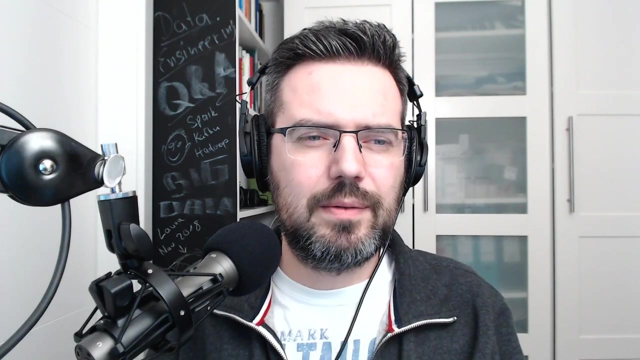 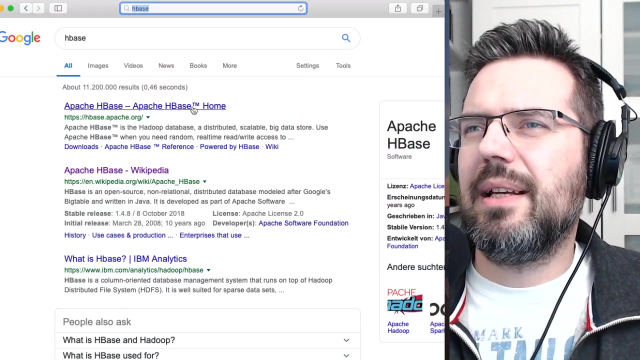 to to find it on the internet. let me just drop you here then the show you this side just a second. I need to rearrange here something to do to do, no, not Wikipedia, come on. so one good resource for HBase is Apache HBase, and they have a. they have a very 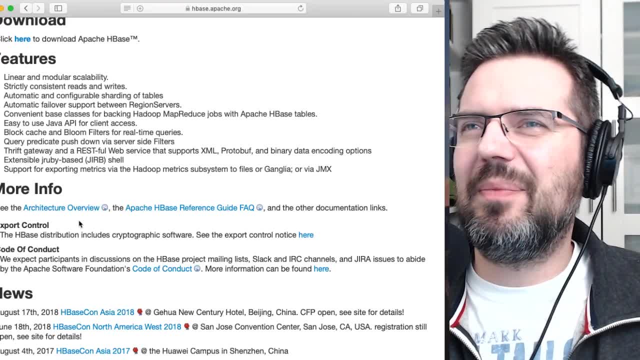 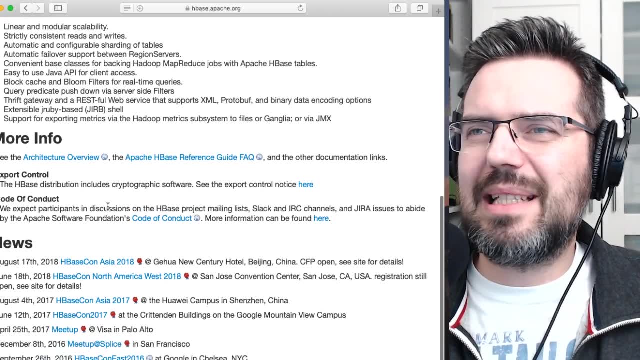 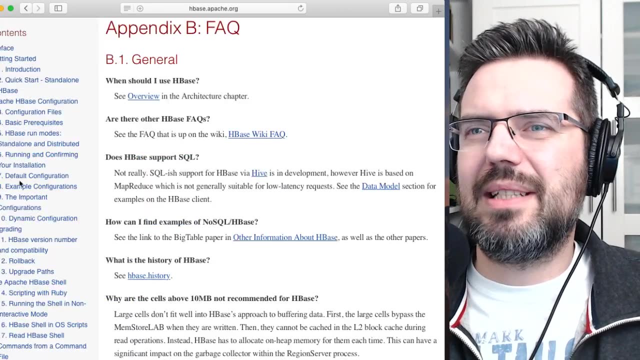 good or very, very big FAQ section and and reference guide for HBase. it's- this thing is is crazy big. so you can have the reference guide. there is basically everything- everything you need to know about HBase. so you can have the reference guide. there is basically everything you need to know about. 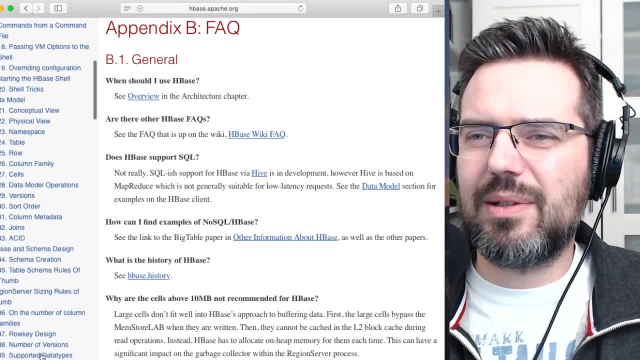 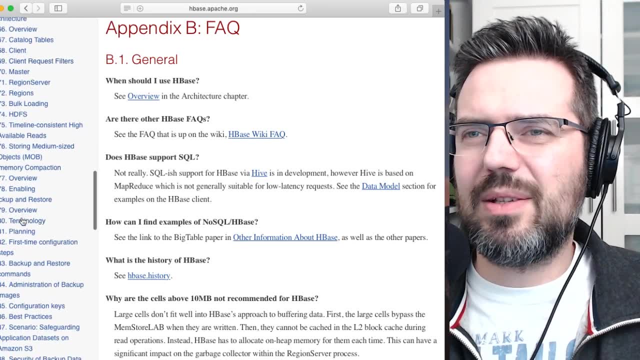 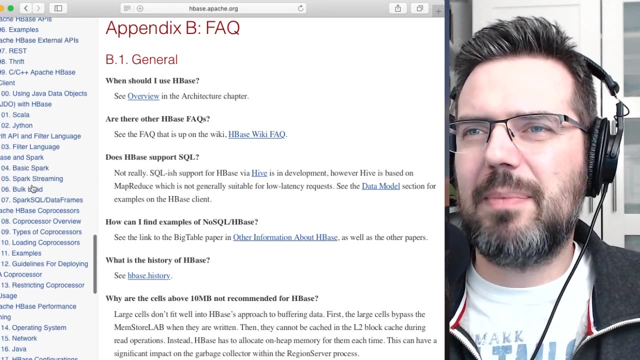 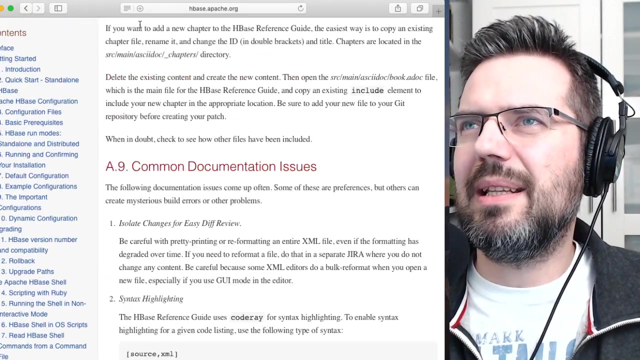 for from configuration table: rows, column, families, how you can do joins and clients and so on. so basically everything you can do, rest api's and so on. I can access it from spark and and a lot more. you can have that. I'm going to put this also in in the description after the stream. I leave that open. and another. 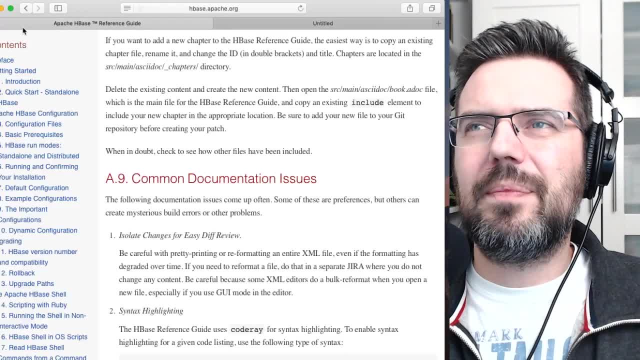 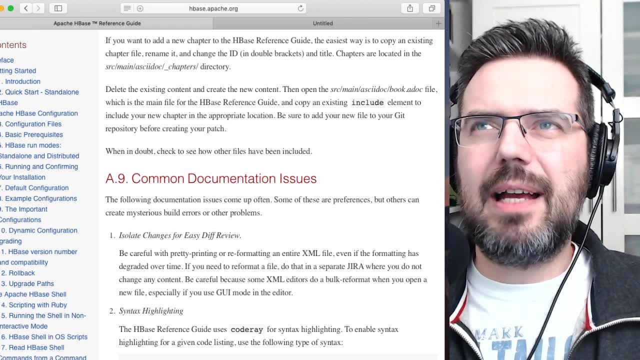 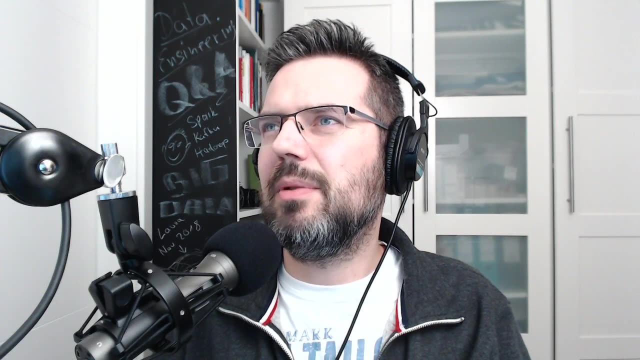 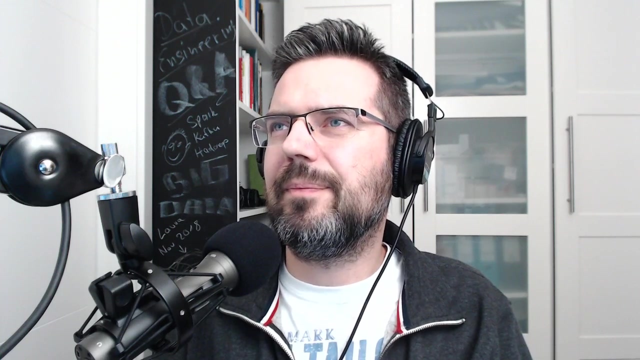 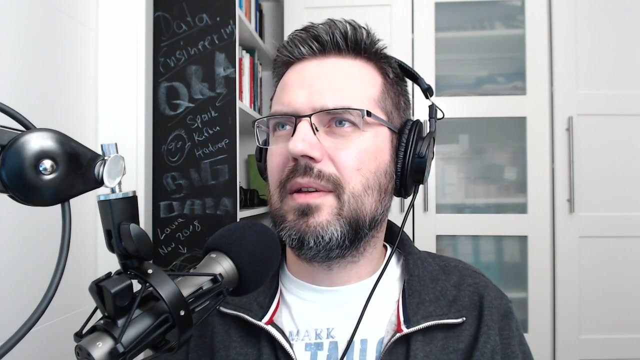 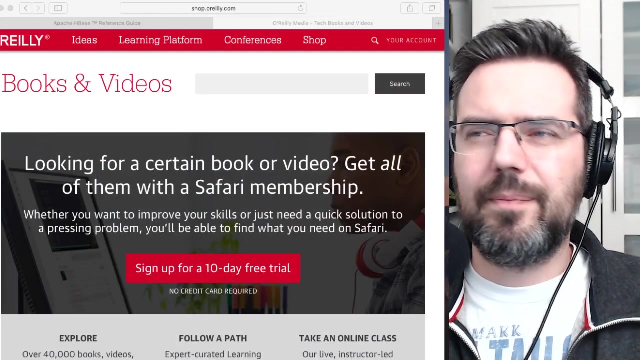 thing. what was that? I had another thing that is very interesting that you should. yeah, there is a book from O'Reilly. just let me just search this. there is a good book from O'Reilly, O'Reilly media. yeah, the shop, the shop from O'Reilly. there is a good book about HBase, and this is 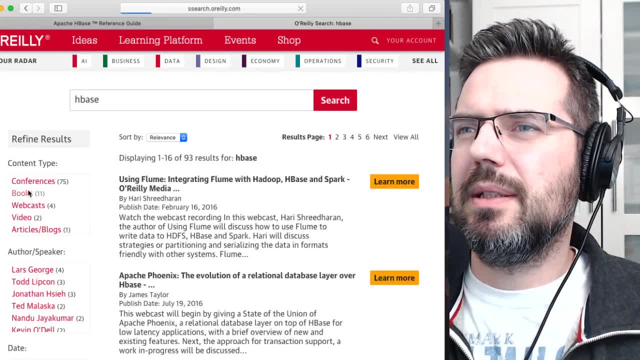 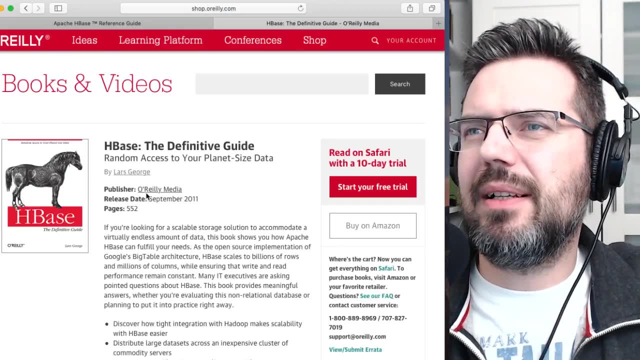 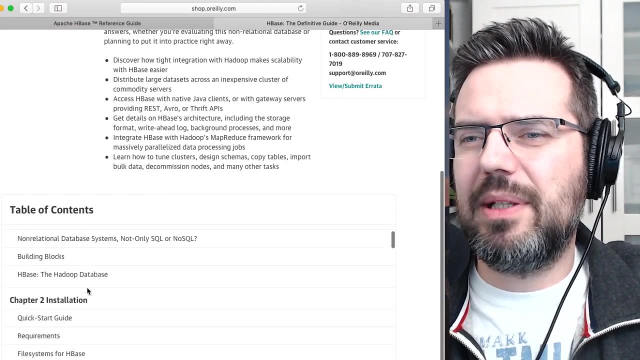 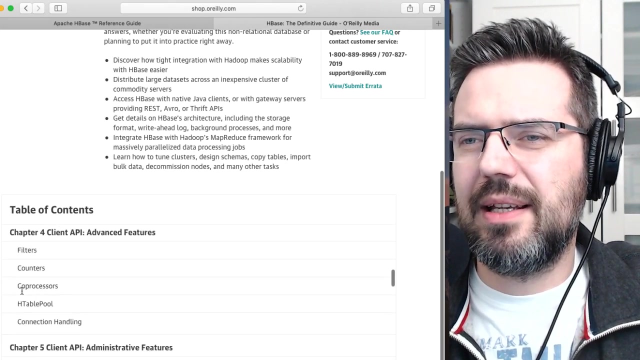 called books. this one here, the definitive guide. this is a. I have this book myself and this- this one is really good to learn- HBase. they have basically everything from introduction how to install it, basic api's- how you can do scans, for instance, and filters, counters, this. so it's, this is. 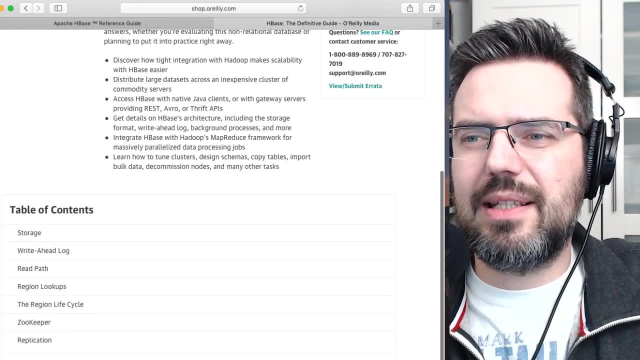 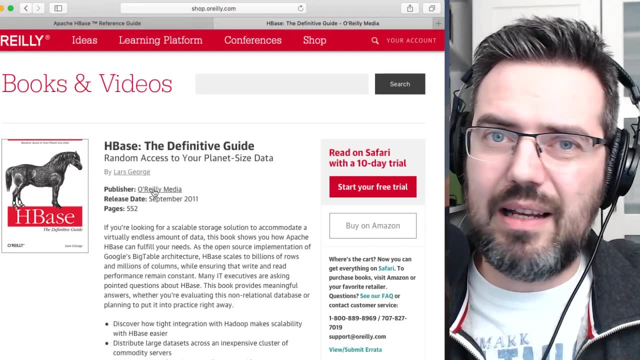 a huge thing and I would suggest, if you want to, if you want to, get into HBase and check out this book, HBase definitive guide. it's not as with all O'Reilly books, it's it's not simple, it's not cheap. I'm gonna. 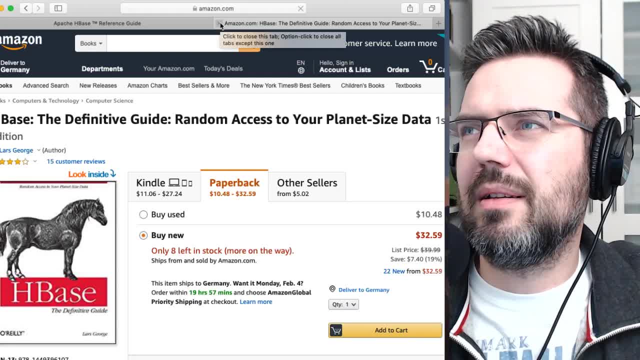 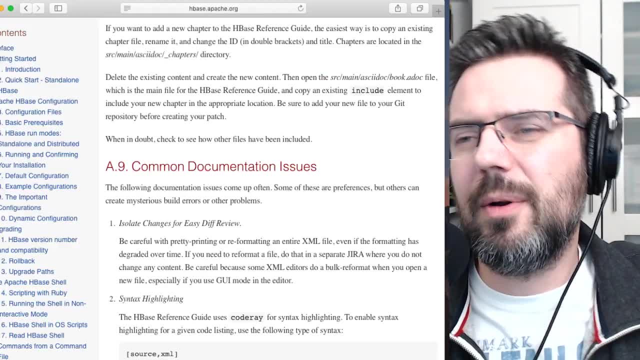 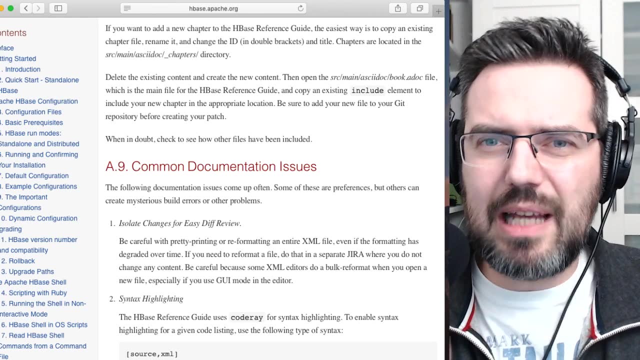 just this, just check. it's okay. twenty three, thirty two dollars, so it's not. it's not super cheap, but I would say, if you're, if you're getting into HBase and if you're using HBase for work, get the book. if you're just for learning it, 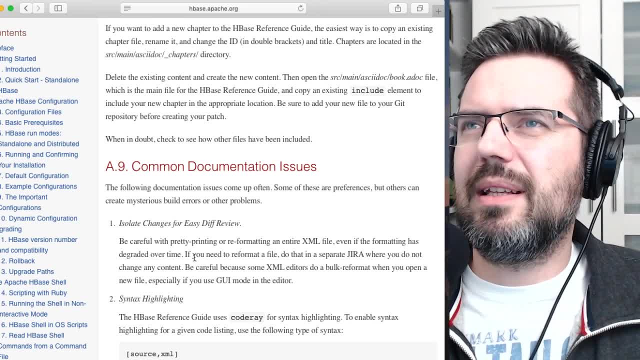 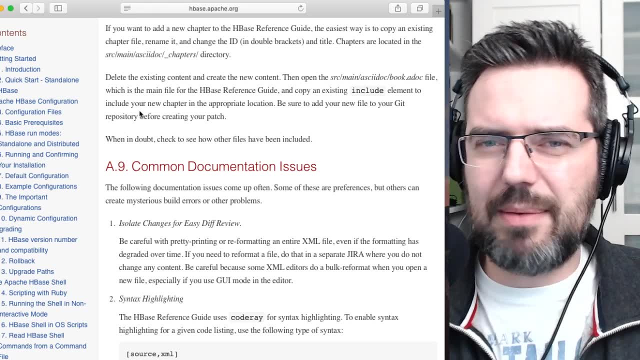 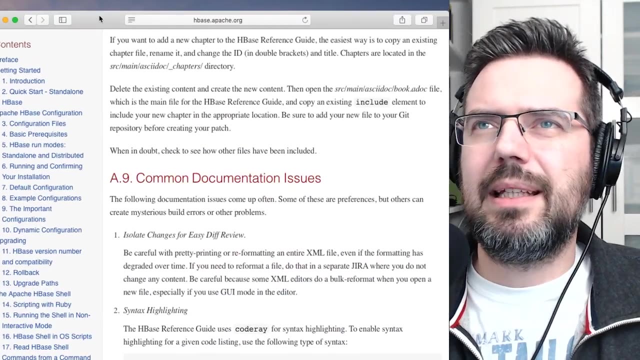 don't bother, go with the, go with the documentation here and go with stuff you're finding on O'Reillycom, the internet, that's. that's completely. it's absolutely sufficient. yeah, so I know I have closed the book again, but I going to put the link into the of the. 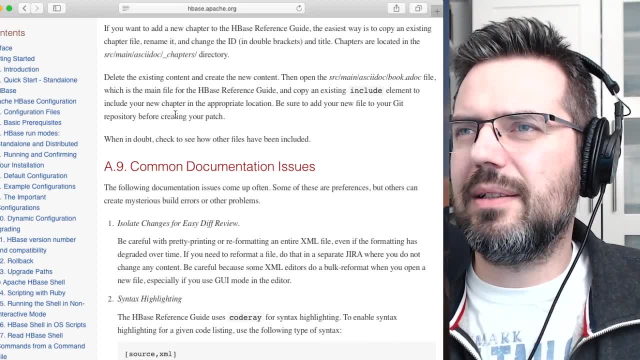 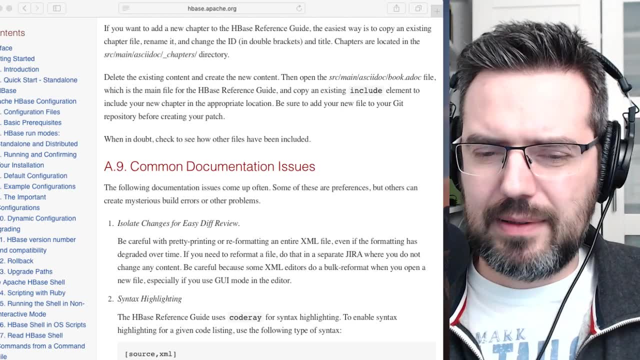 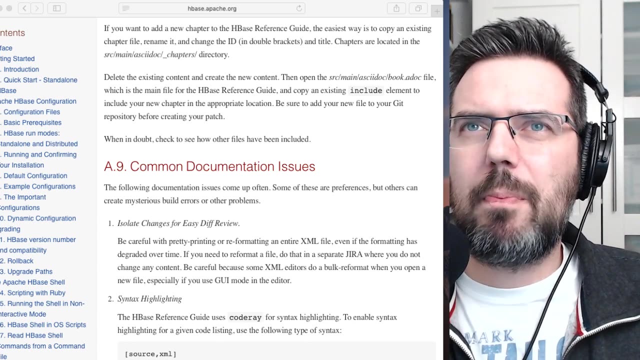 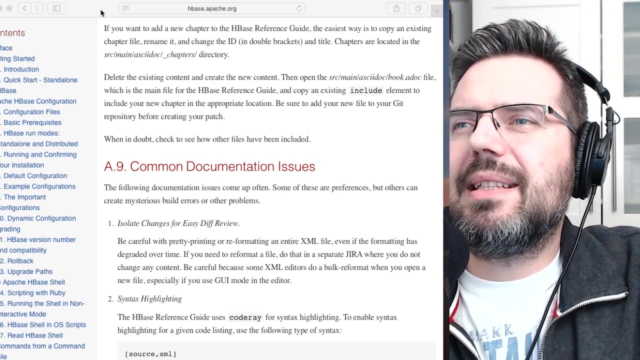 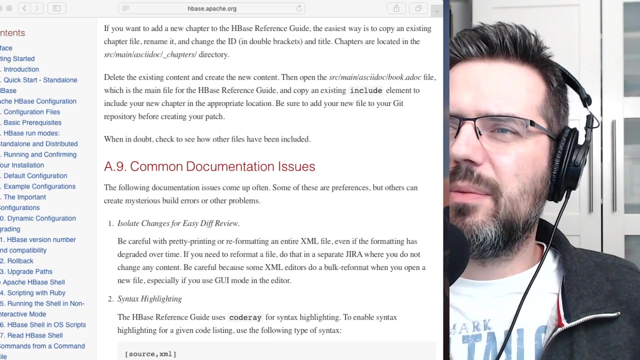 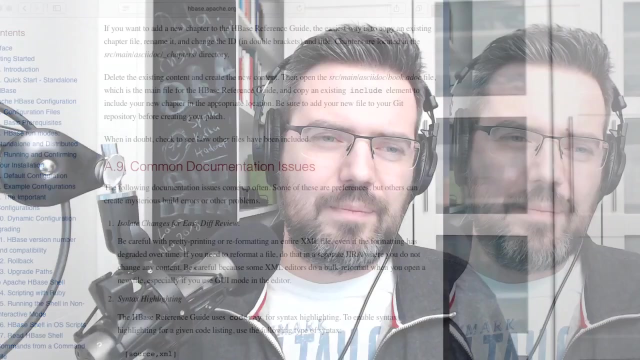 book, into the section built into into the description of the of the stream. yeah, okay, something more. do I have more? I don't know. I think this is. this is a good overview of of what you can do with with HBase, how this works. of course there are a. of course there are a. 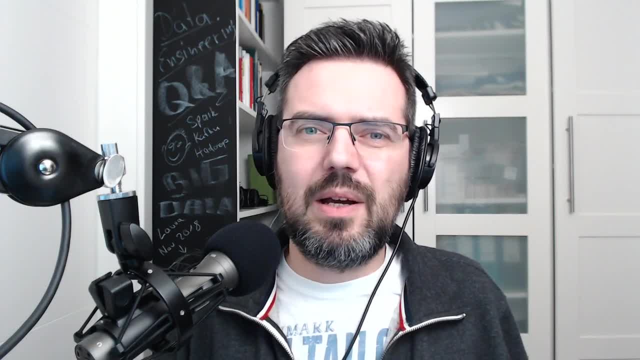 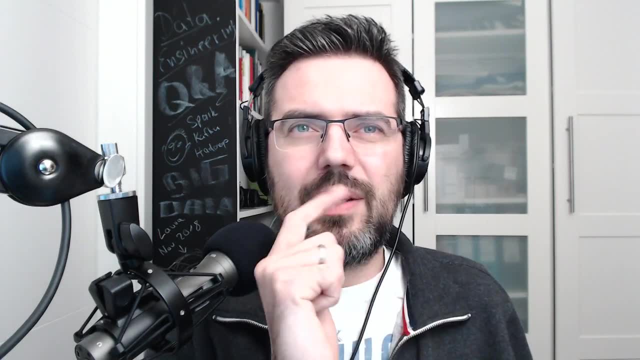 lot of a lot more no sequel databases. what you can do with HBase is you can do with O'Reillycom do, is you can. I would recommend you look into Cassandra. you look into you're looking at MongoDB. MongoDB is also very interesting. a lot of people use MongoDB. 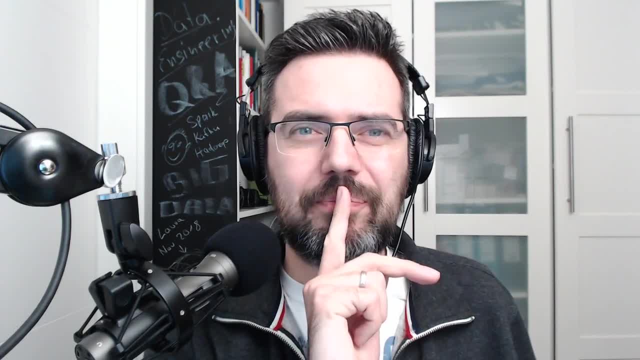 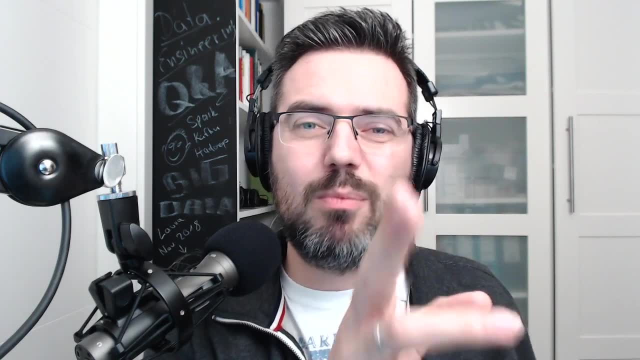 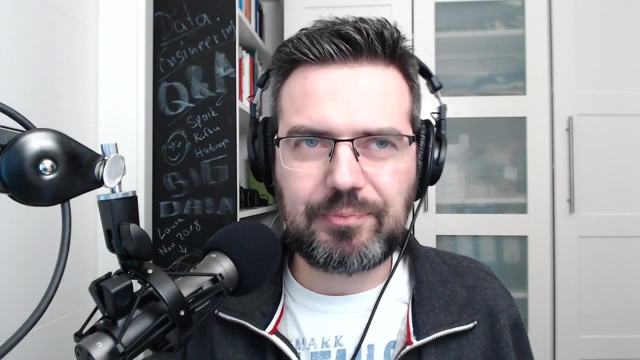 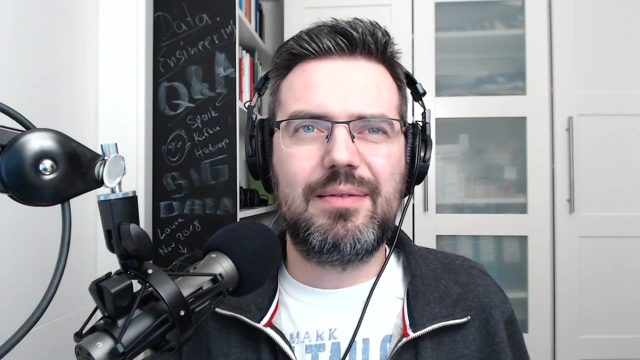 and one thing that is quite funny is if you, if you're on AWS, the DynamoDB, that is more or less HBase, so the DynamoDB works more or less like HBase. it's super interesting and yeah, thanks for the great content. yeah, of course you're. 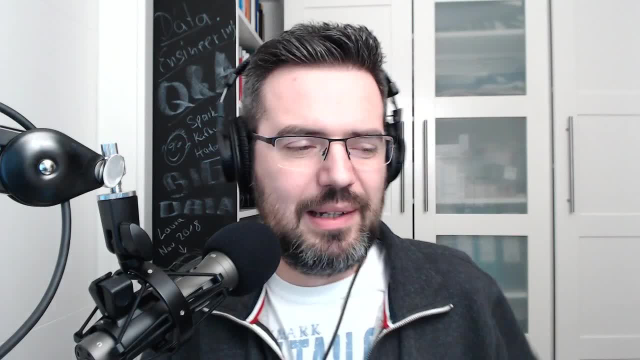 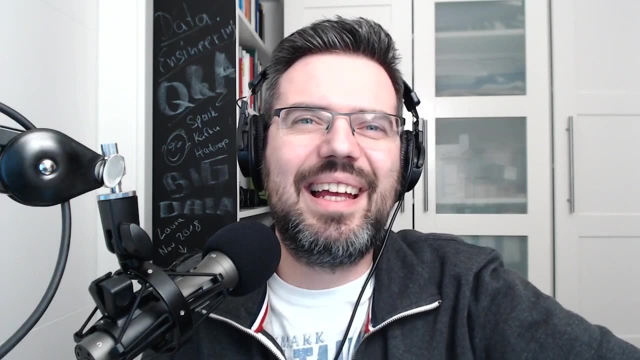 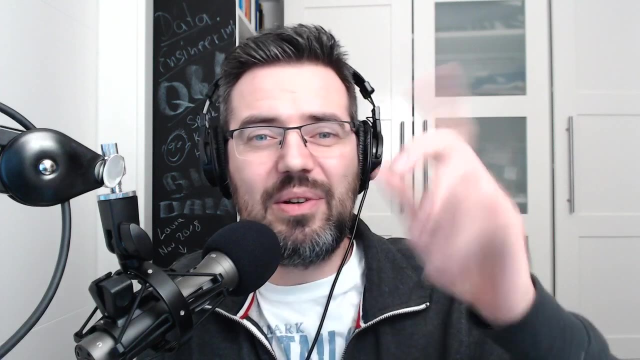 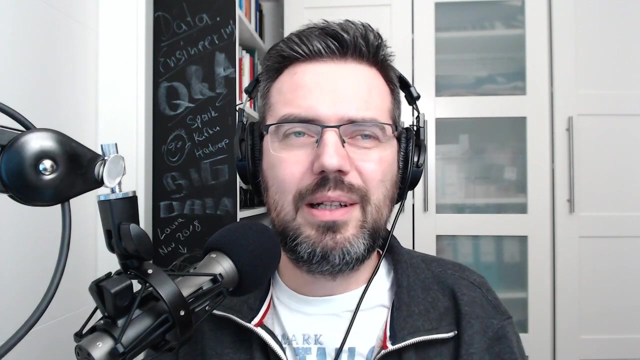 welcome. I'm trying to do the streams more often now. yeah, if you like it, let people know. yeah, yeah, check out the complete video. I'm already in the QA section. so if you, if you have some something would like to know, Karthik, let me know I can. I can stay a few minutes on, yeah, so 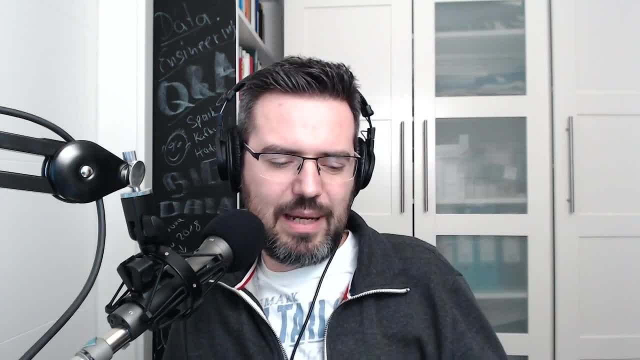 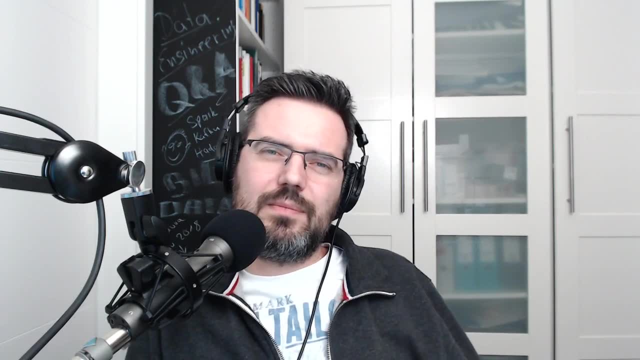 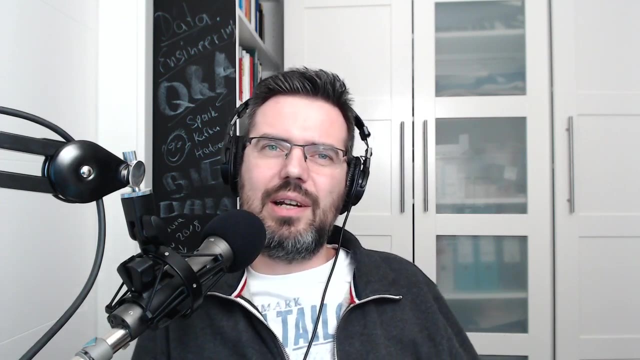 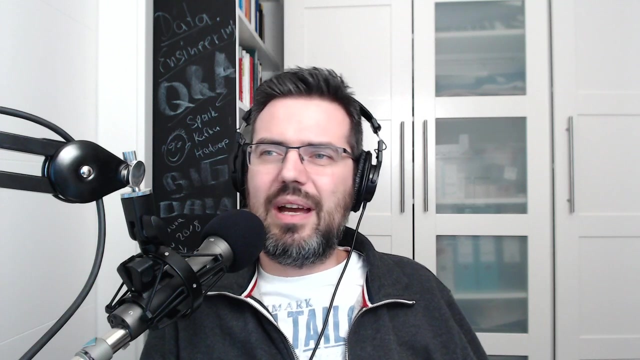 I have. I have very- I have made very good experiences with HBase. it's it's simple to set up. if you're running something like a, if you're, if you're already on something like a Cloudera installation, it's already there and the configuration is quite simple. you have a, you have a, you have a shell where you 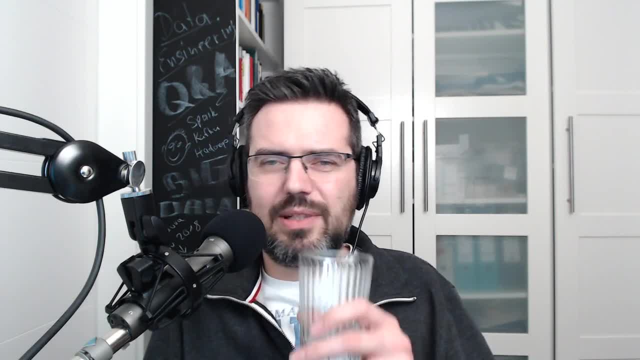 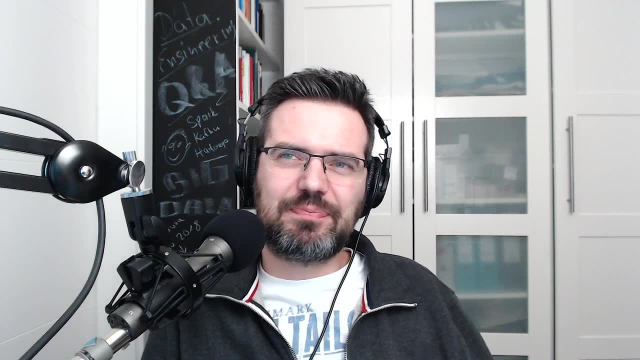 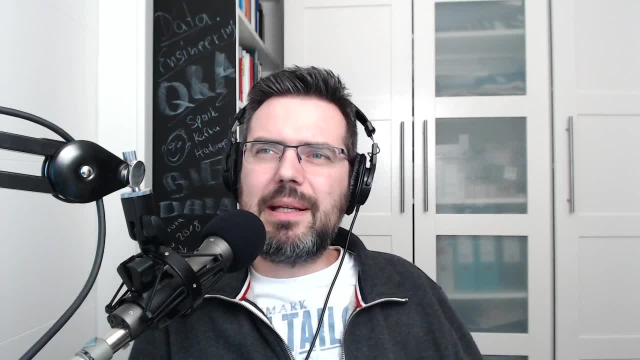 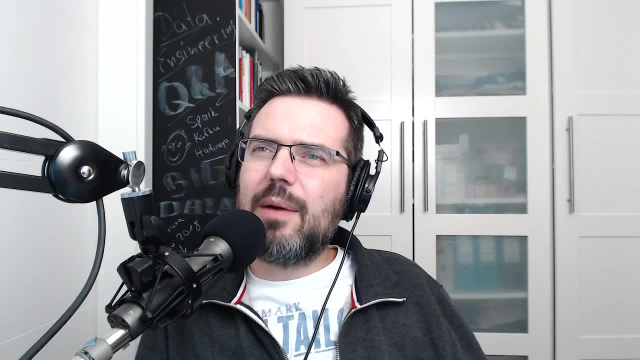 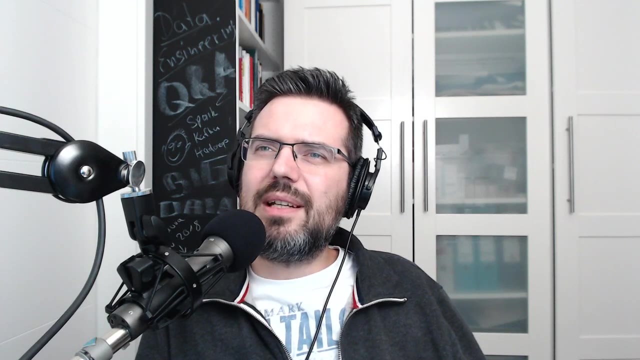 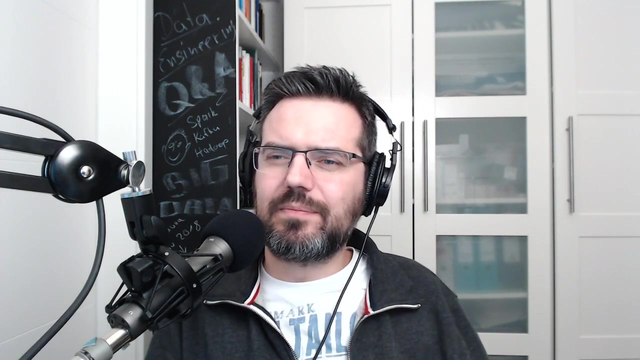 I personally, I like it. it's a bit it's a bit complicated to actually. one thing that I would need to look up now again as well is how it's how data is written to HBase. is some with something like you write a headlock, and this is also? 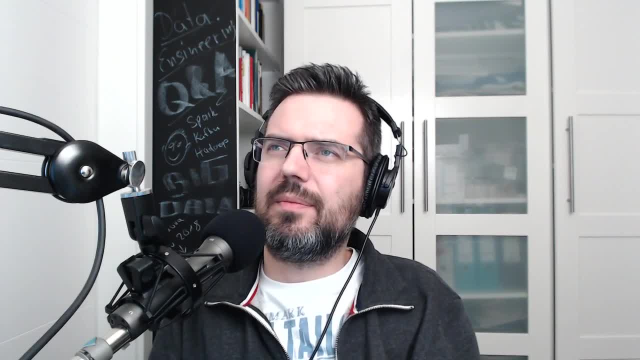 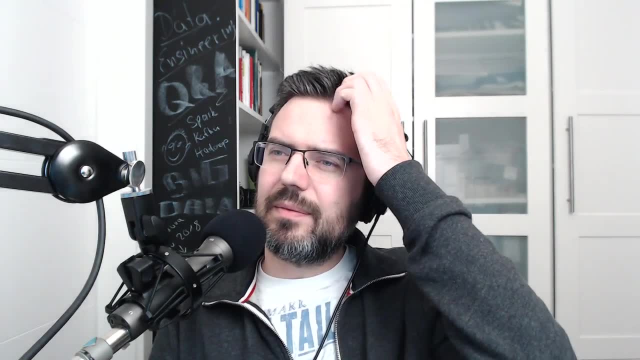 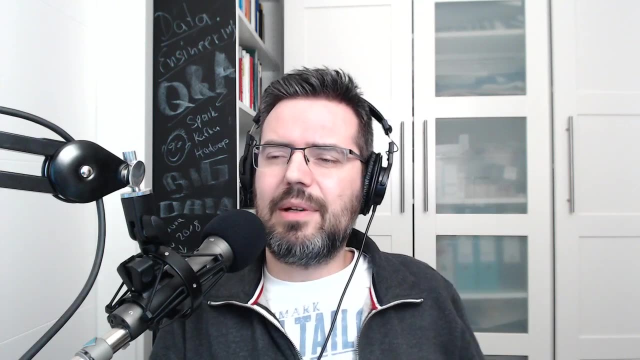 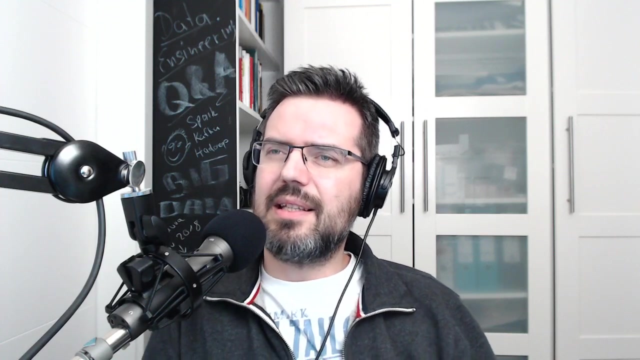 something interesting to get into it. can I find this? yeah, yeah, the write a headlock. so basically everything is is put into the write a headlock at first and then dumped into the store, and so this is. this is something that that is interesting to look up at the beginning. 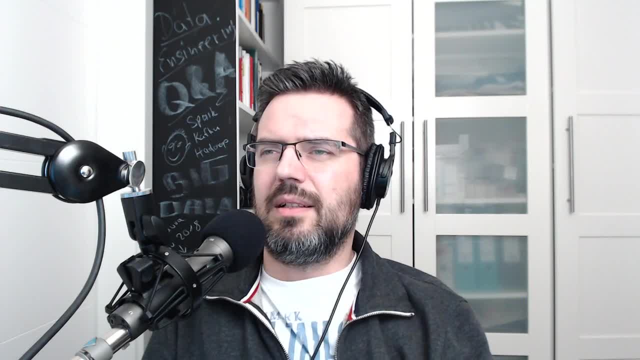 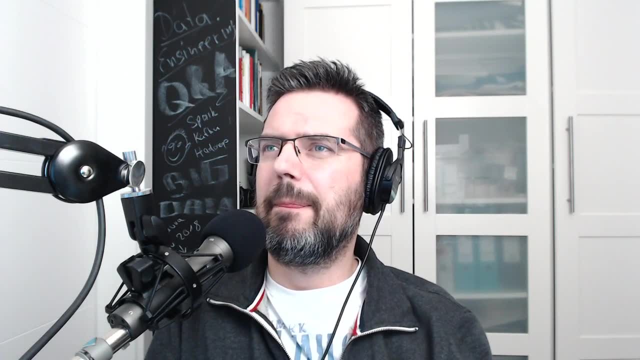 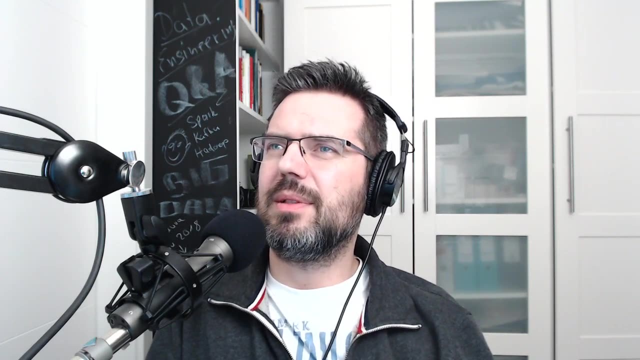 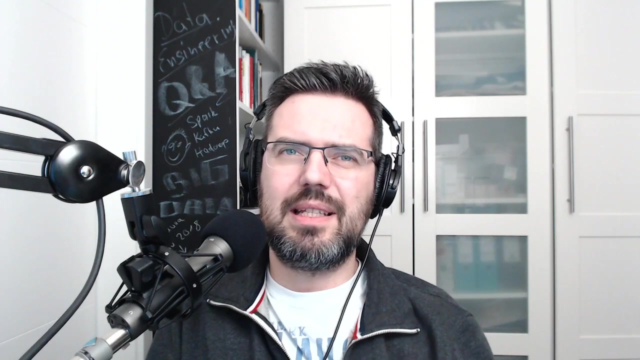 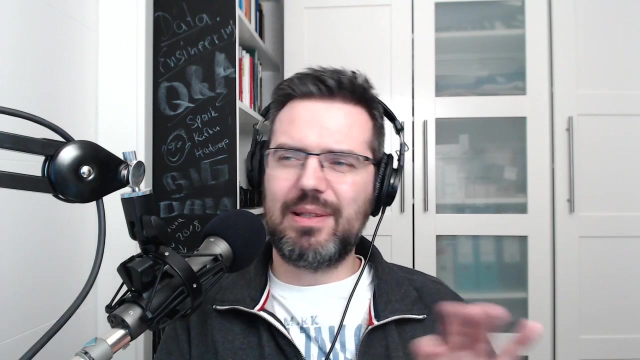 when you're, when you're using it. I know this, but I have to admit I have already forgotten it because I'm not right here. they have something interesting. there are also, with some some interesting, a regional splitting. you can split regions and what the system is doing also is compacting regions together and minor compactions with small. 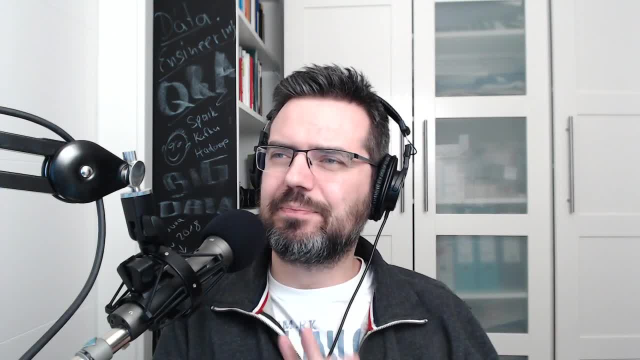 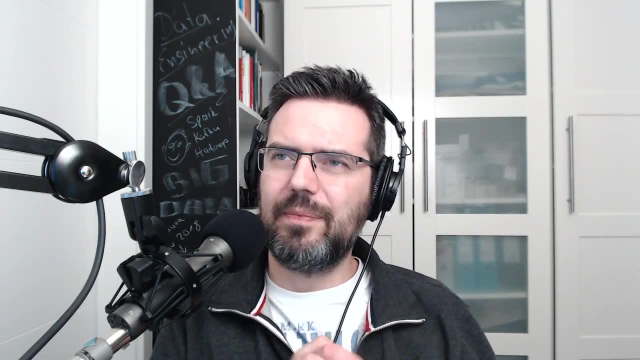 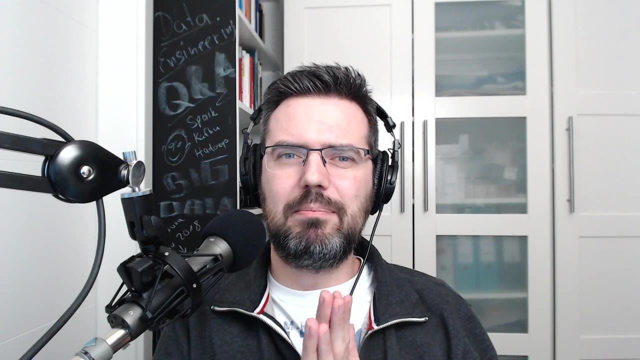 smaller things or major things is the system is doing, but yeah, I'm not sure I- or major compactions and it's. yeah, it's a very interesting database design and very versatile. yeah, um, i'm basically through, i think, um, is there something more that i have you know? 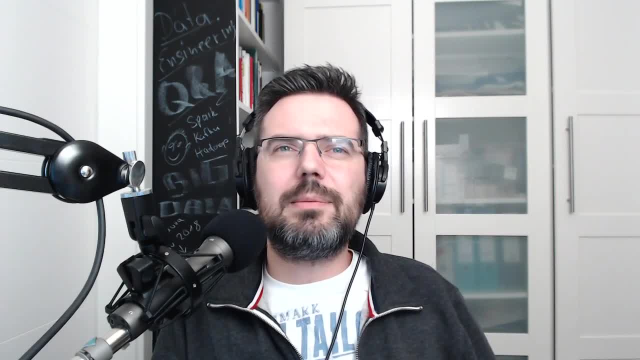 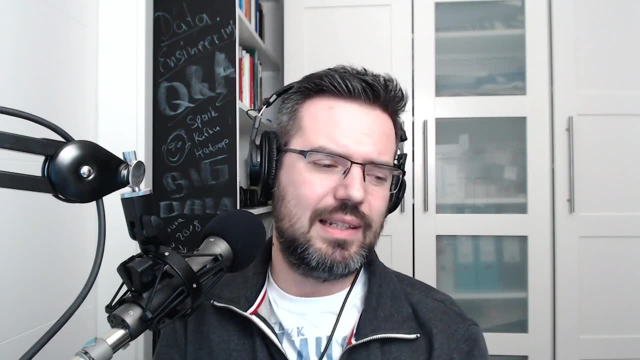 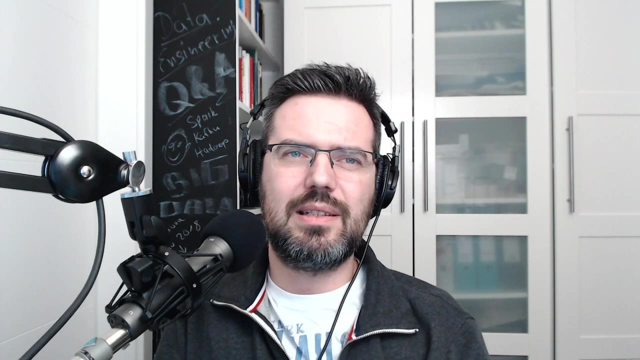 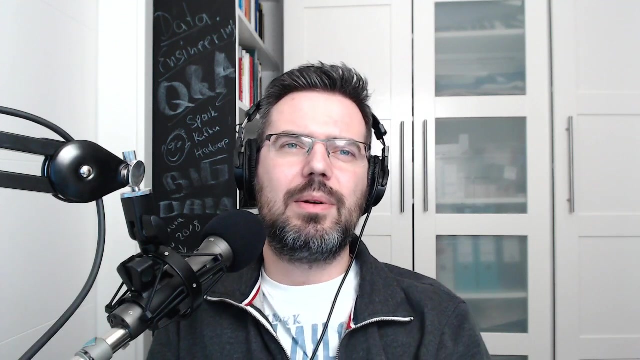 i would like to show you- um- i don't think so- calm families. we went over time to live that this is very, very good. we went over um counters that you can very easily set counters and increment decrement counters. um composite key design: hot spotting how data is stored. 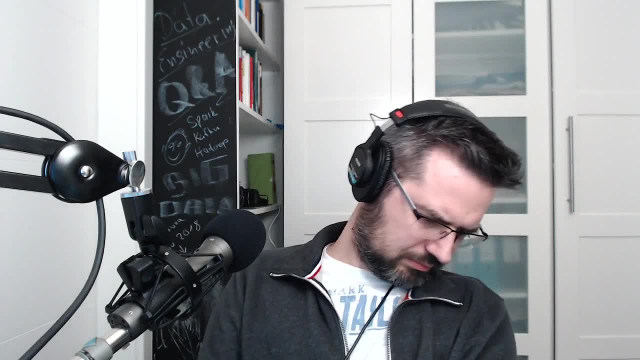 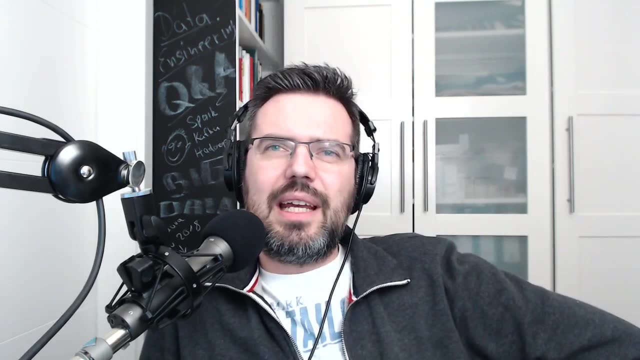 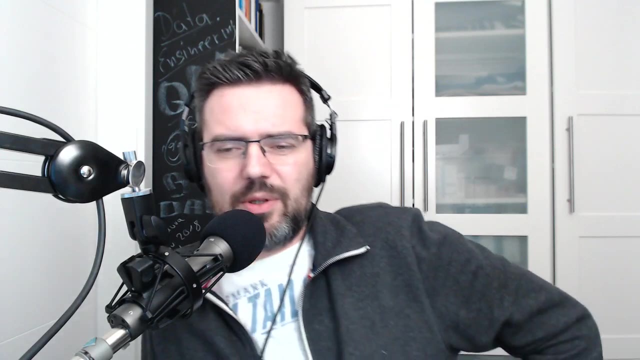 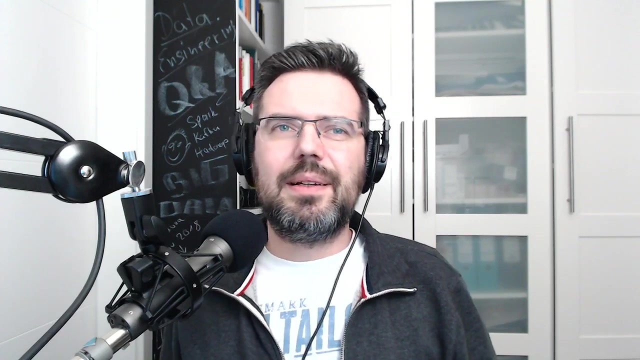 sql. yeah, whoops. okay, i think i made a mess here. um, that's it for today. um, great having you here, guys, let me just check the chat again. okay, no more questions. um, yeah, if you like this one, let me know. uh, write a comment if you have more on this video. 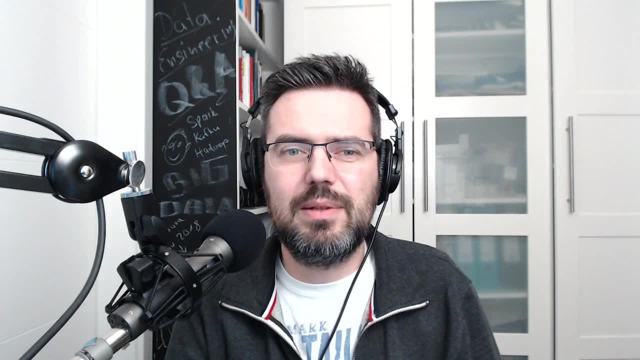 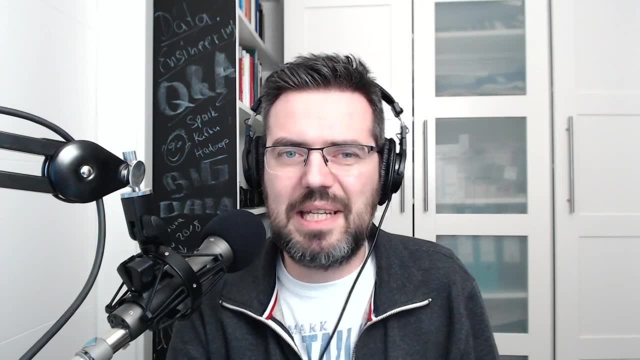 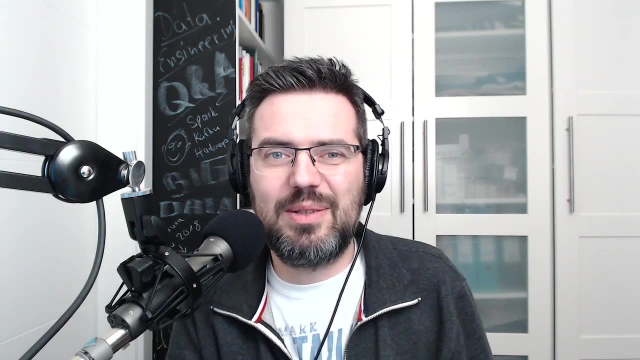 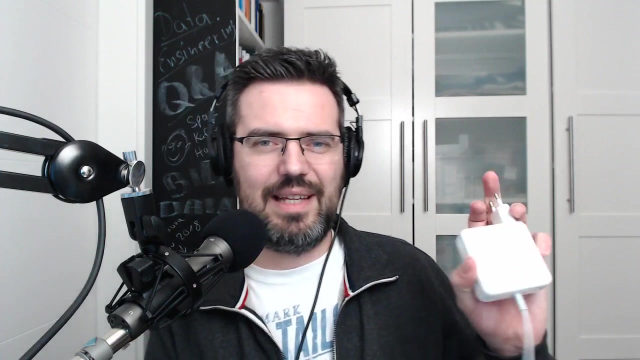 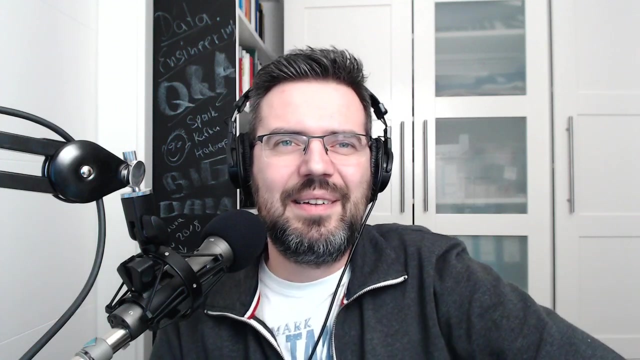 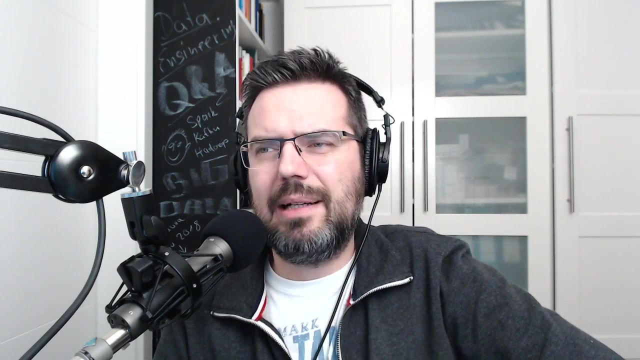 if you have questions about hbase and about no sql databases. and yeah, see you tomorrow. i'm going to. i'm going to work on on uploading this also as a podcast to my, to my audio podcast. ah, now i know what is okay. the um, something fell off here. um, okay, then see you tomorrow. i'm trying to do another stream tomorrow. i'm not 100. 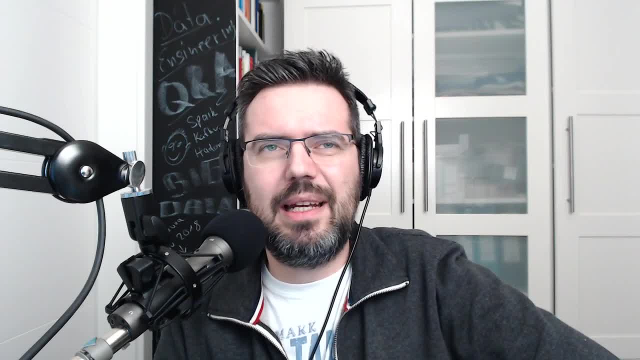 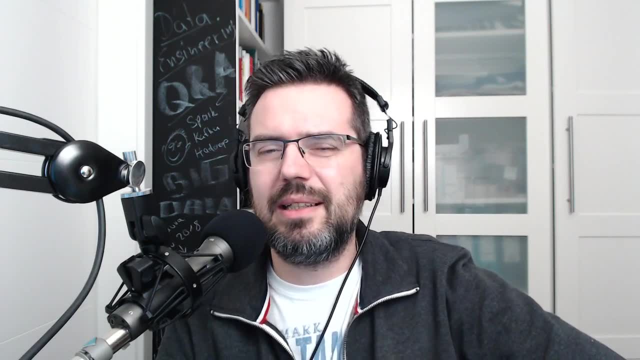 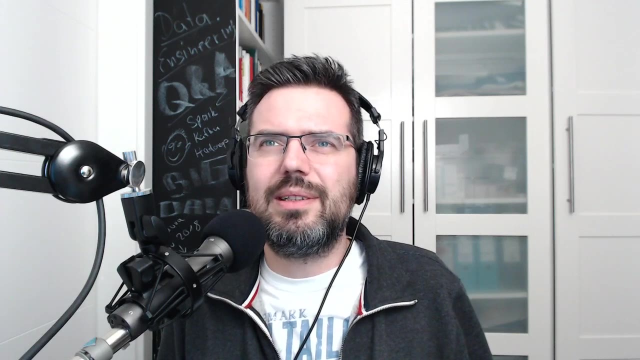 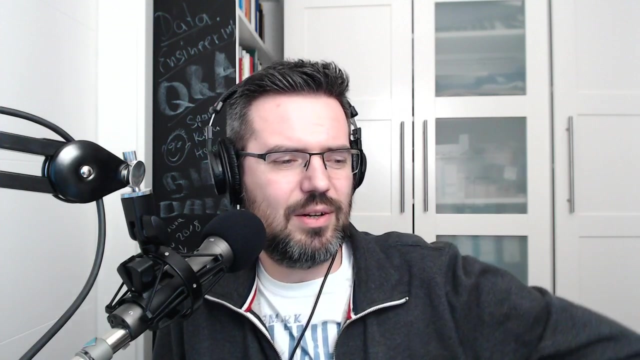 sure about the topic yet. um, i will let you know and i will upload some bits here on my facebook and my my linkedin. um, i'm also working on a, on a clips channel, for so i have the, so that i have the plumbers of data science channel where i do the long form videos and then i am. i'm thinking about 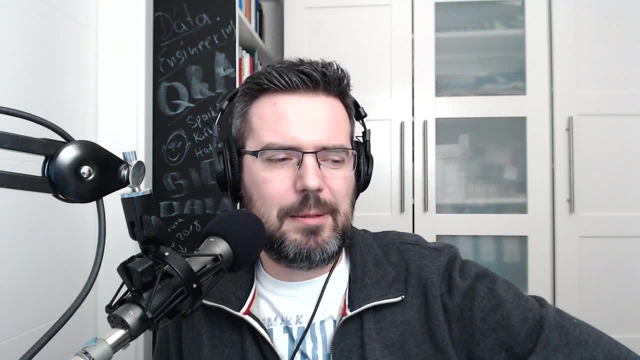 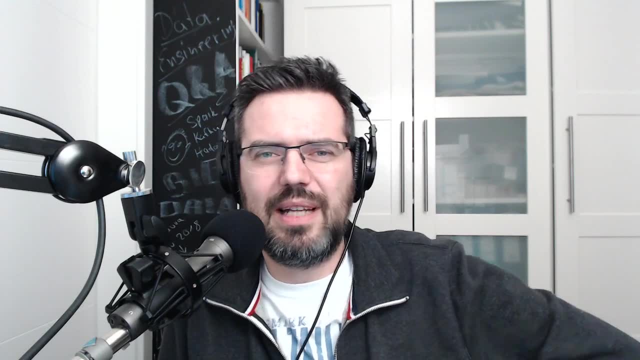 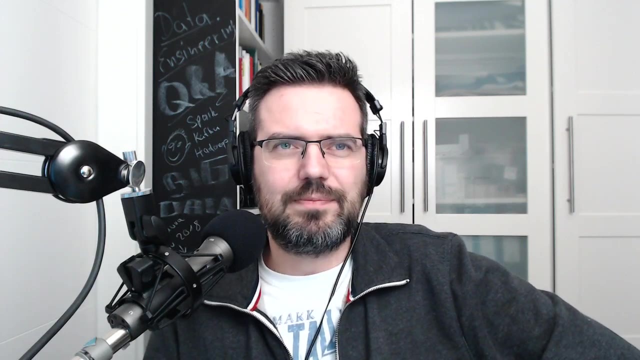 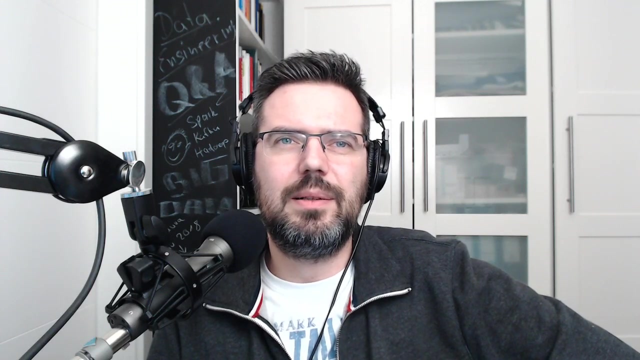 setting up another channel for small clips, um, where you can just get into into the, into the interesting stuff and if you don't have time for the whole stream and you can just search for it, okay, so uh, another um, is it all? is it possible to do a stream on data pipelines? i'm not 100 sure what you mean with is. 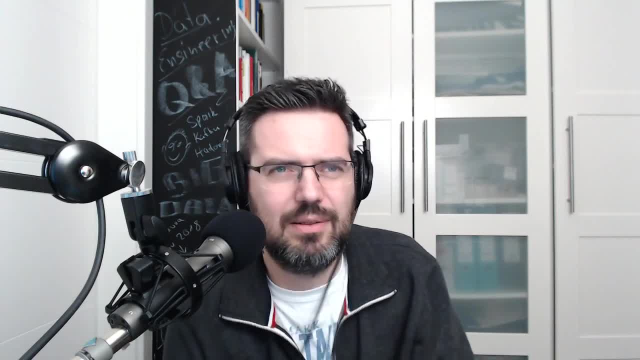 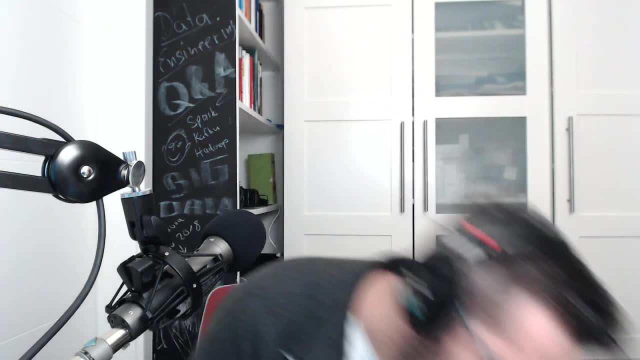 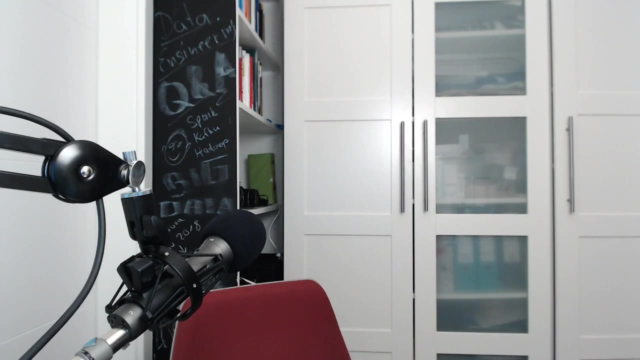 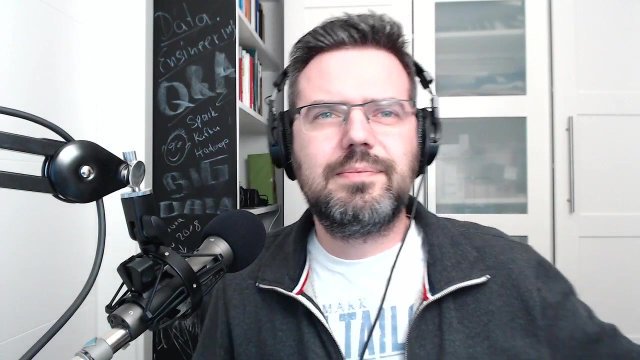 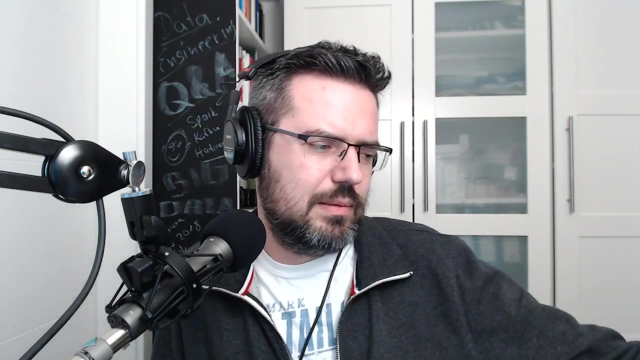 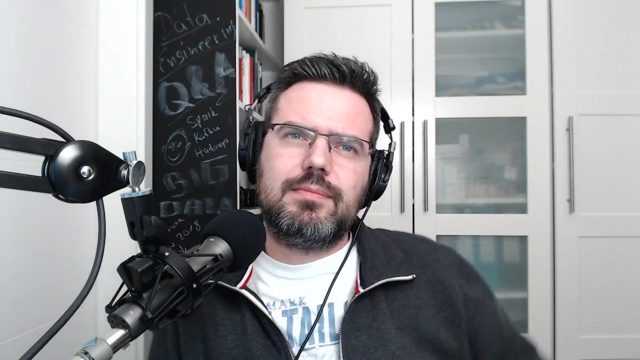 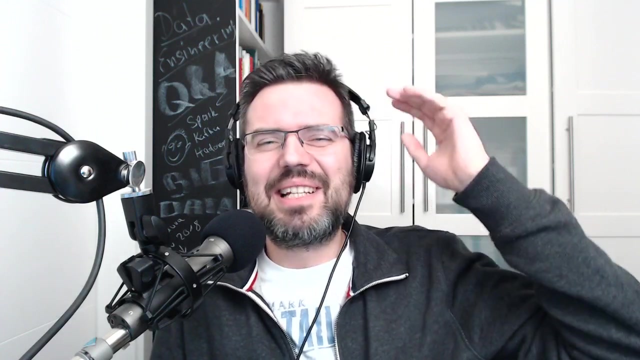 it possible to do a stream on data pipelines? can you elaborate a bit more while i'm plugging in my macbook again? all right, um, um, um, sorry, just stream on data pipelines. um, this dream on data pipelines, ah, okay, now i. i was still. i was still, uh, hung up on on hbase and and no sql database. 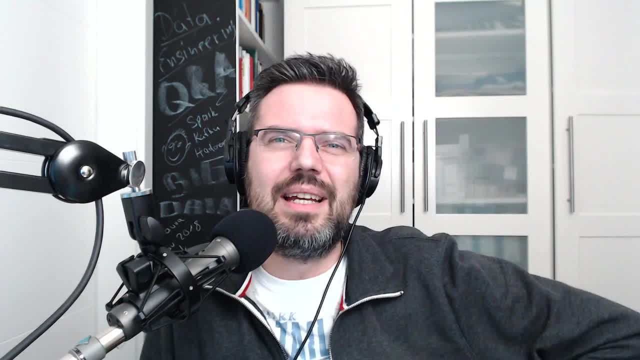 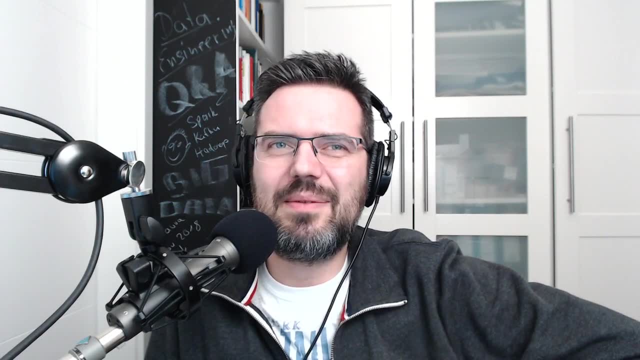 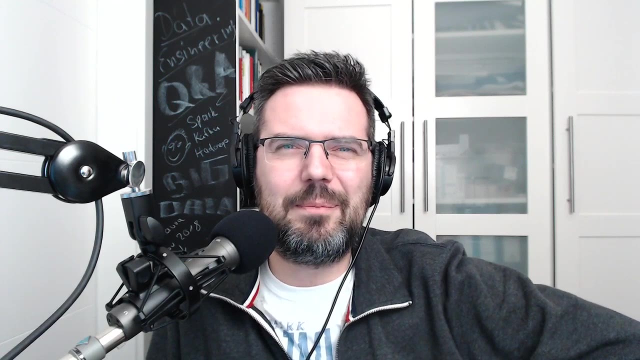 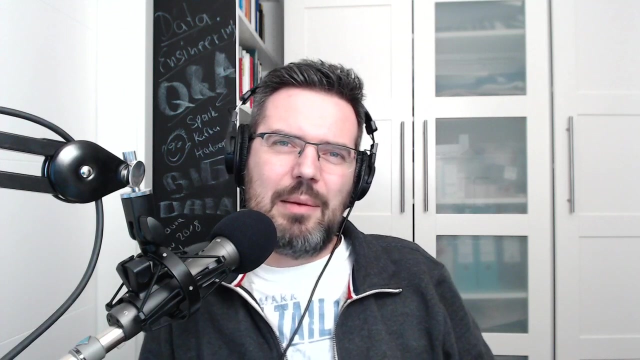 yeah, i'm actually i have, i have thought about this. um, no problem. um, this is something. i think this could be something that i i need to do in the future more: um, get into um architectures that people are using and, uh, analyzing what they are using and how they are using it, because, um, i'm i'm not 100 sure how to. 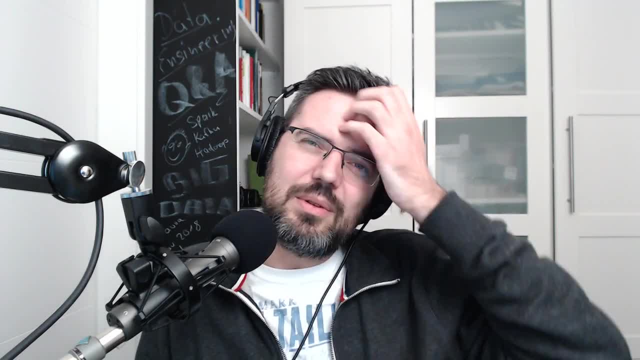 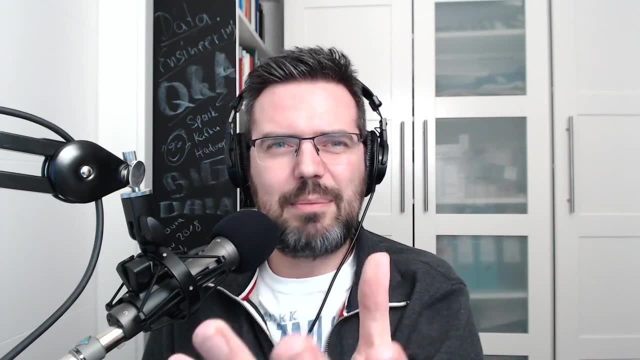 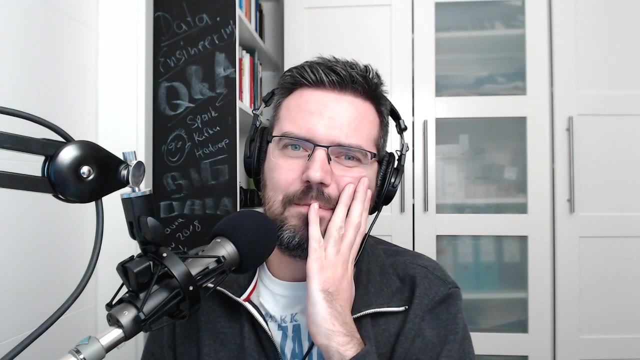 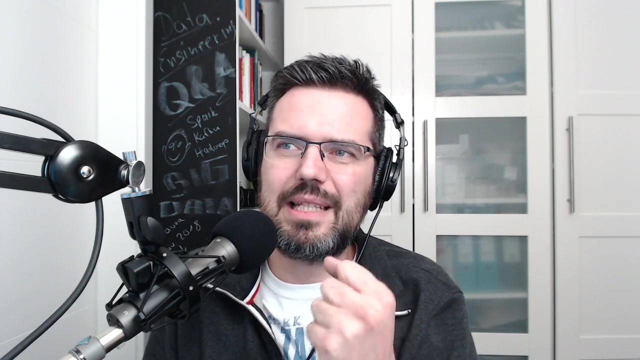 where, where this podcast is going. i'm, i'm or i'm always working on um getting. i'm always searching what is, what is helping you guys and how can i, how can i provide information to you that is that is unique and that that you, yeah, that that, uh, benefits from my experience in. 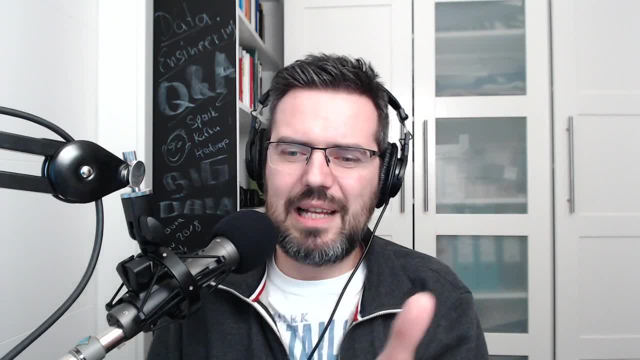 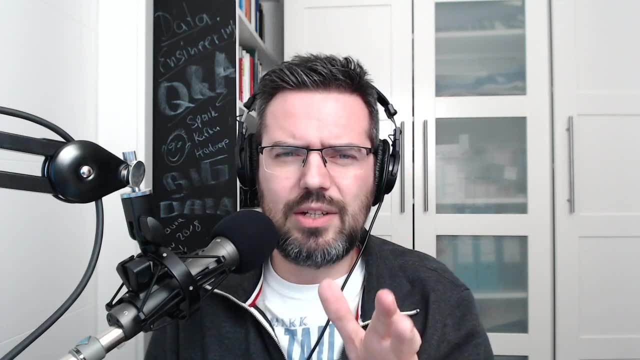 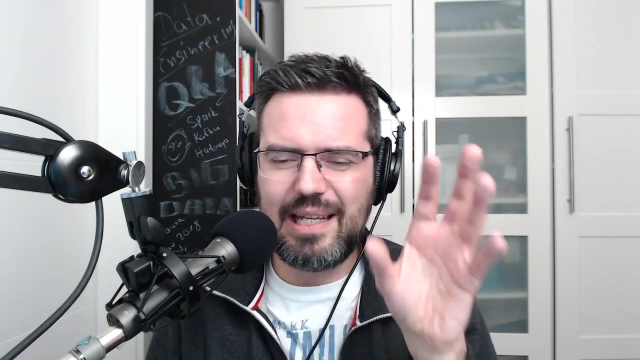 this field because, um, although these streams like this are, i think these are, you know, i think these are necessary and great and and interesting, but, um, i'm 100 sure you can find this, all this information that i have given you today, you can find this on the internet and, uh, there are there. 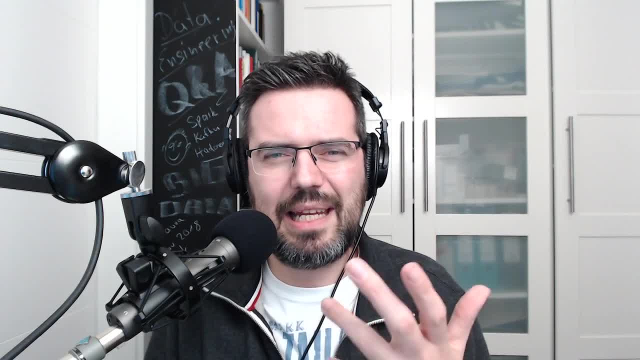 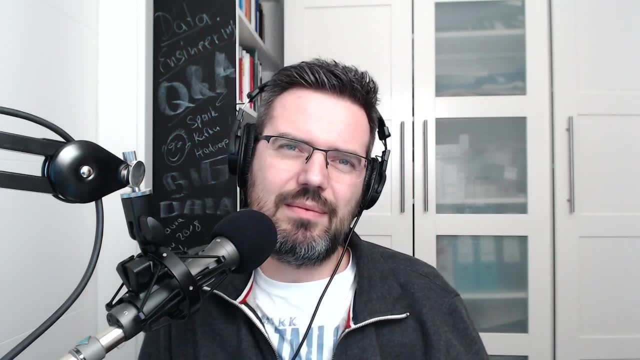 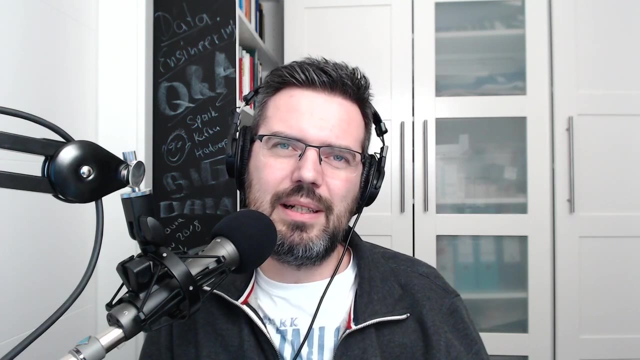 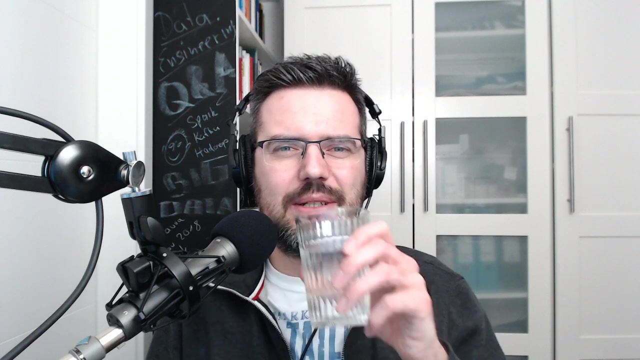 are other people that may be even better in at explaining this, but, um, maybe there, maybe the the direction i'm heading, um, i'm heading, is to get more into into architectures and and reviewing architectures of other people and what they are doing. um, this might, this might be, might be interesting, because i'm, um, i'm also more interested in in the 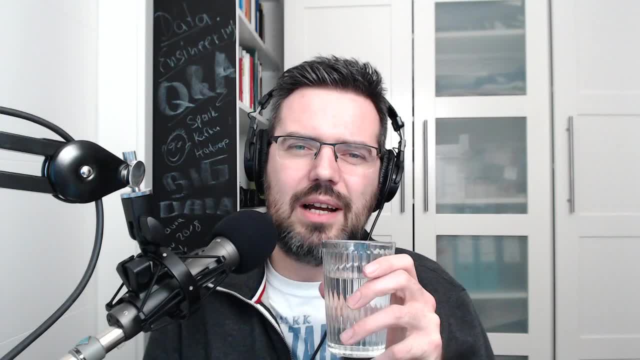 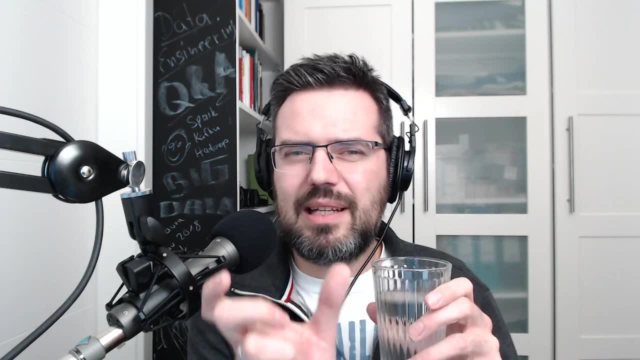 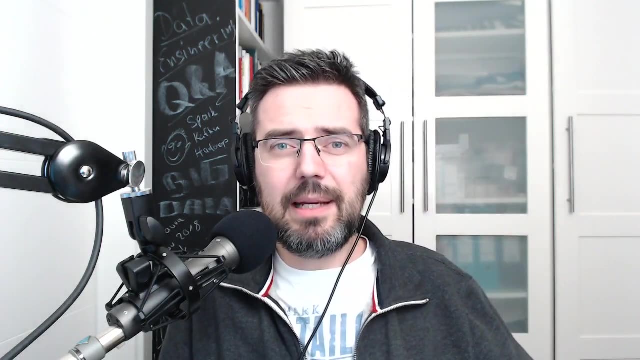 architecture guide, or in the in the architecture side of of the whole thing and not um, and not this one thing of of, uh, processing in spark and only coding in spark, and and so on. so this might be a. it might be an interesting direction. um, yeah, so if you, if you have a, 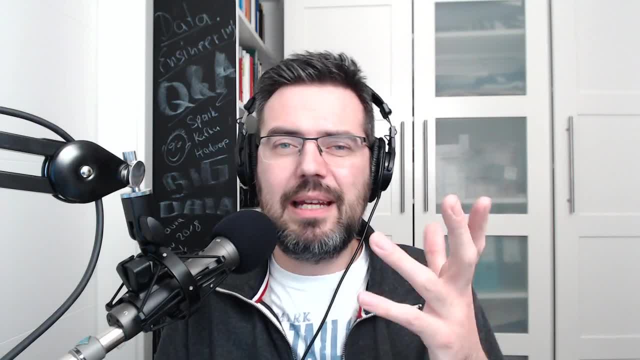 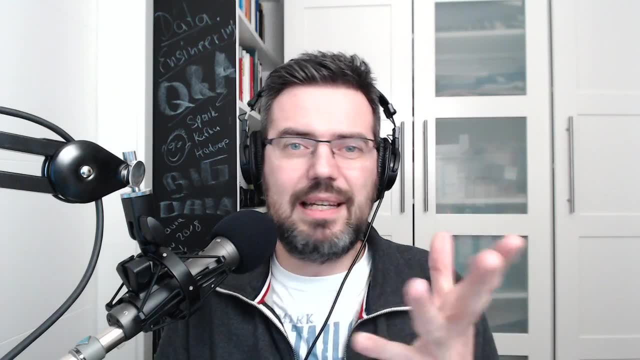 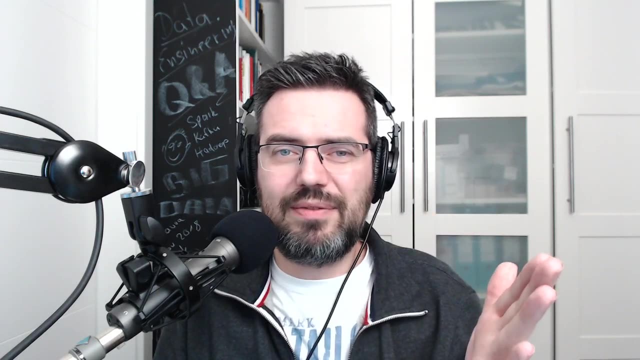 architecture, or if you have a interesting system that you think, man, this would be interesting to analyze and and find out what they are doing and how they are doing it. send it to me, either here or on linkedin or wherever. plumbers of data science- gmailcom. 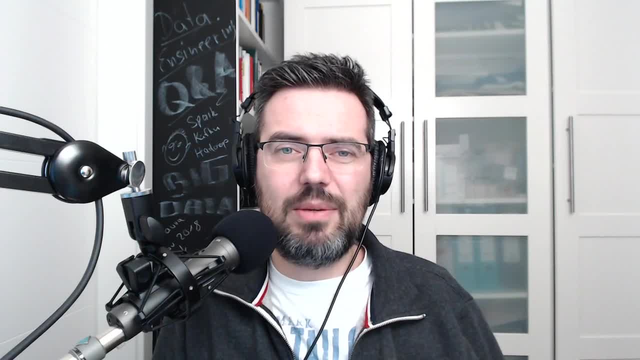 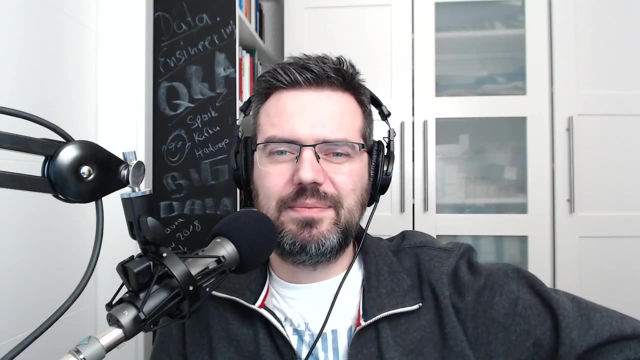 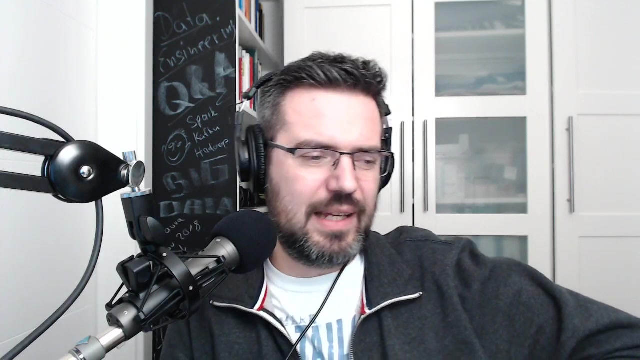 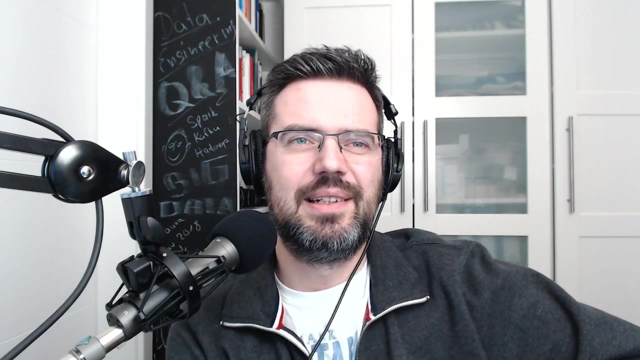 andreas k with two y's at gmailcom. you can find me on twitter or something. um, yeah, let's, let's, let's review this. this is this might also be be a lot of fun. um, yeah, all right then. yeah, let's get back tomorrow and have a have a great day, or a great evening, depending on where you are.